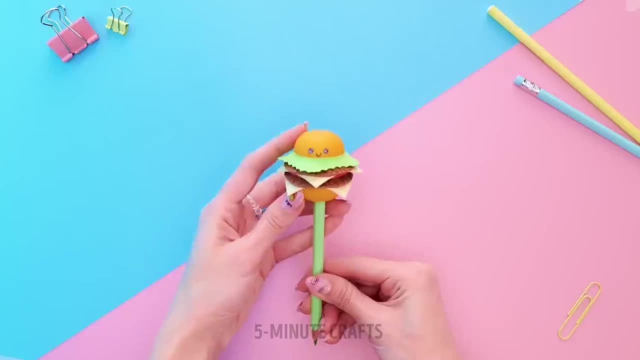 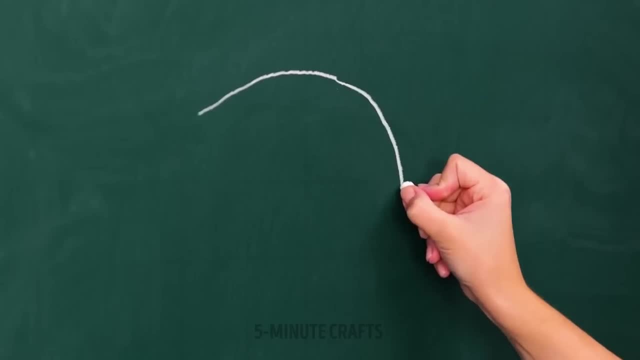 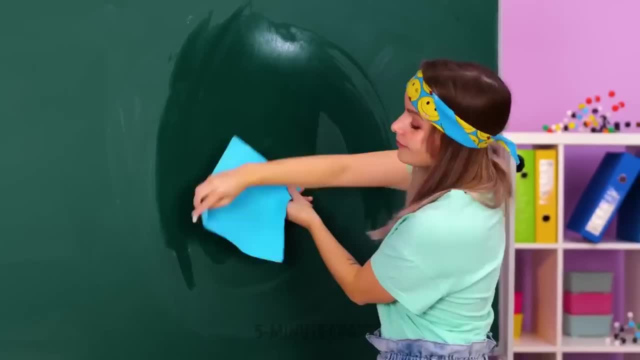 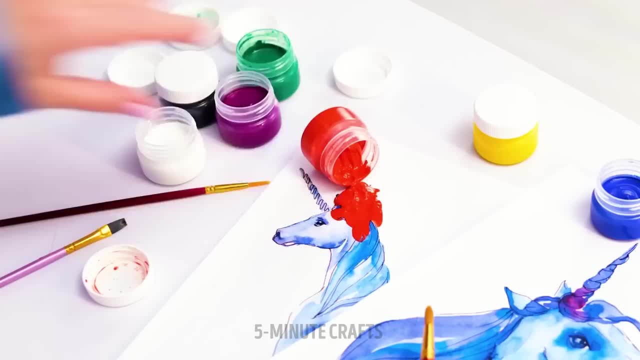 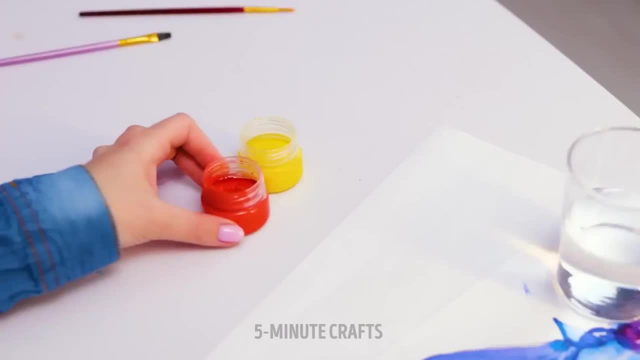 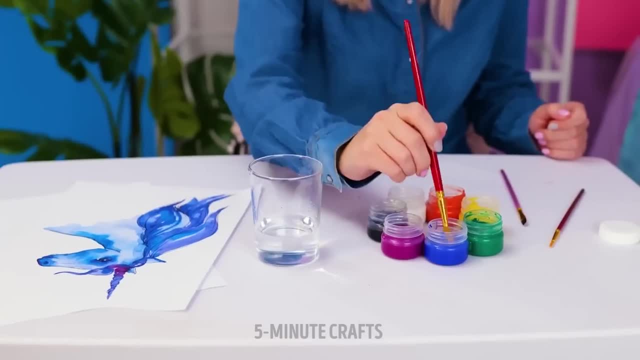 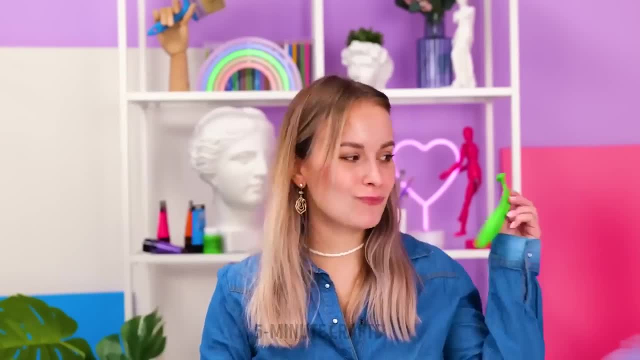 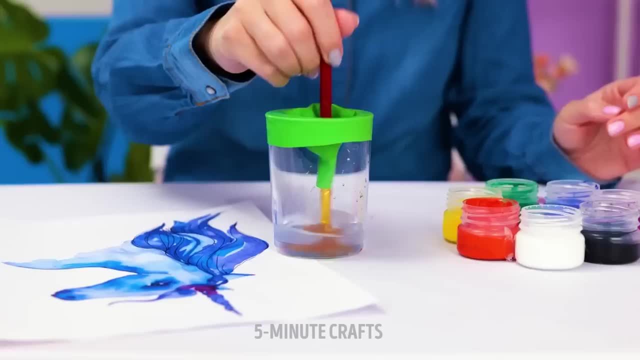 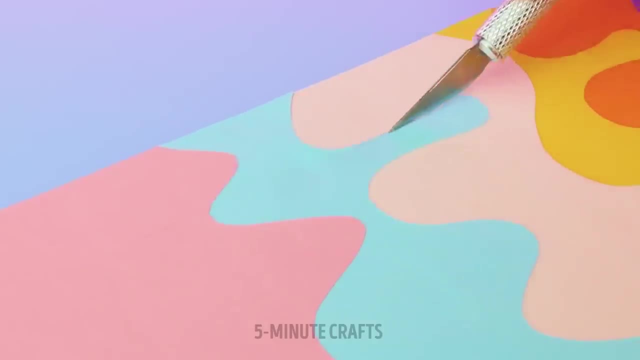 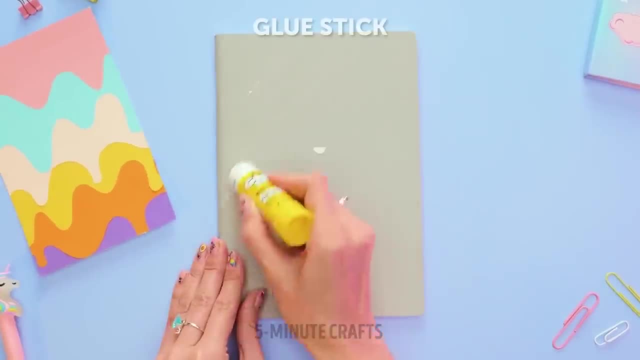 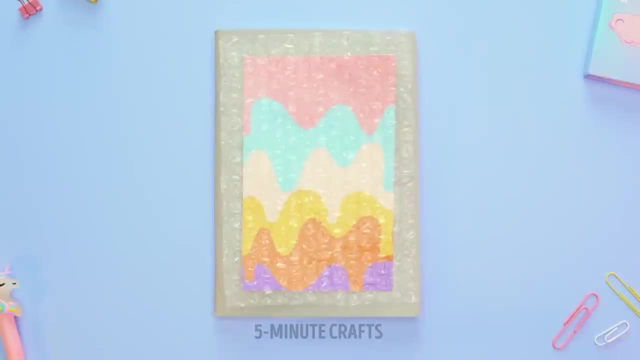 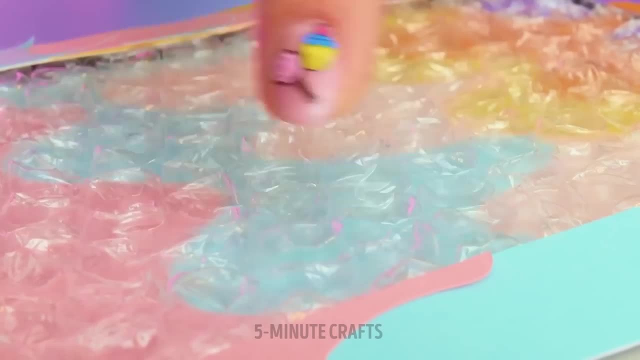 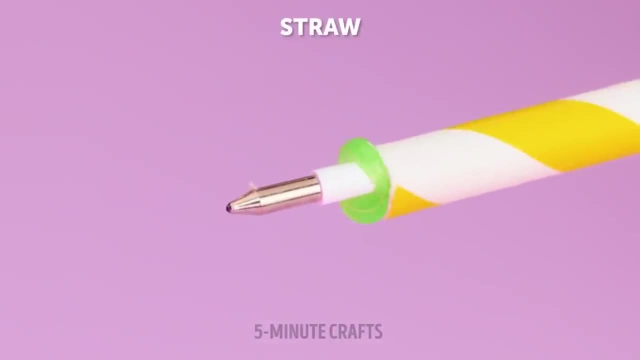 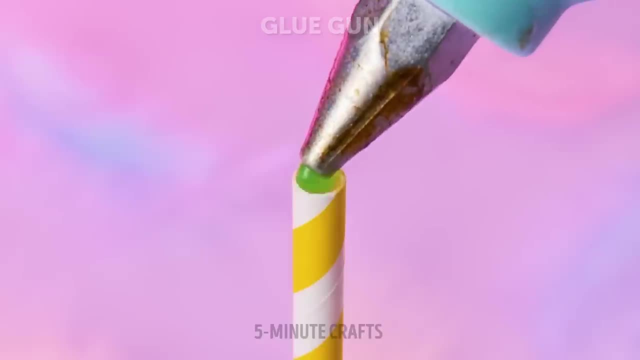 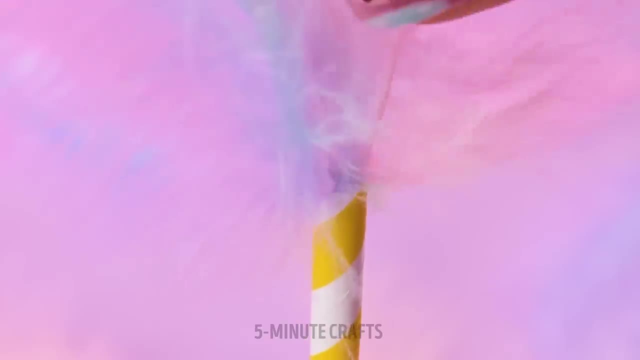 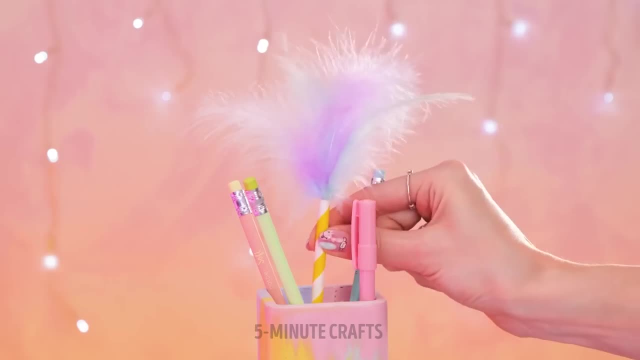 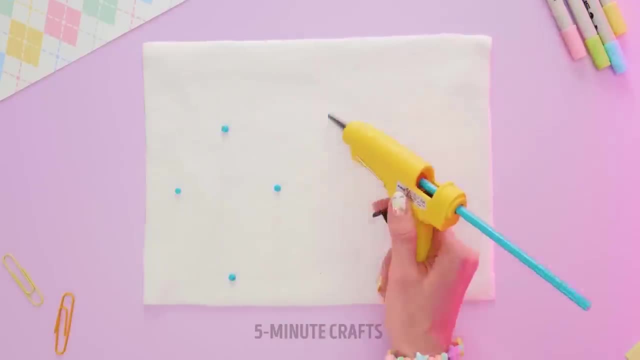 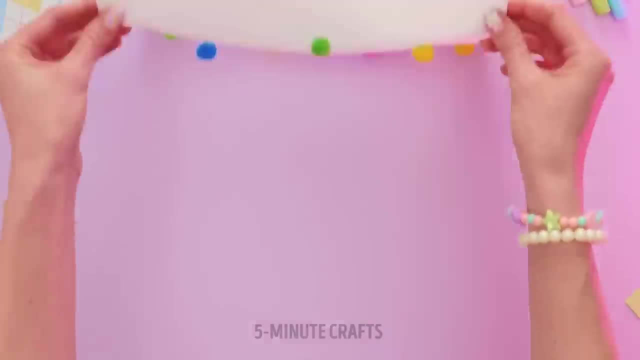 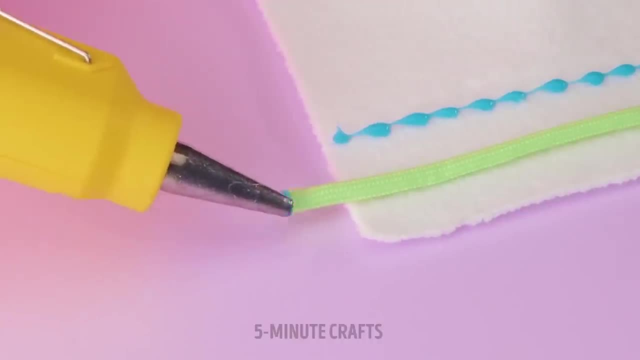 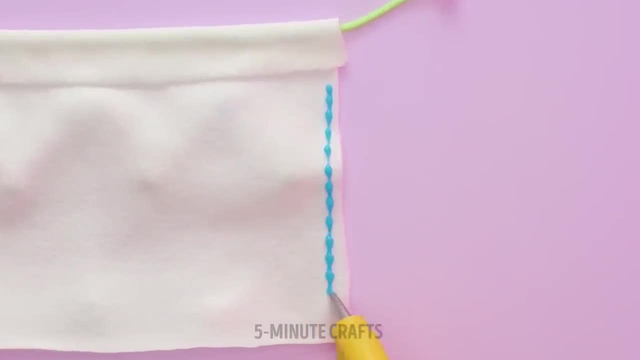 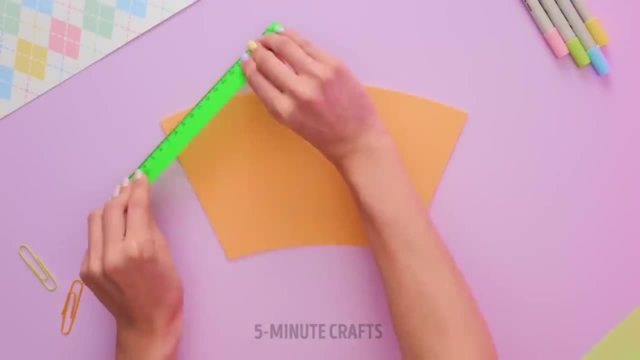 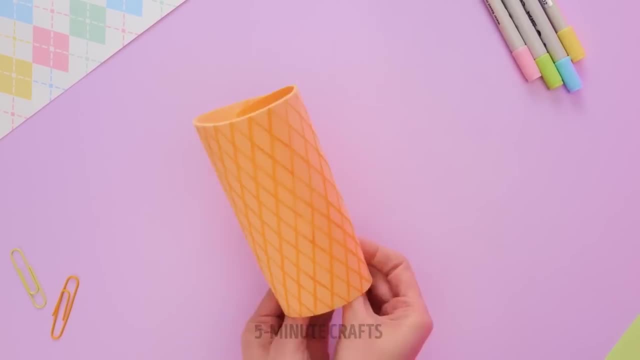 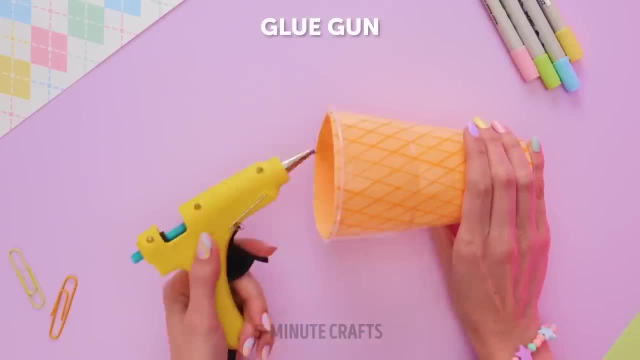 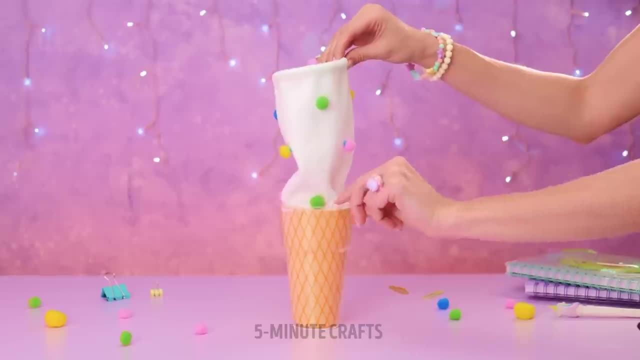 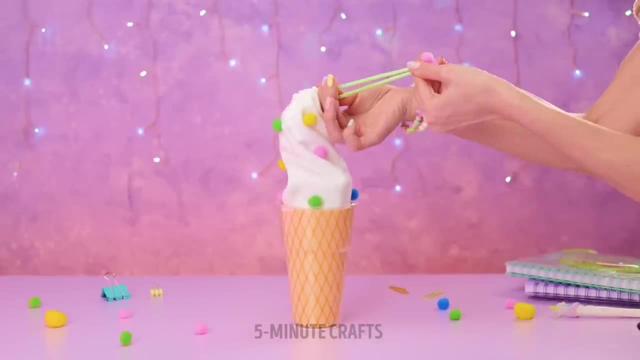 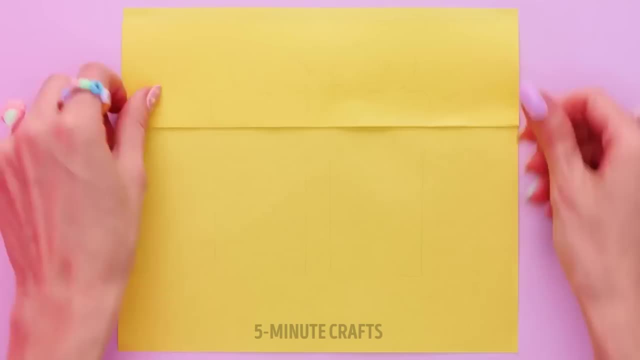 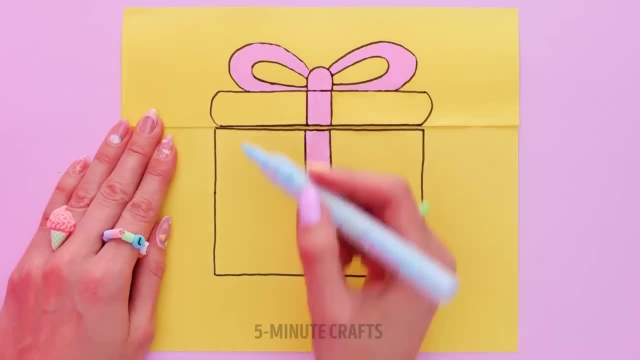 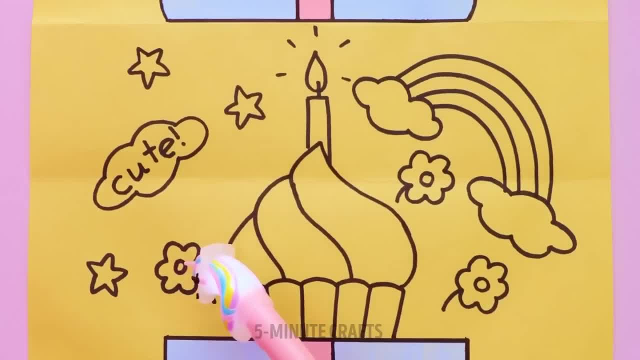 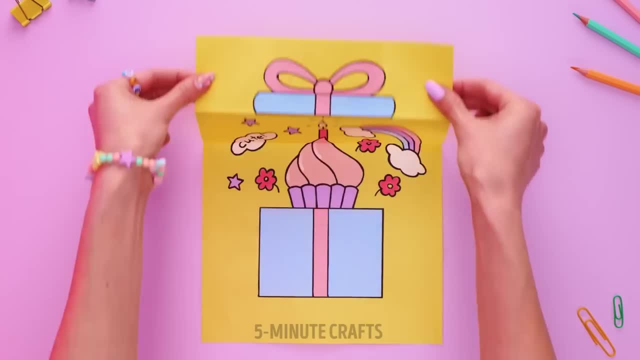 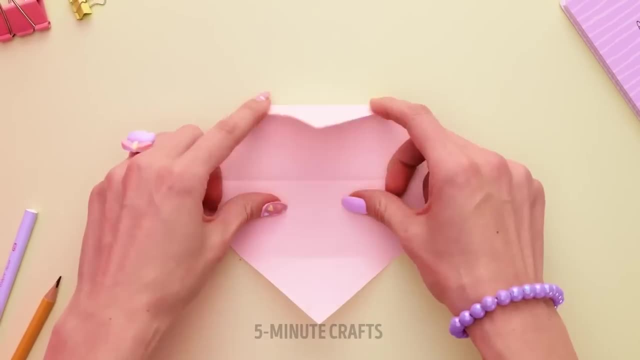 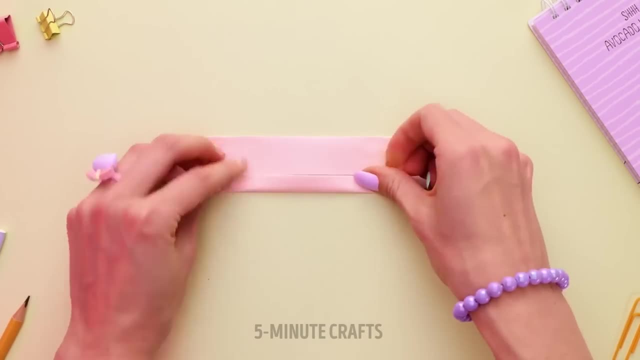 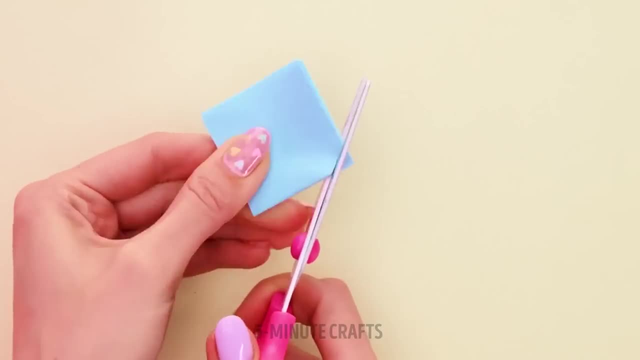 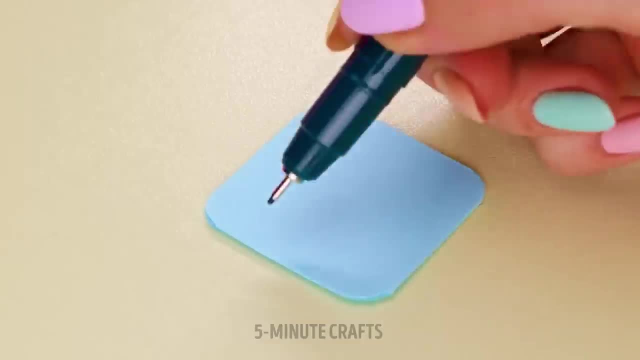 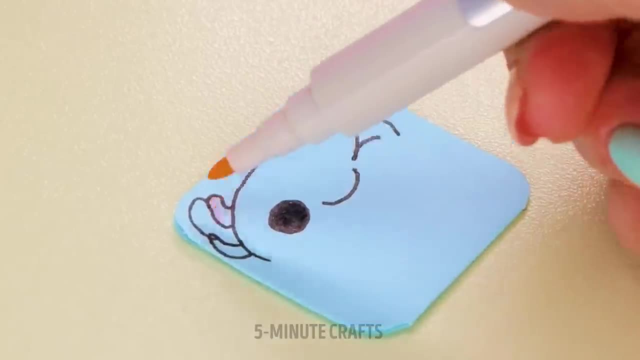 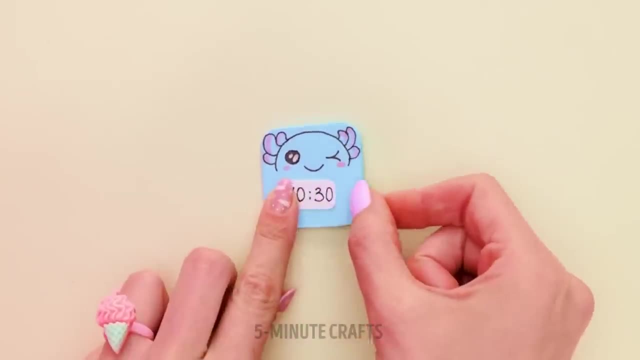 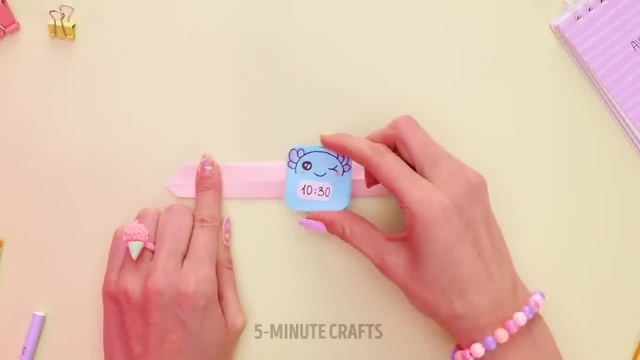 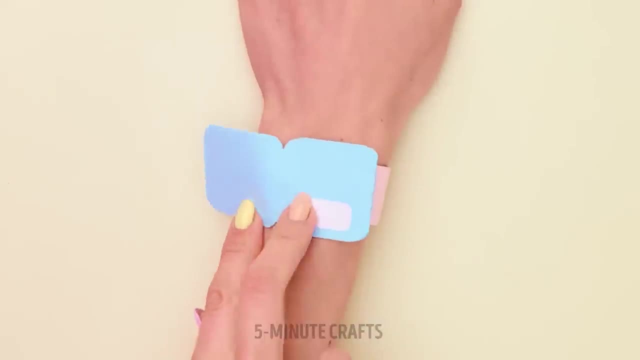 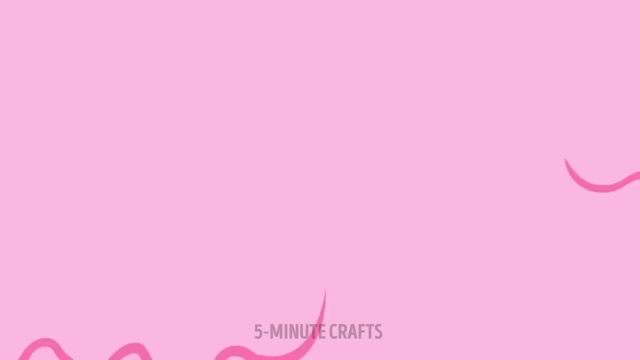 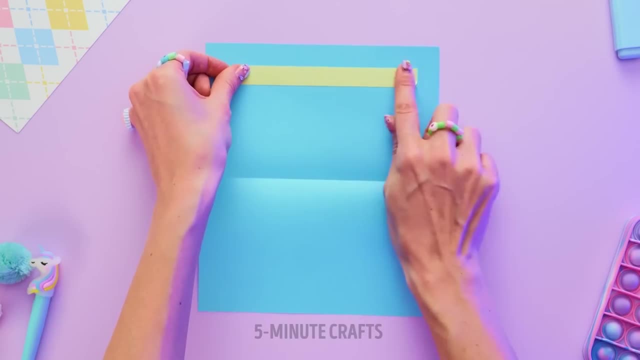 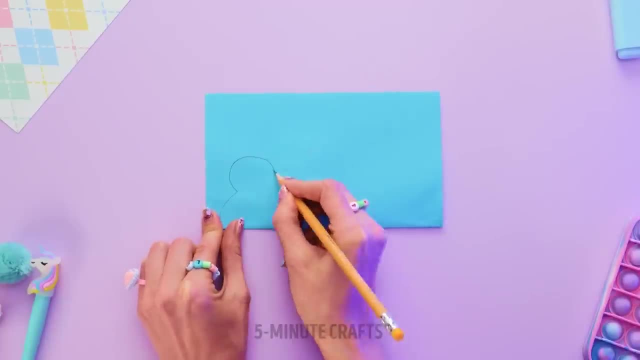 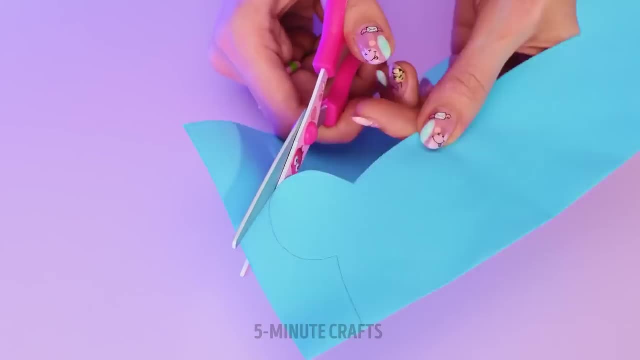 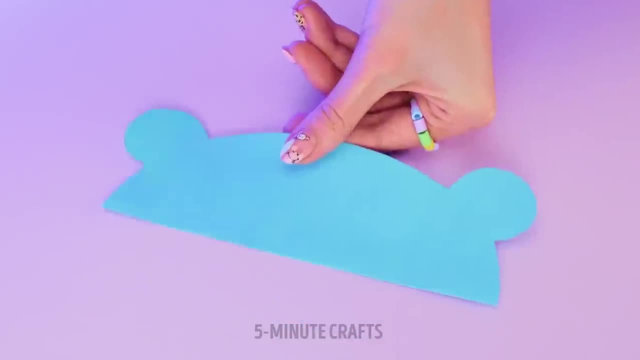 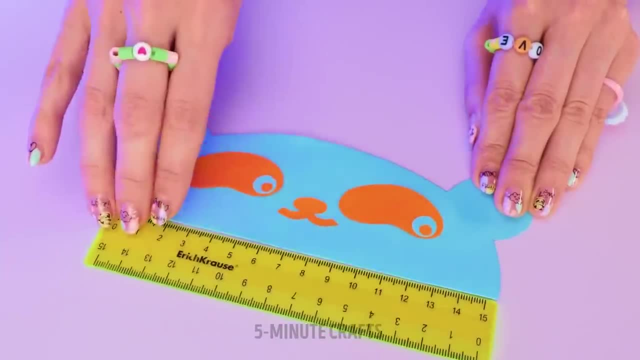 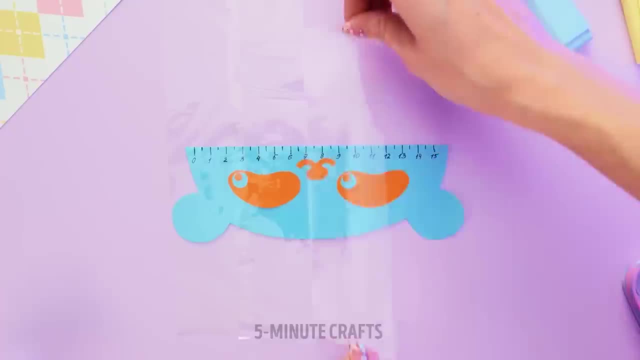 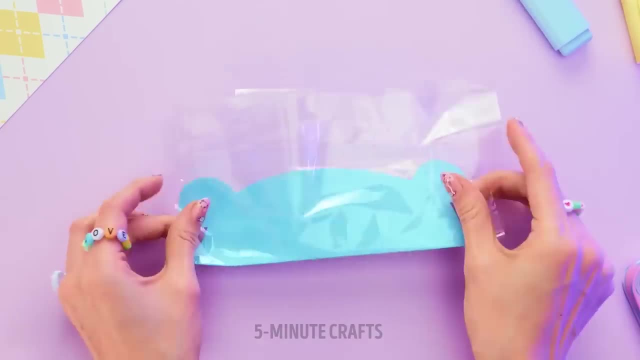 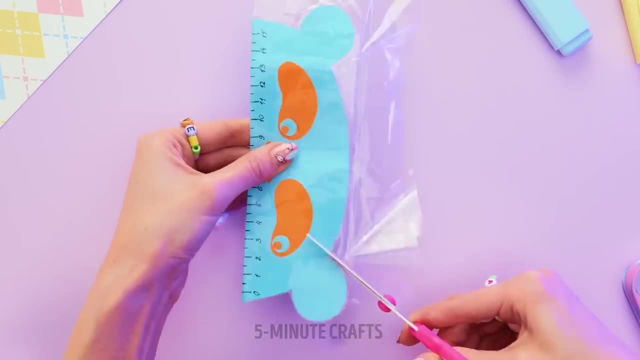 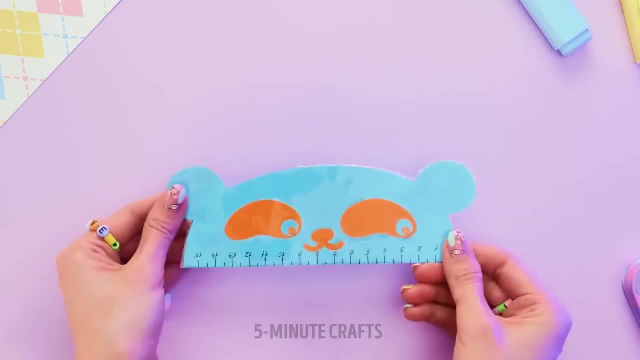 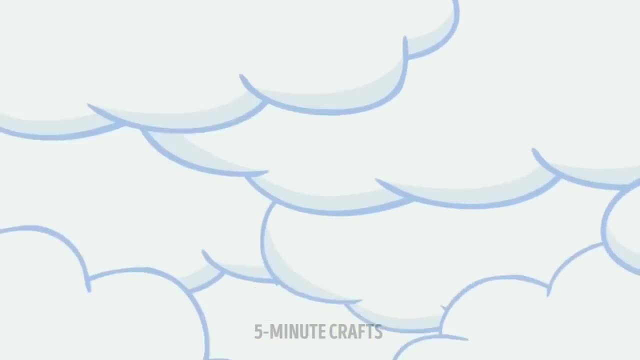 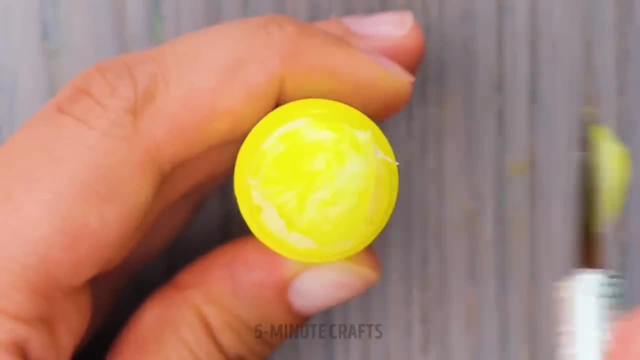 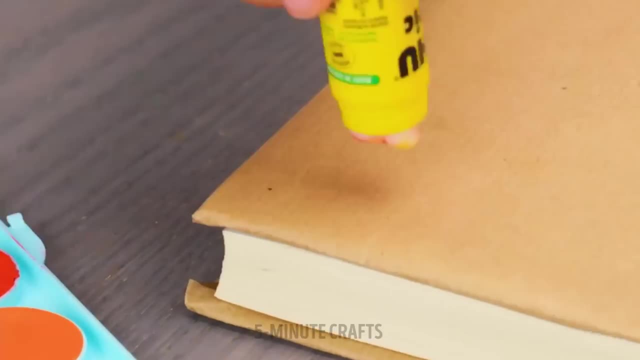 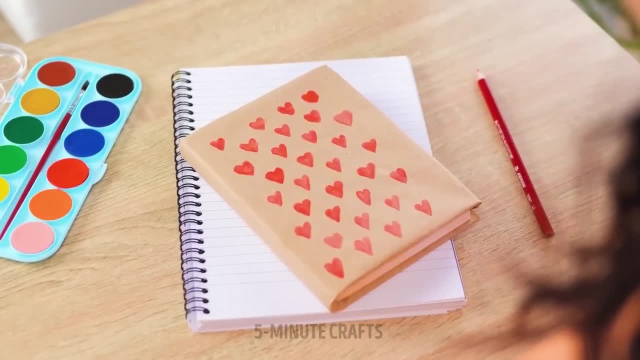 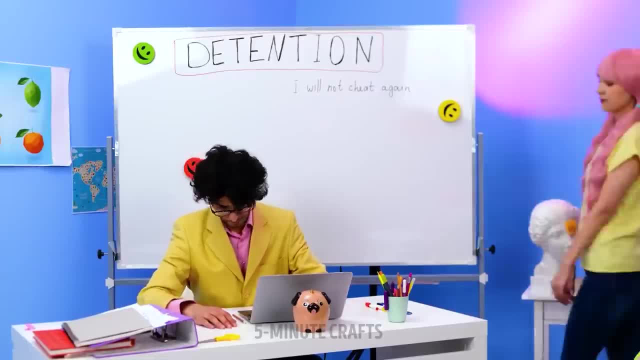 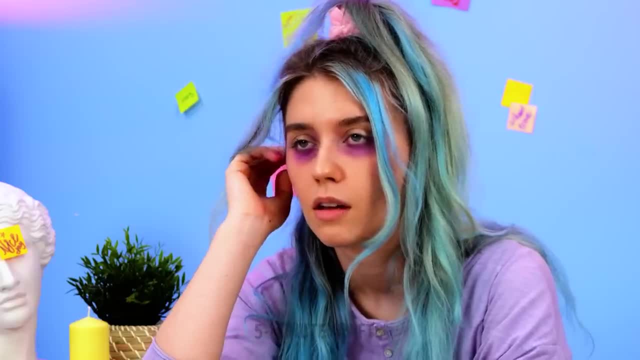 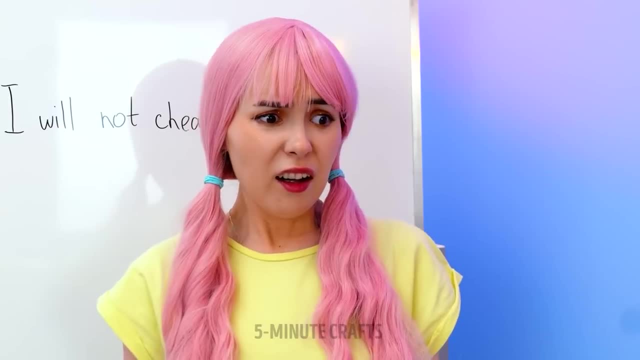 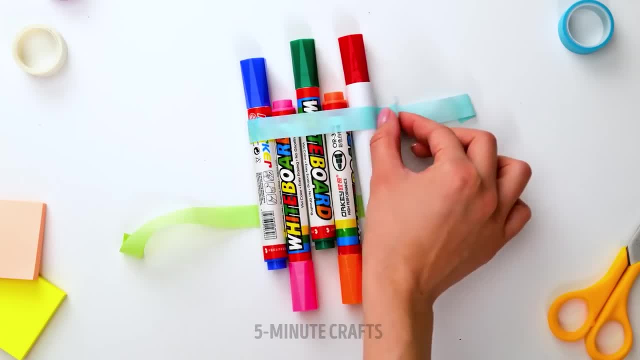 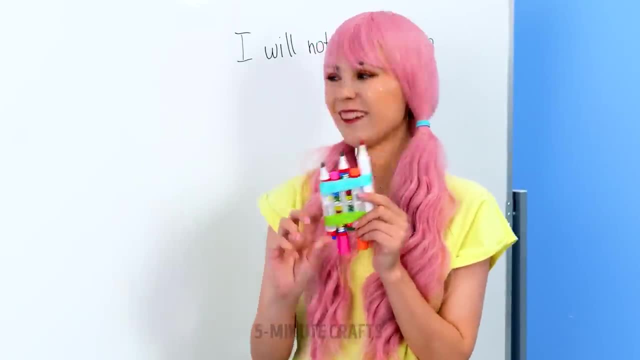 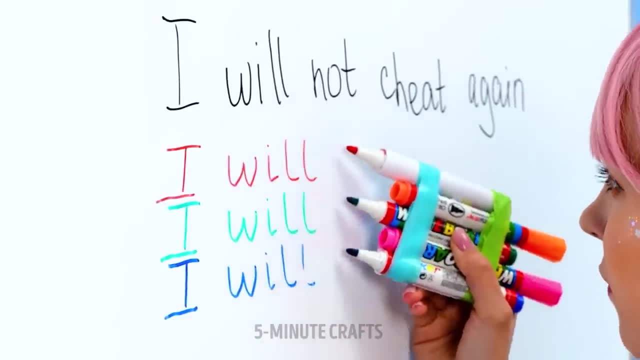 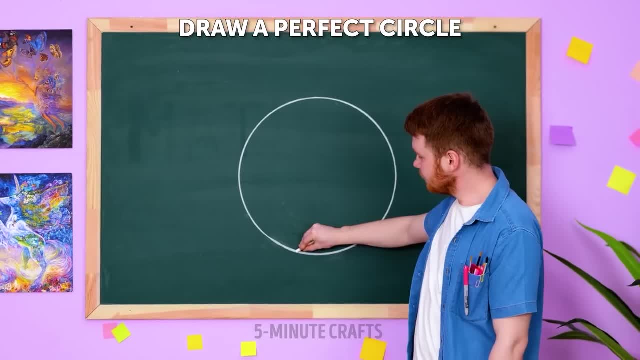 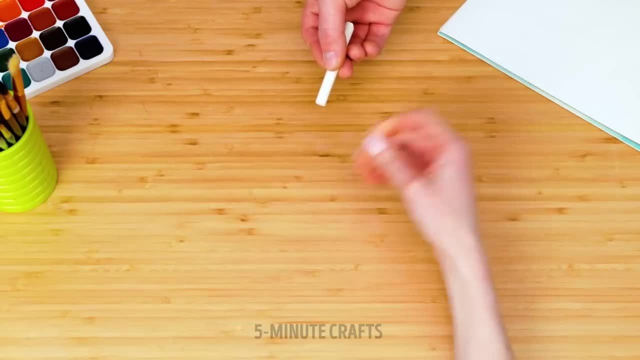 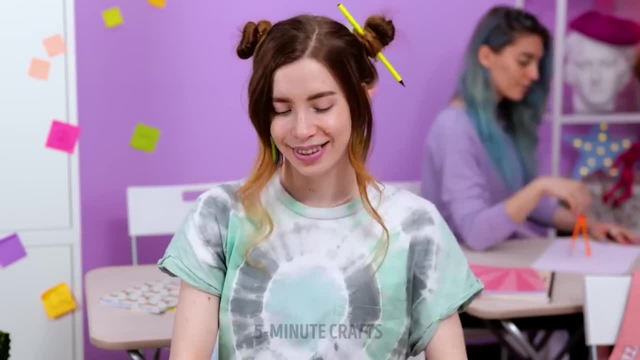 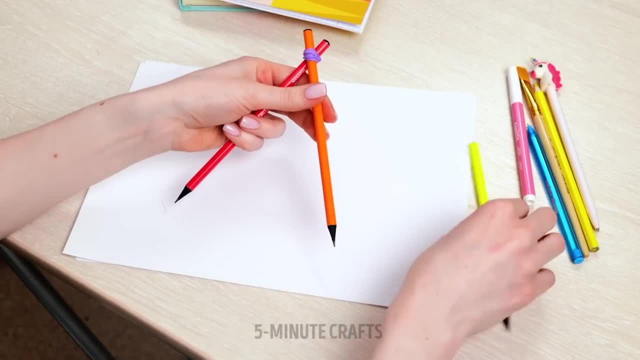 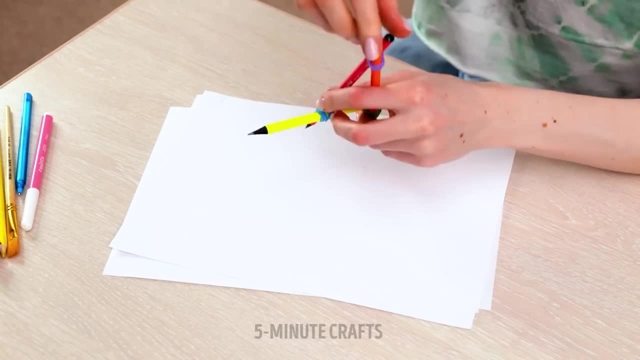 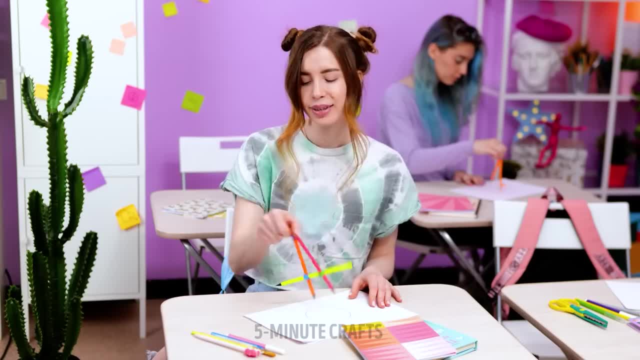 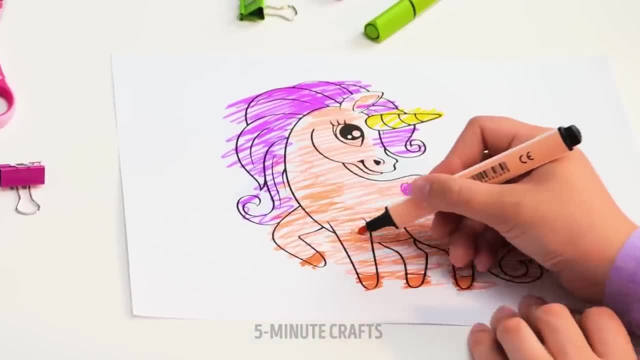 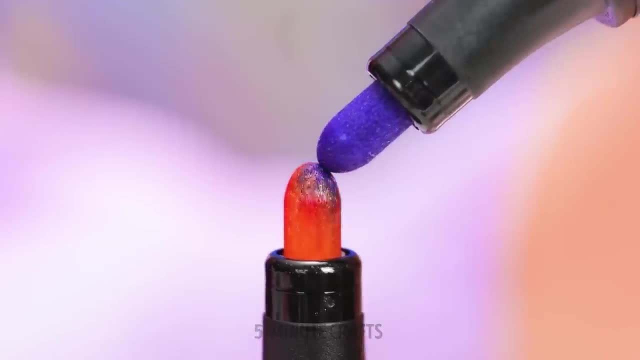 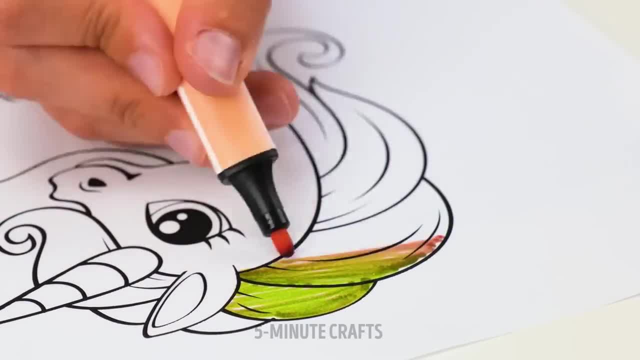 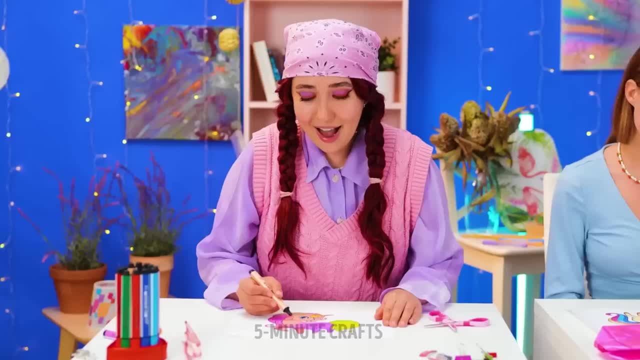 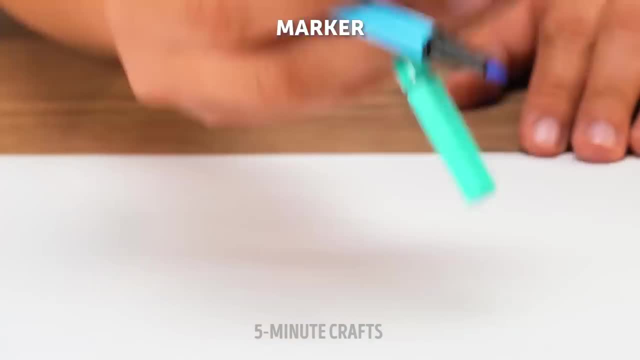 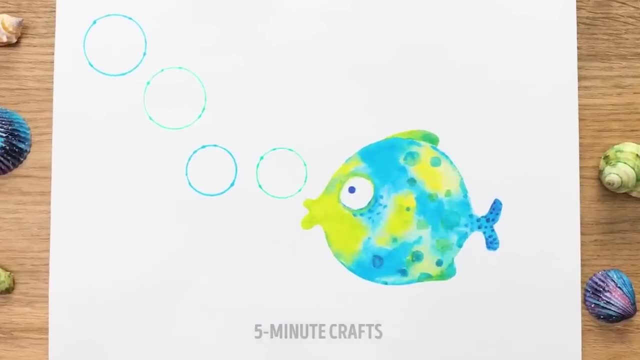 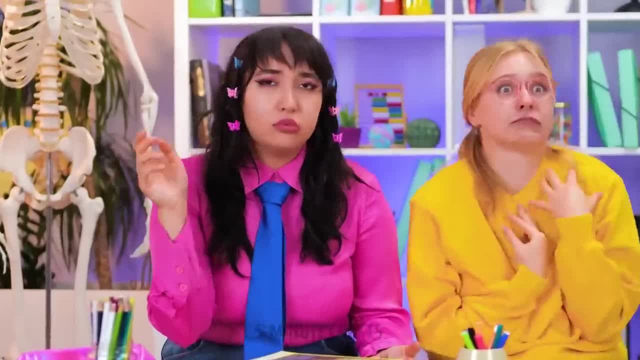 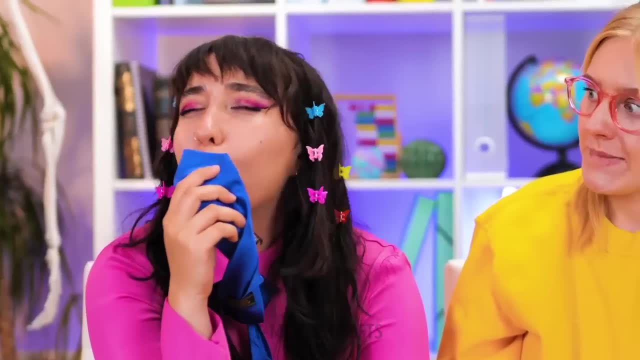 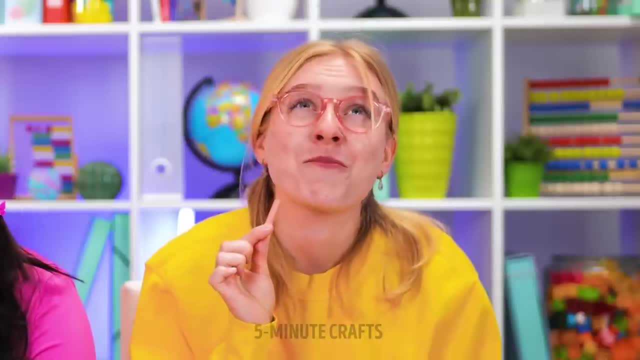 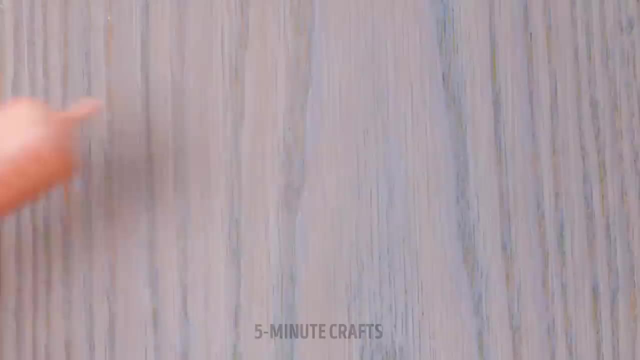 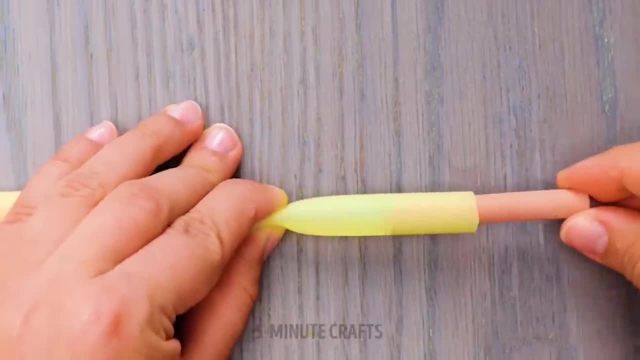 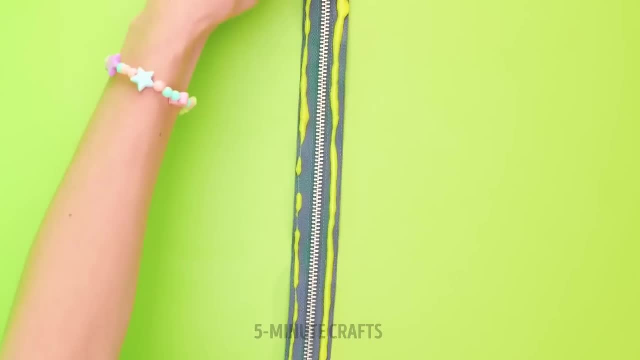 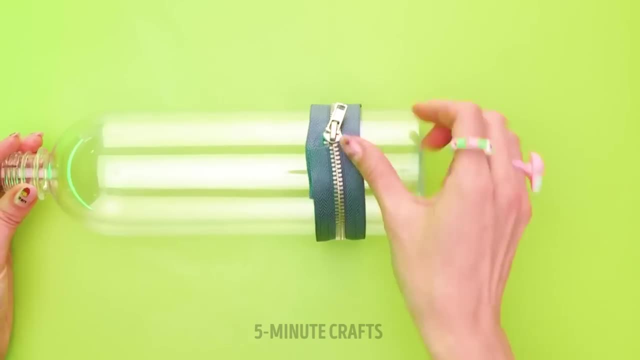 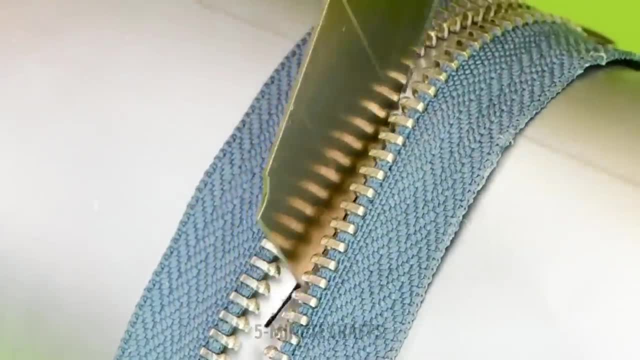 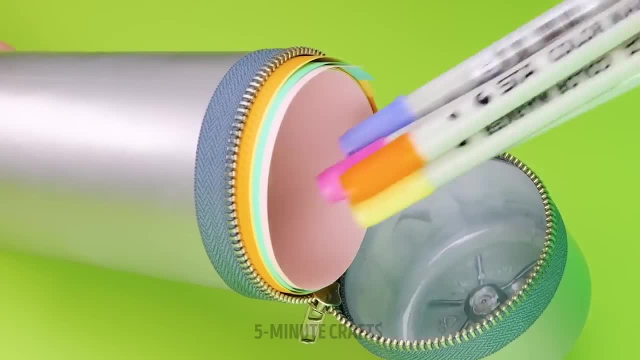 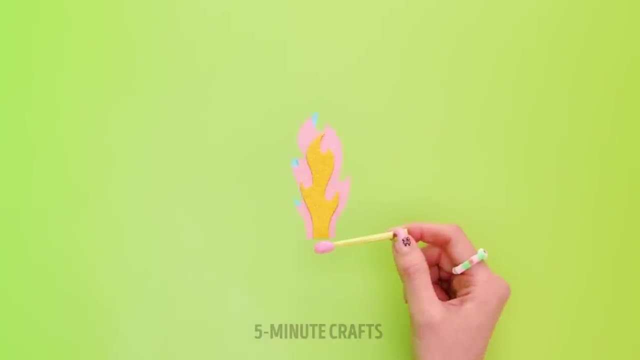 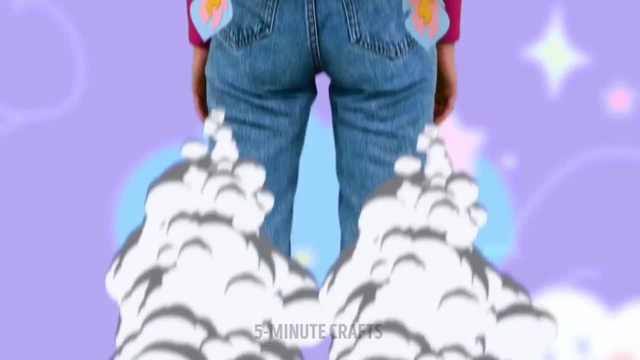 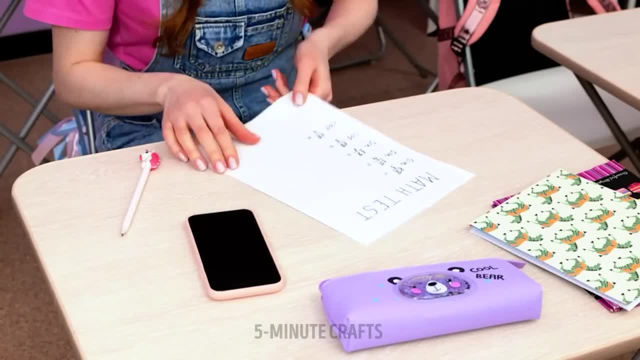 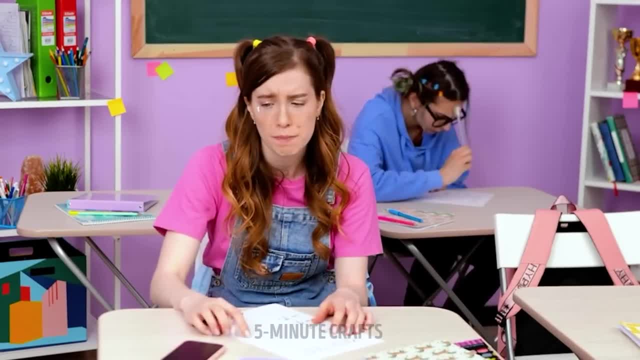 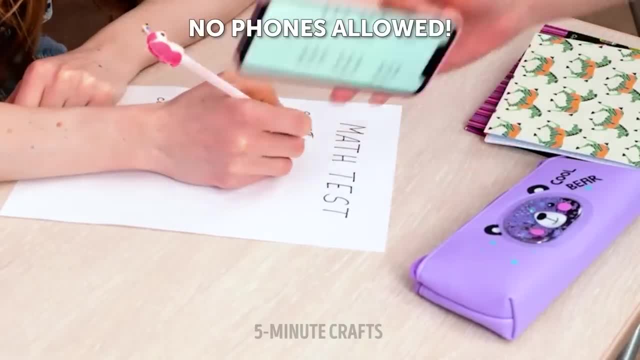 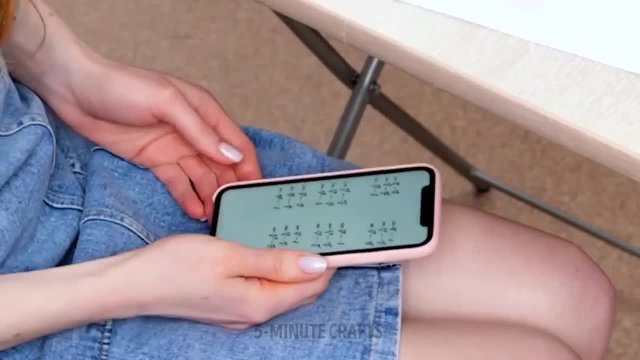 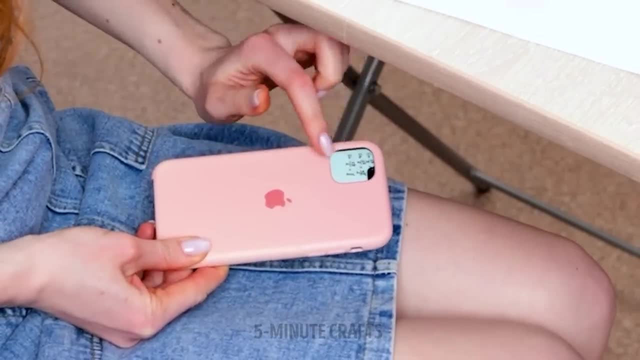 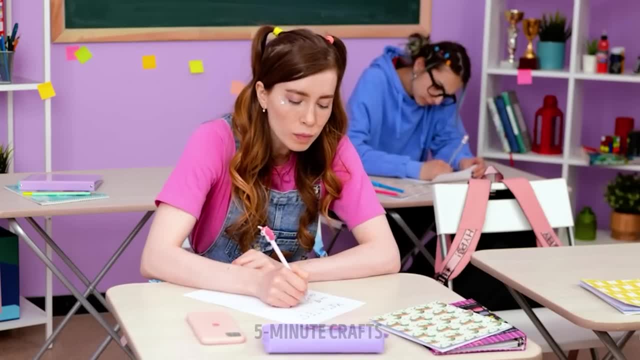 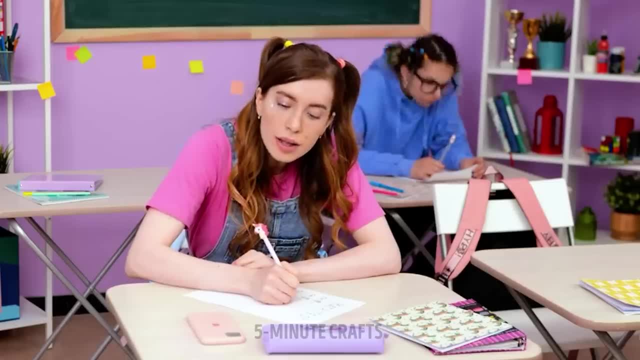 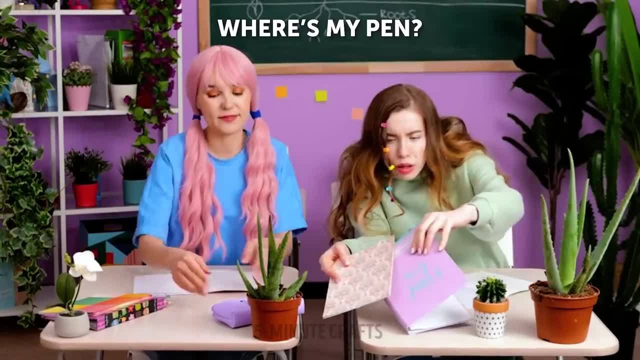 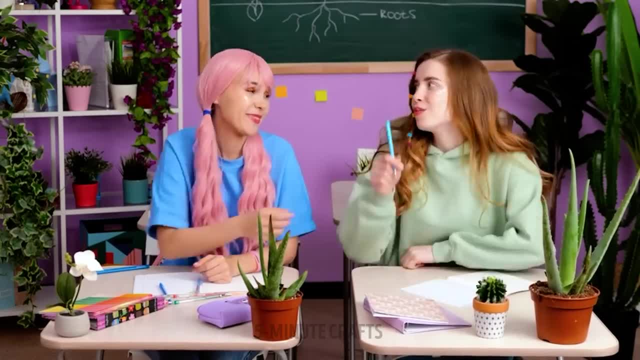 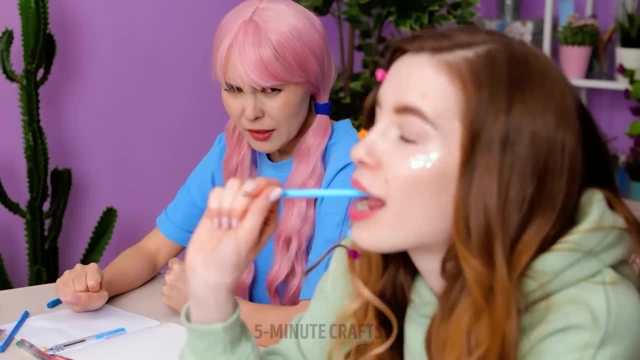 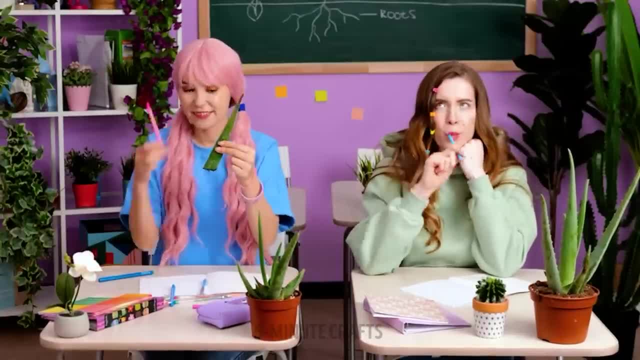 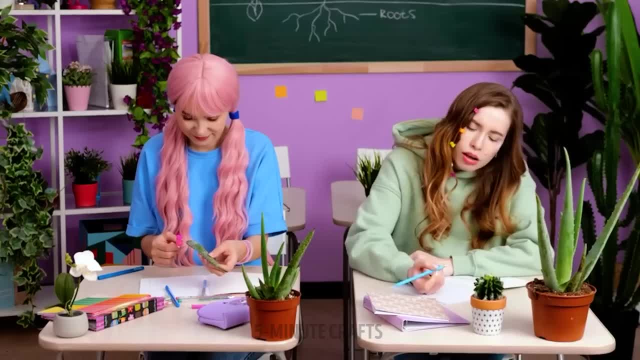 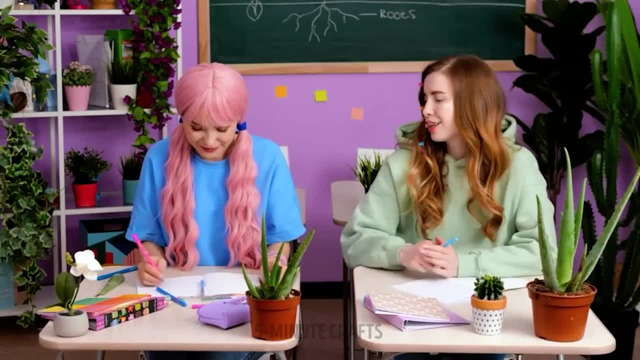 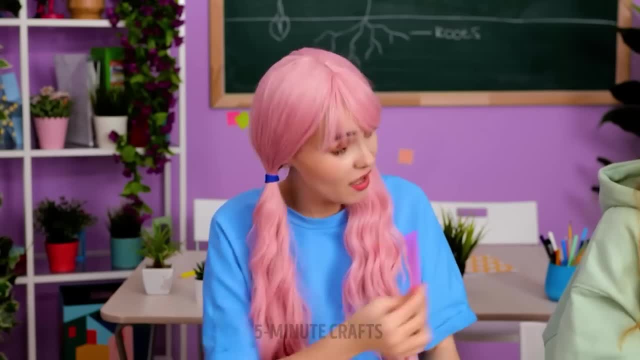 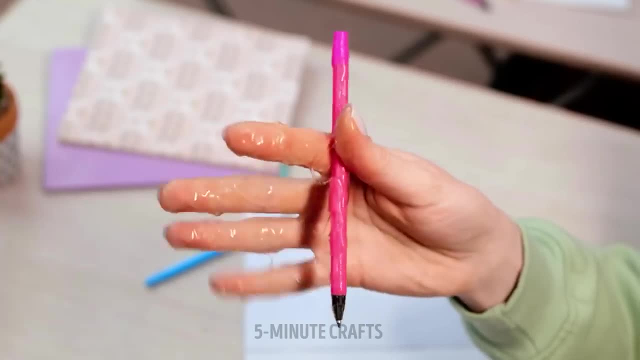 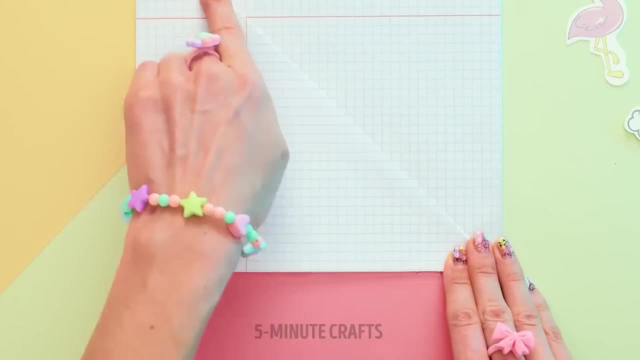 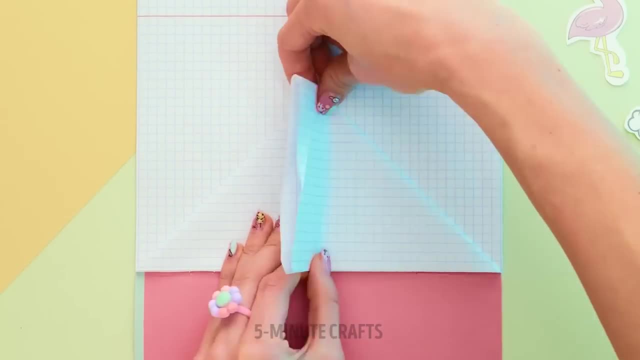 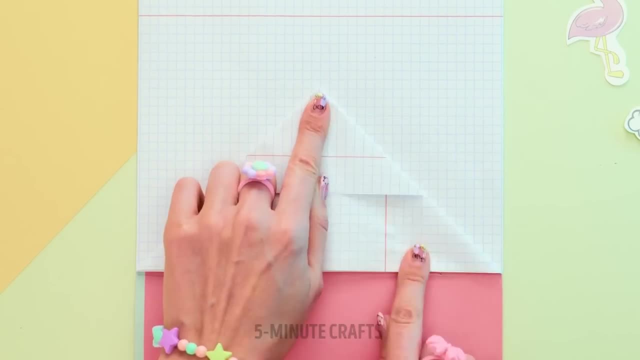 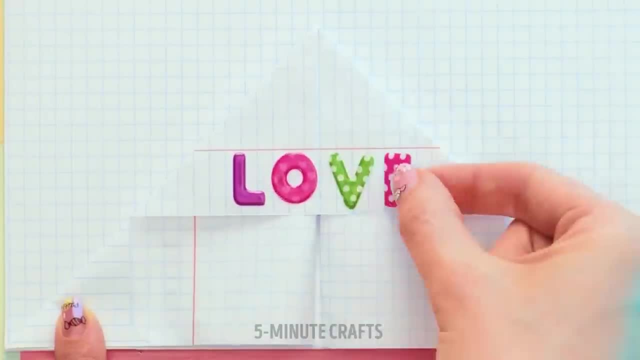 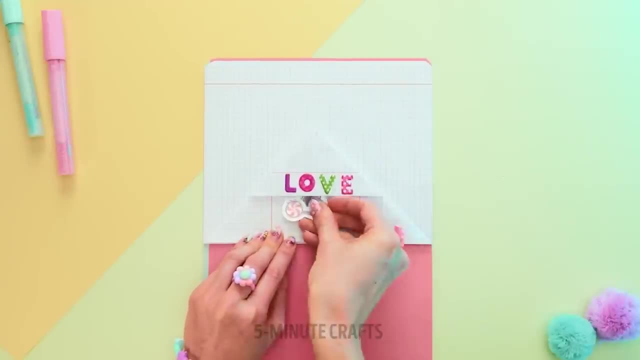 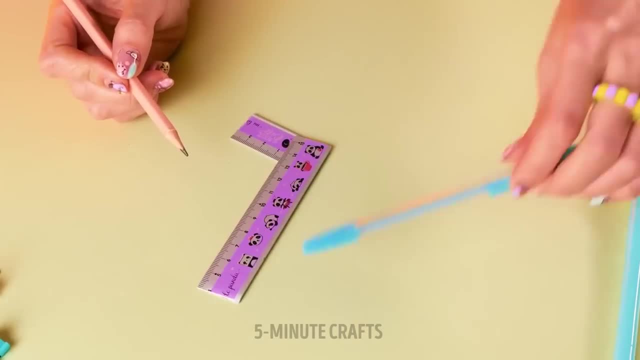 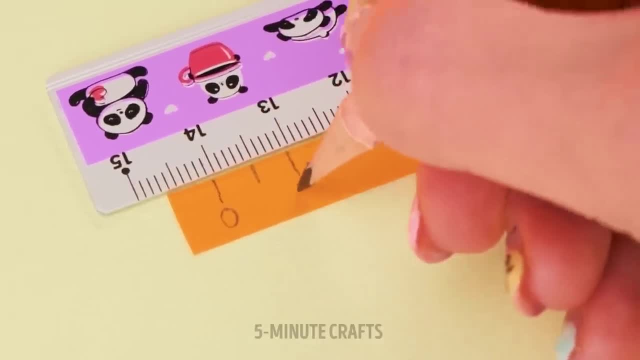 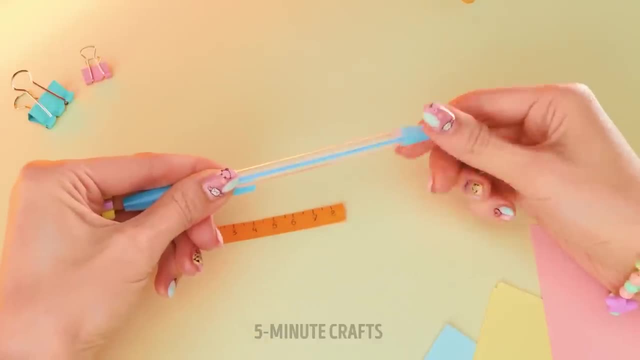 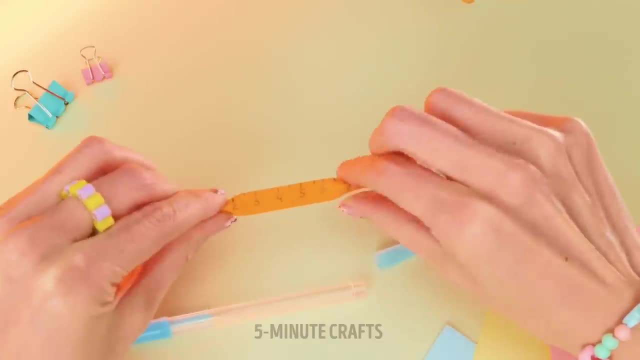 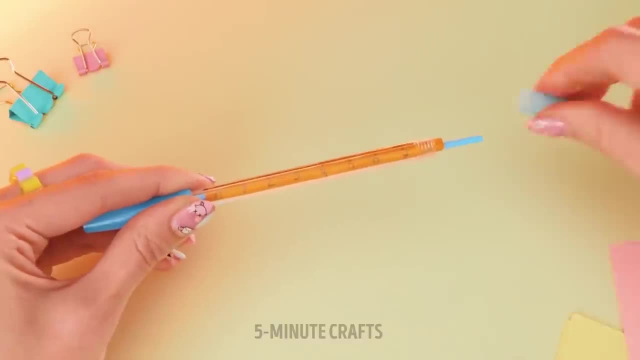 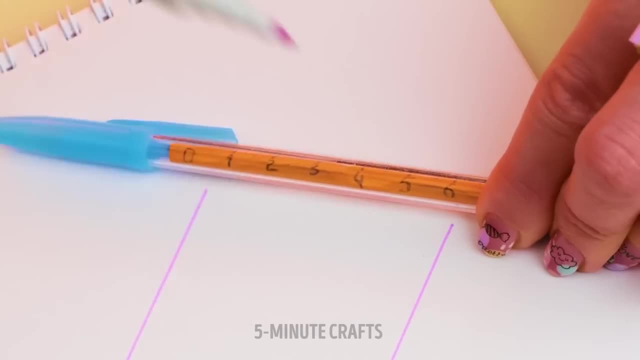 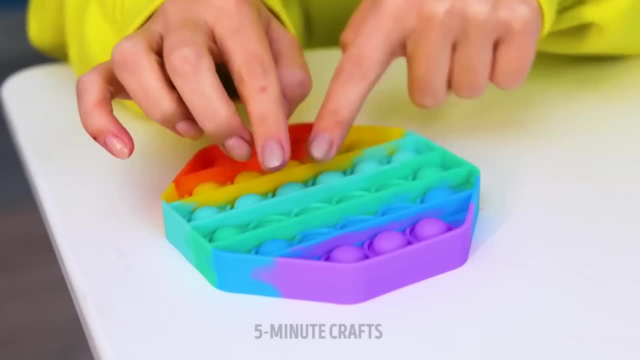 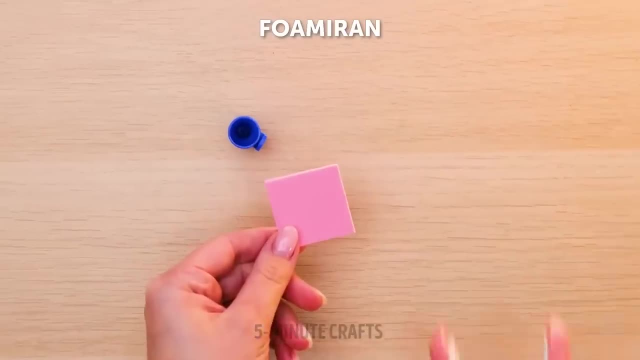 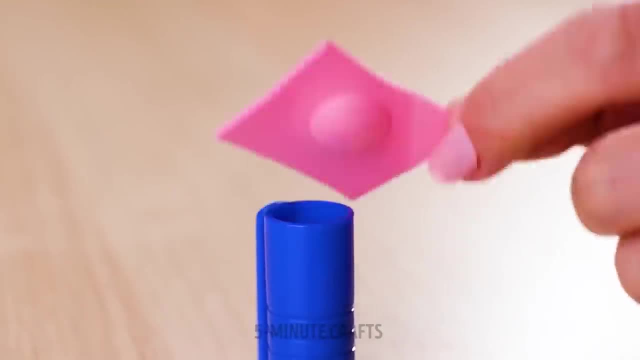 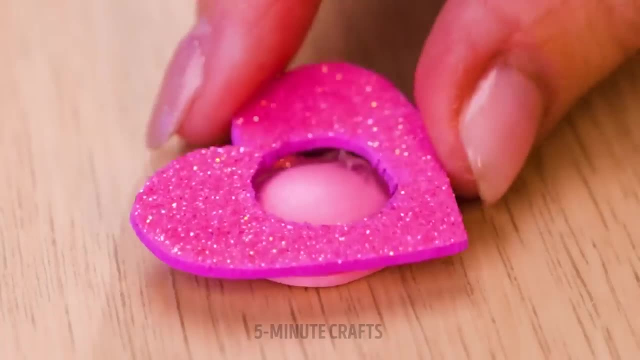 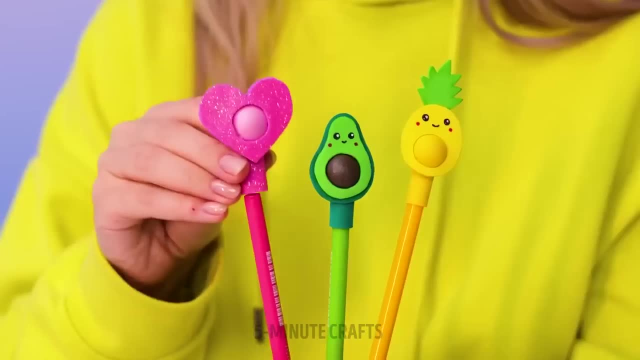 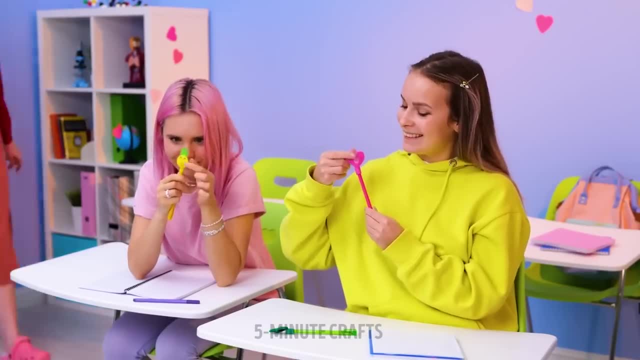 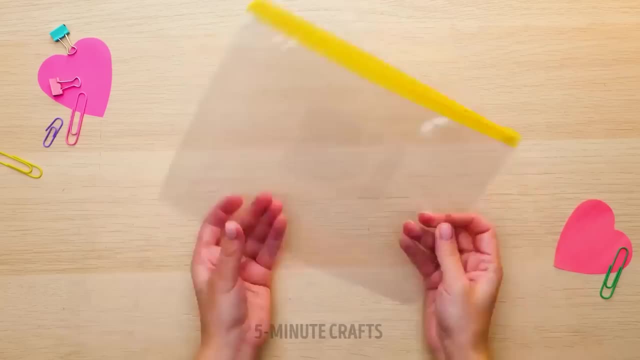 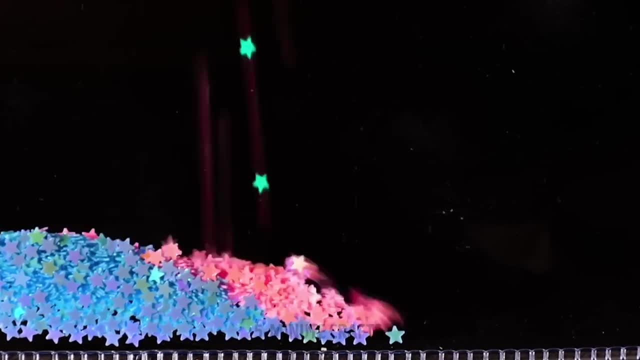 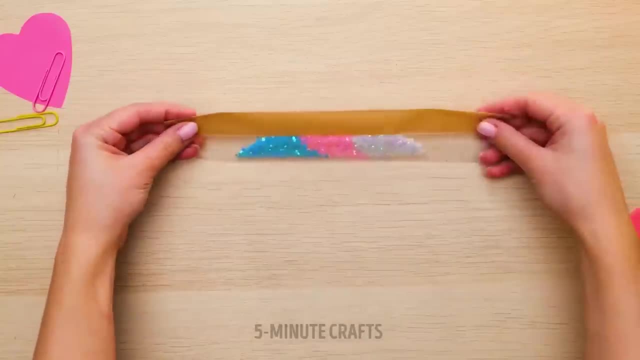 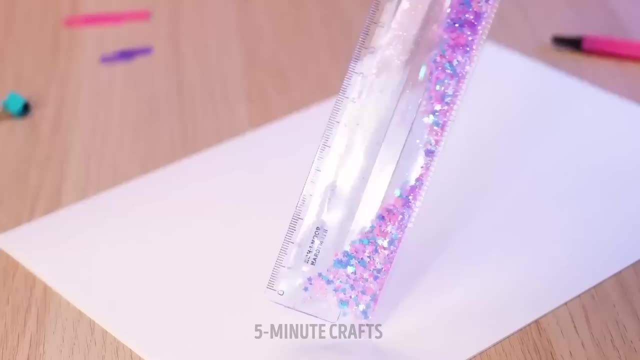 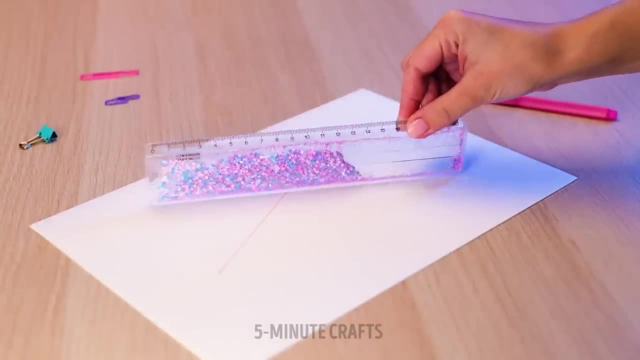 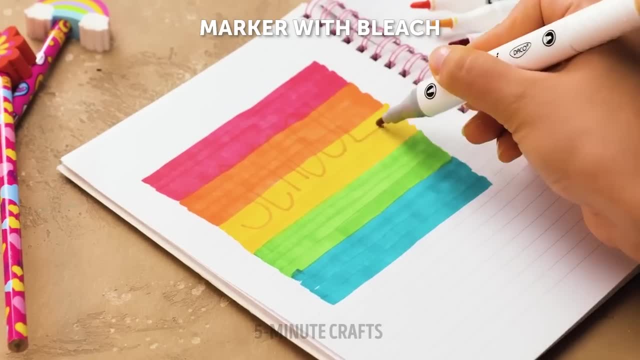 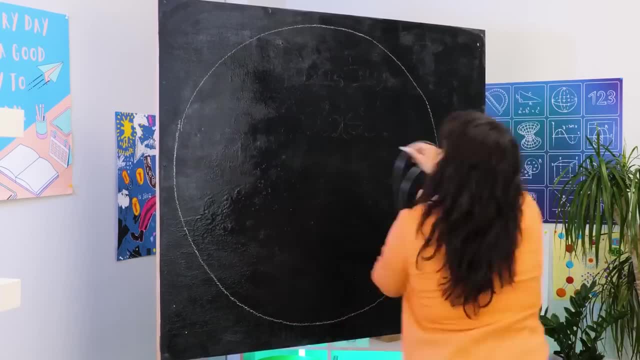 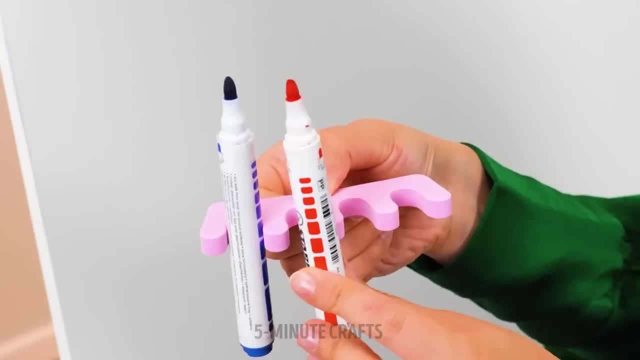 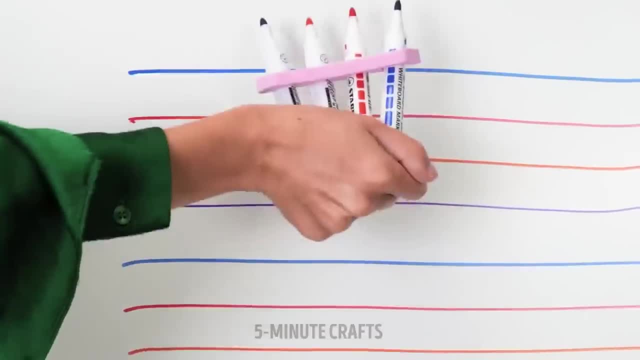 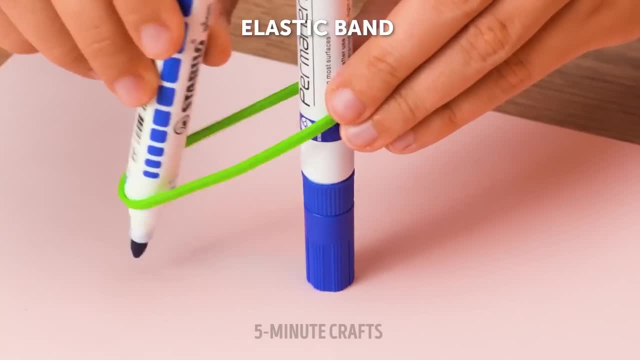 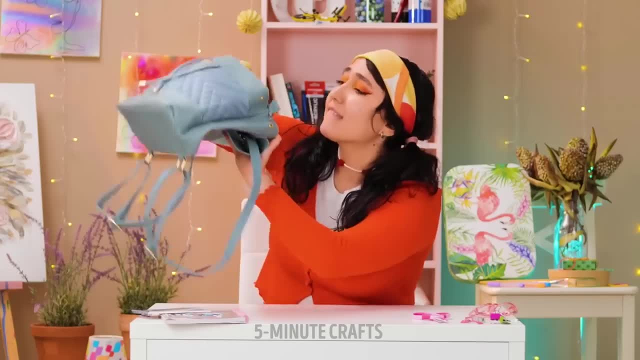 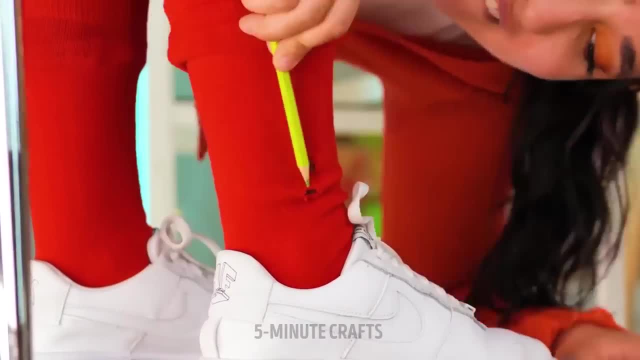 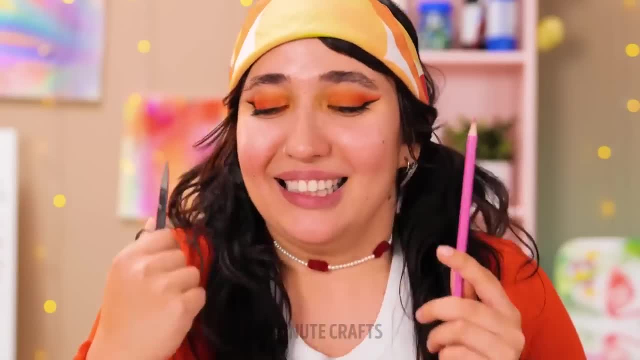 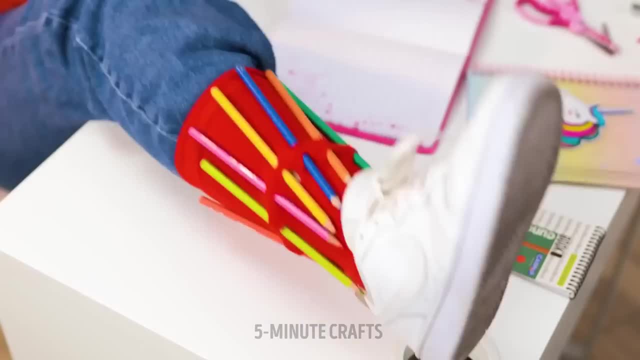 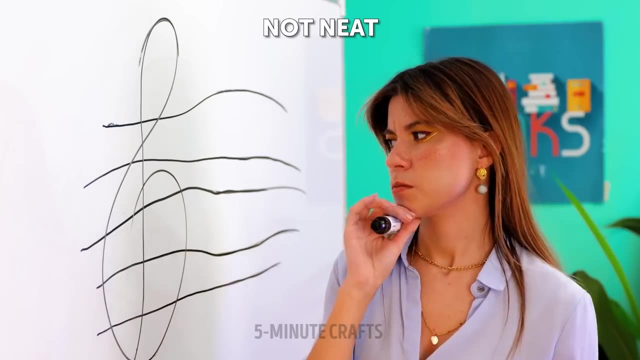 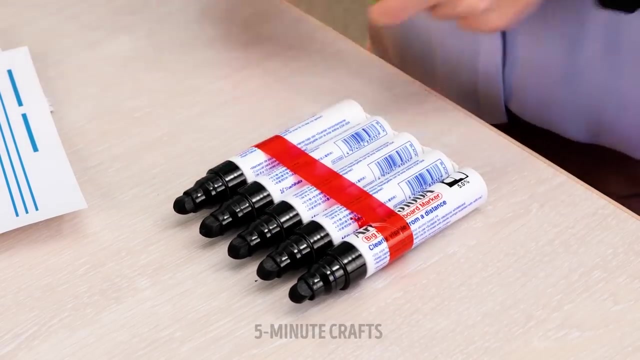 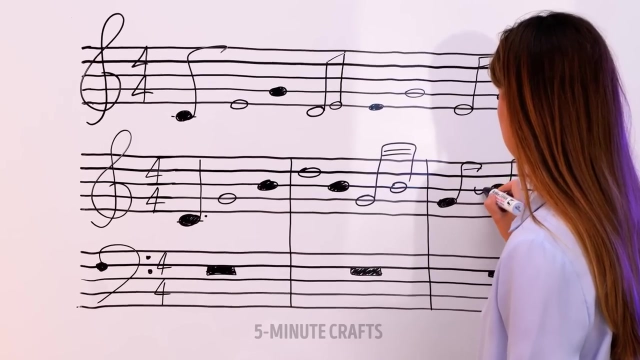 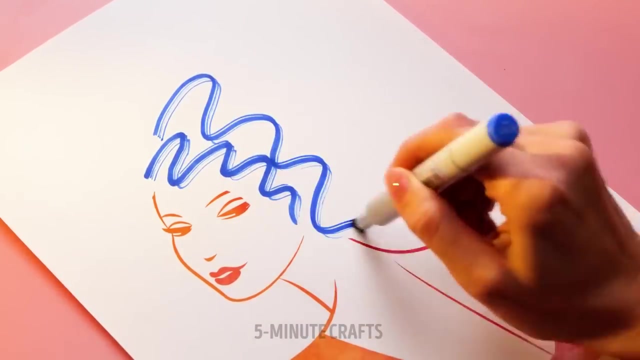 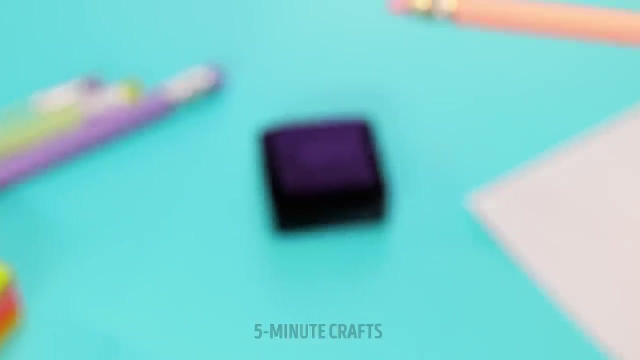 This video is a work of fiction. Any resemblance to actual persons, living or dead, is coincidental. Talk to me, baby. I've been waiting for you for a lifetime. just keep on fading in all these photos, calling the memories and capturing the. highlights: just keep on waiting. glass after glass, i keep hoping you'll come around, drowning. i'm fighting what whatever can be found, cause i've given in to all my demons lately, you know, might be easier just to let it go, cause the cable's short and the problems all. 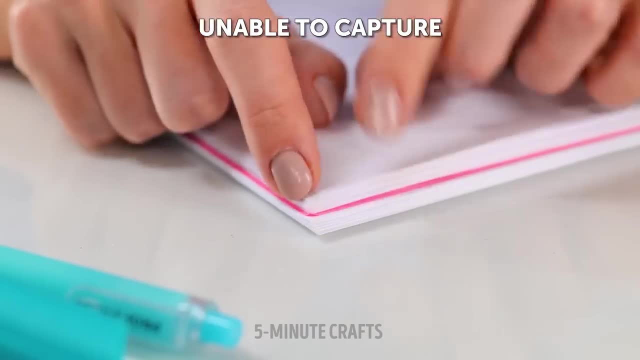 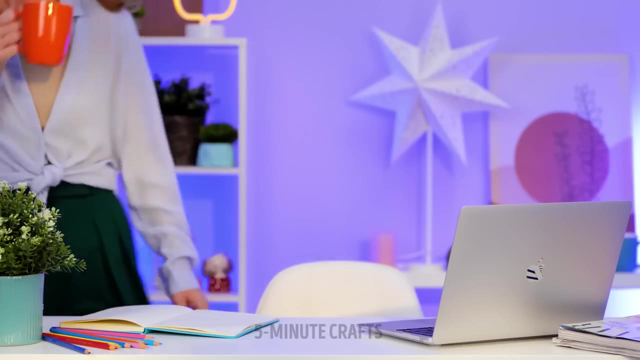 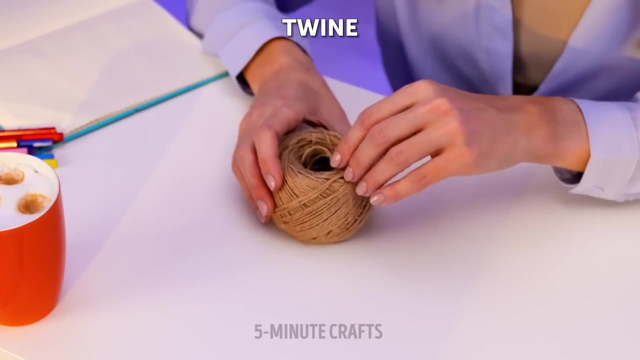 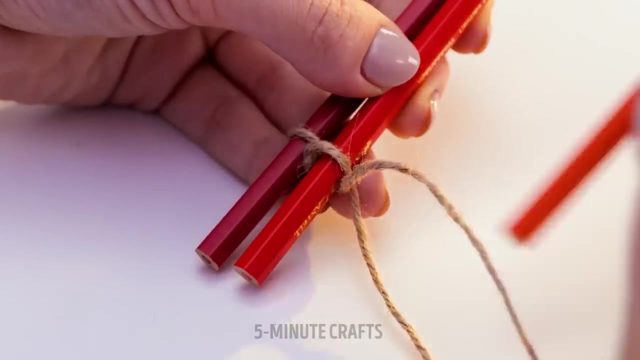 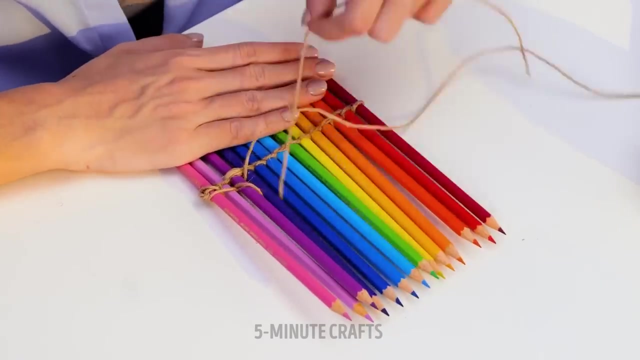 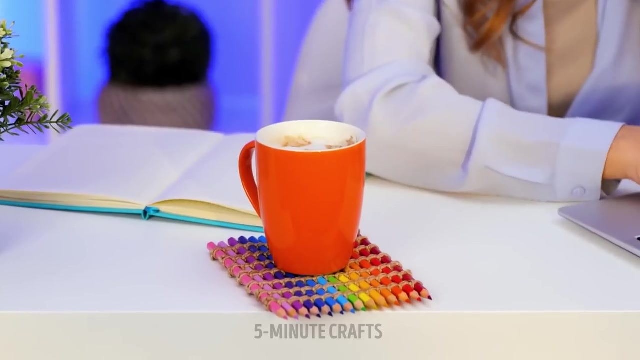 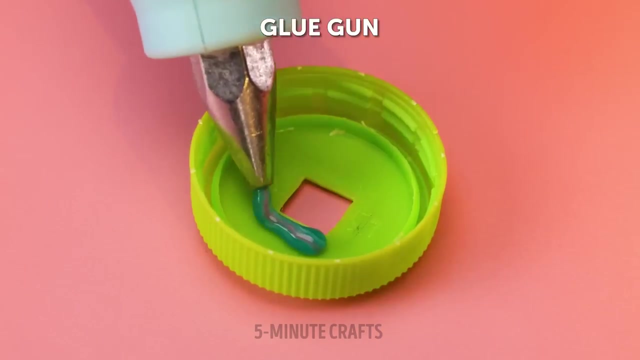 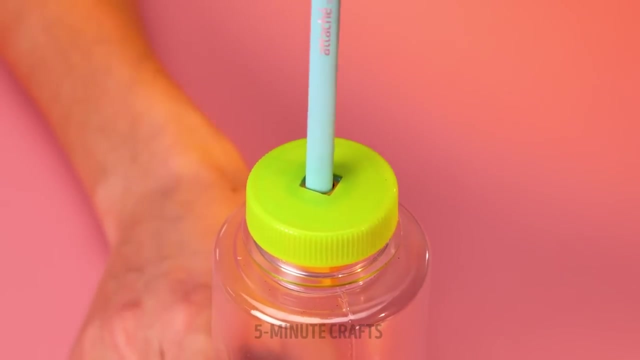 might be easier for you. i do it all night staying for me darling. it's been quiet for a day now. can't bear the silence, you know. might be easier just to let it go inside my own head. i keep on hoping somehow we can make this all right. just keep on trying. 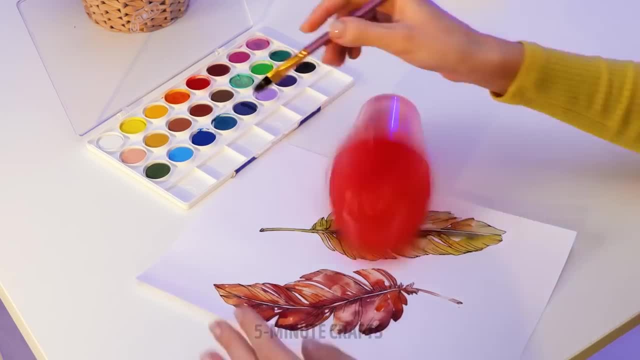 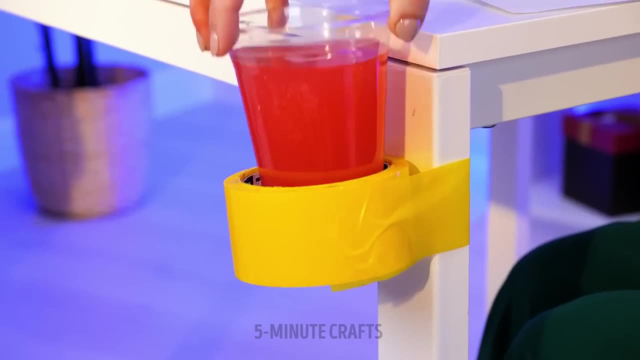 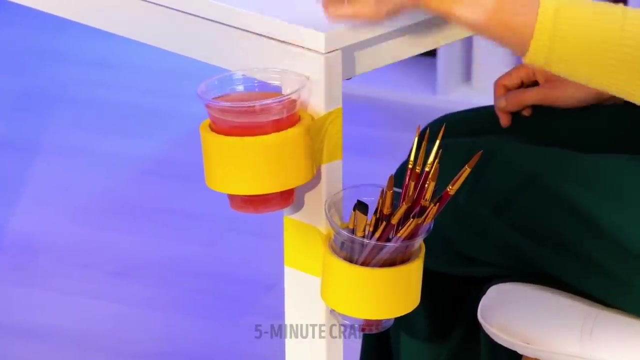 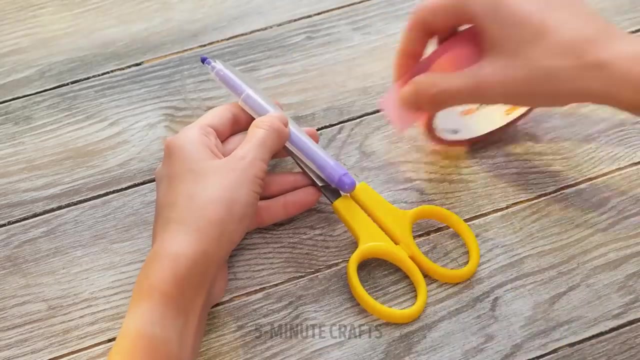 glass after glass, i keep hoping you'll come around drowning. i'm fighting what whatever can be found, cause i've given in to all my demons lately. you know, might be easier just to let it go, cause the cable's short and the problems all might be easier. 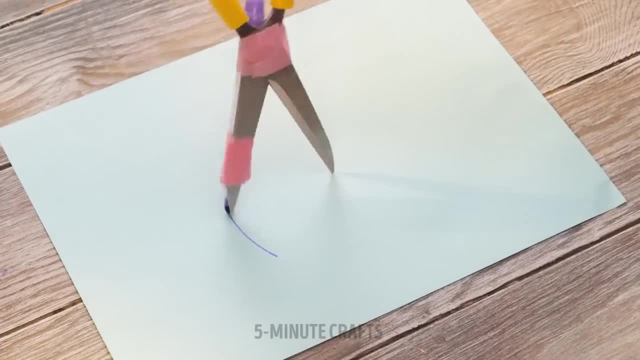 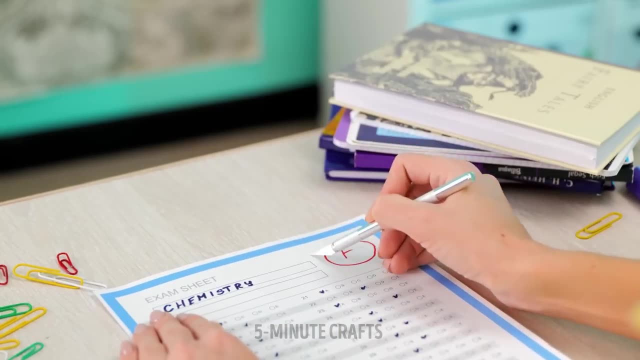 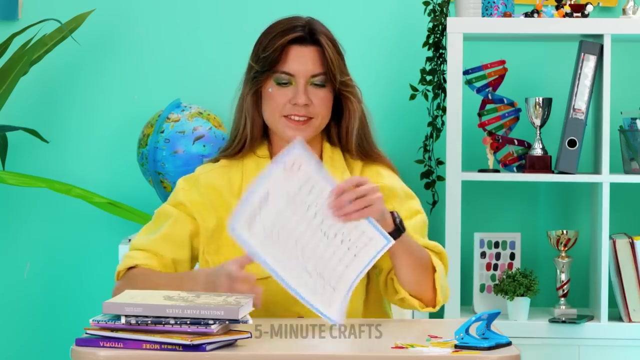 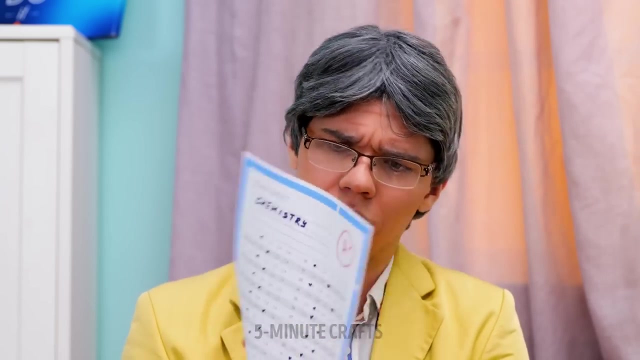 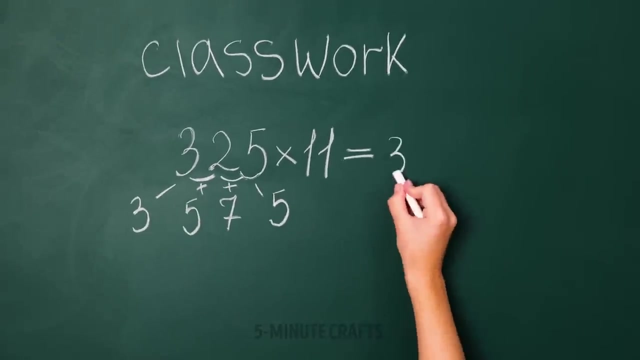 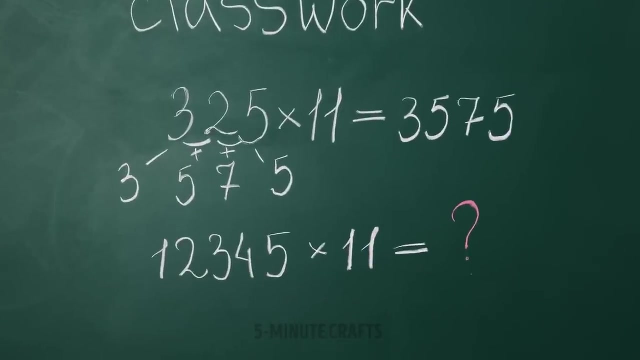 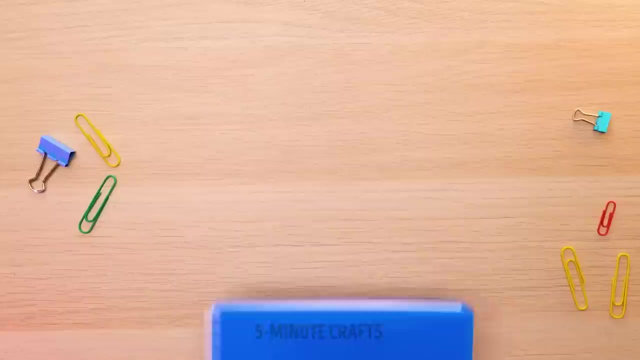 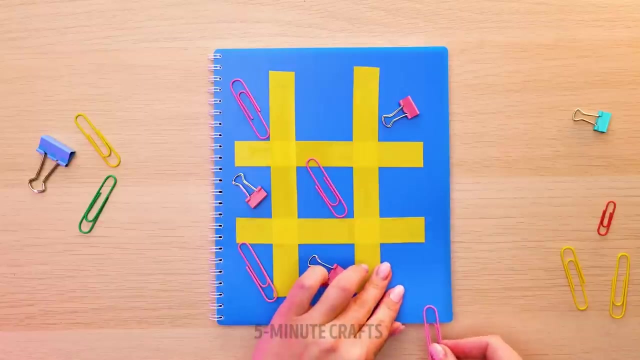 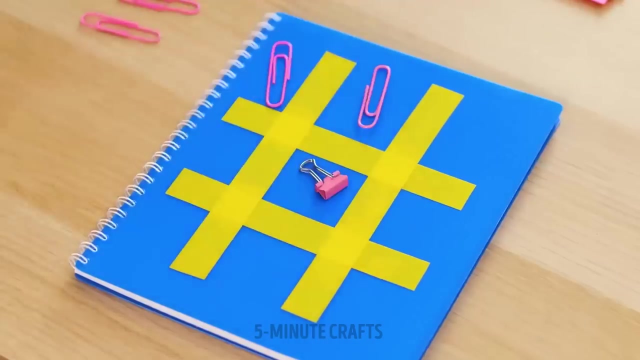 for you. i do it all night. you're my only last sign for me, baby. i've been waiting for a lifetime. just keep on fading in all these photos, calling the memories and capturing the highlights. just keep on waiting. just keep on waiting might be easier. just to let it go cause the cable's short and the problems all might be easier. 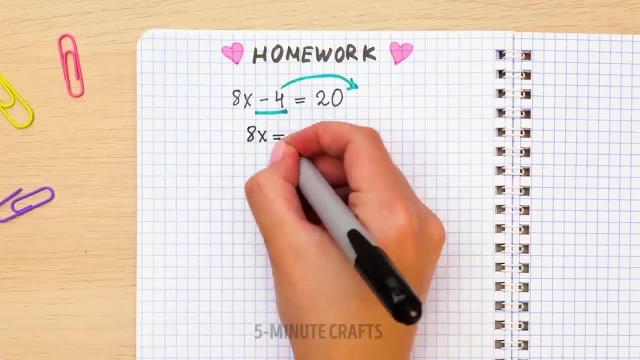 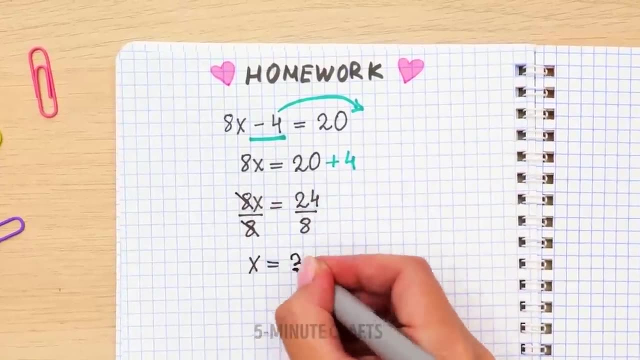 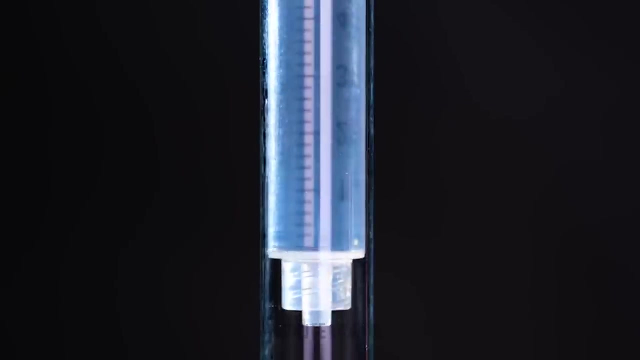 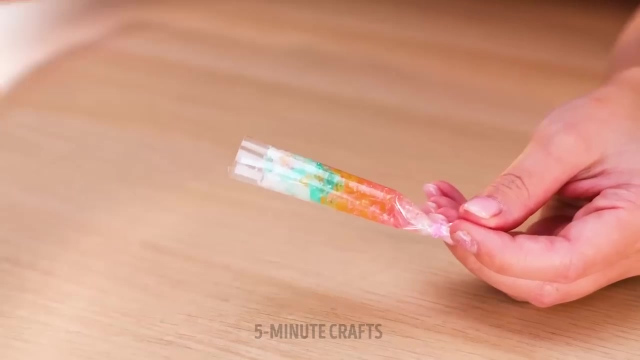 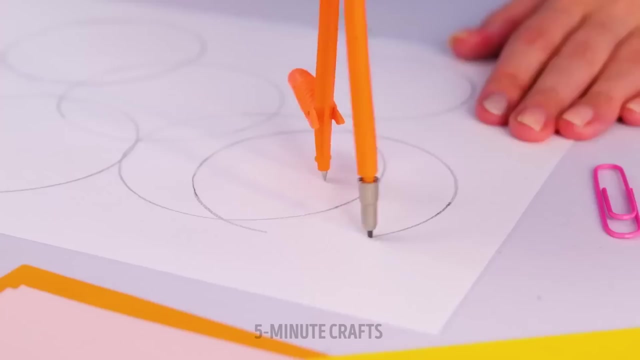 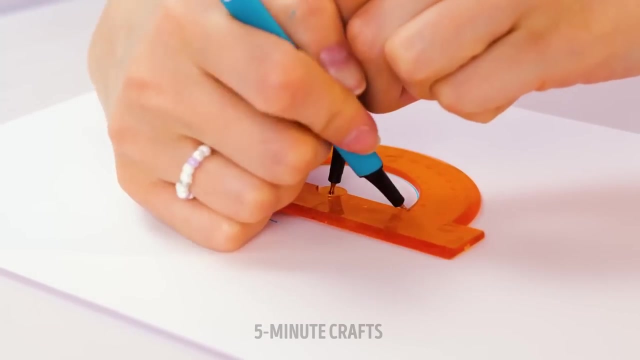 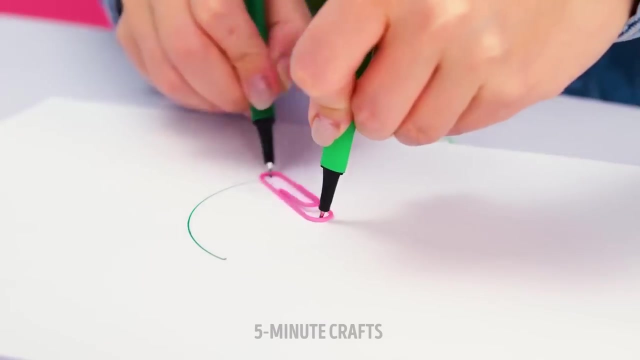 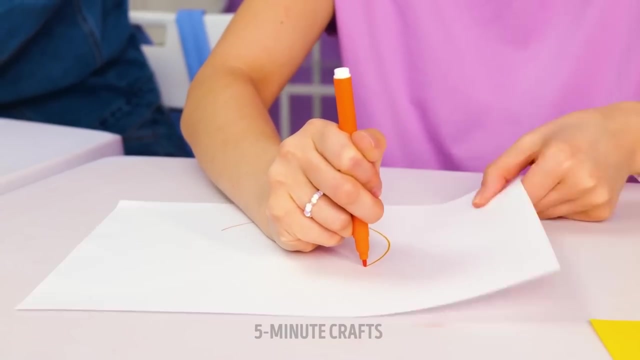 for you. i do it all night. you're my only last sign. i get so caught up in the middle thinking of drowning his blue eyes. i'm losing sight. cause i'm losing sight? cause i am falling. i'm so deep down, deep down, and it's not a lie. 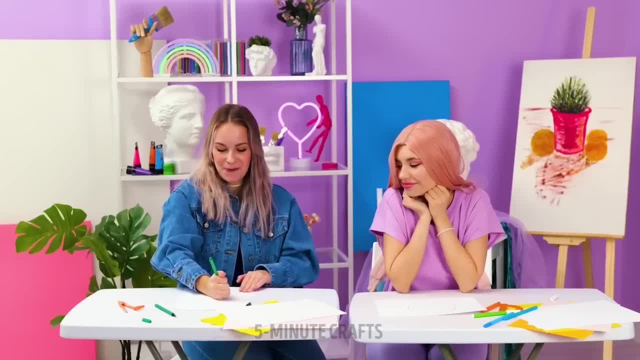 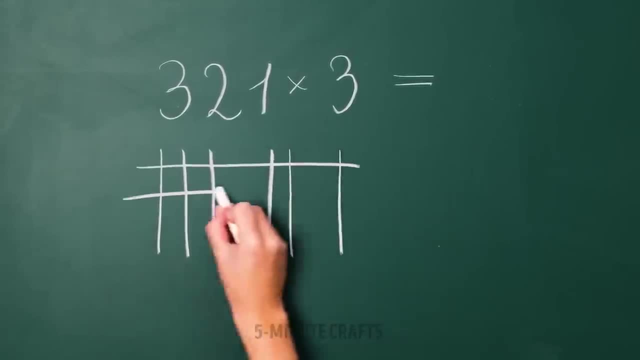 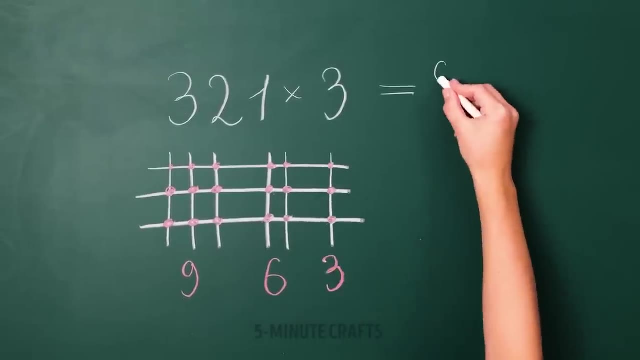 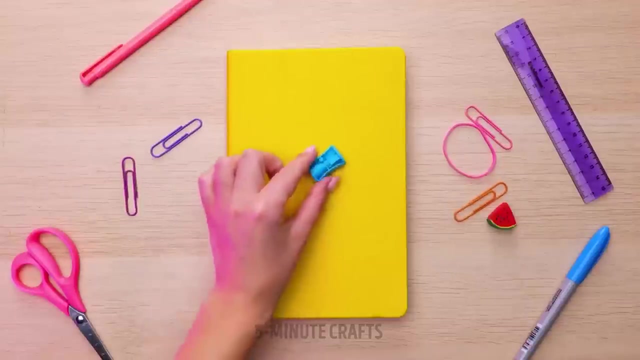 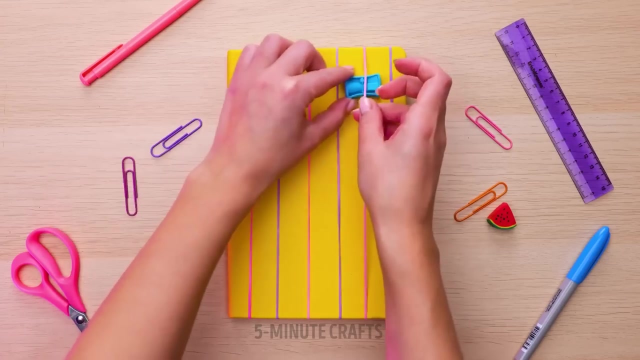 that i die. i can't hide what this is. yeah, i keep drowning. his blue eyes and you can tell me all the lies. i will put out all of the fire if it gets too dark. oh-oh, i'll be your light. ooh, be your light. 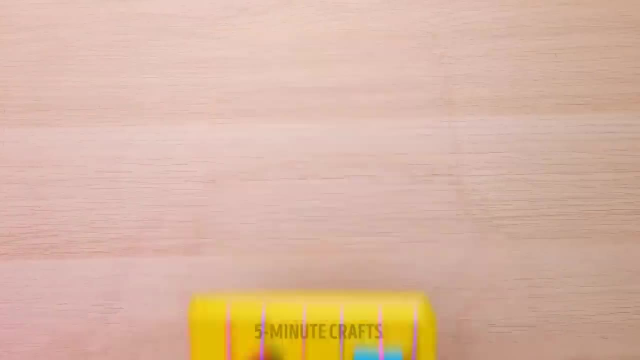 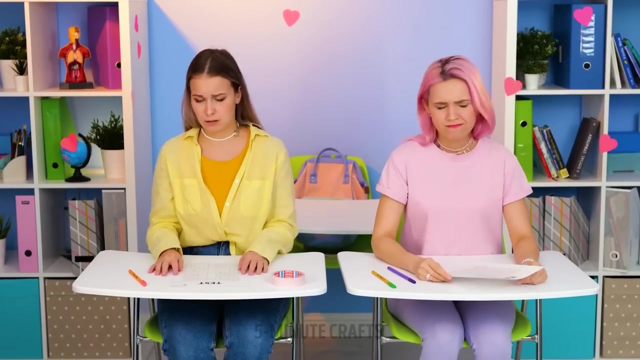 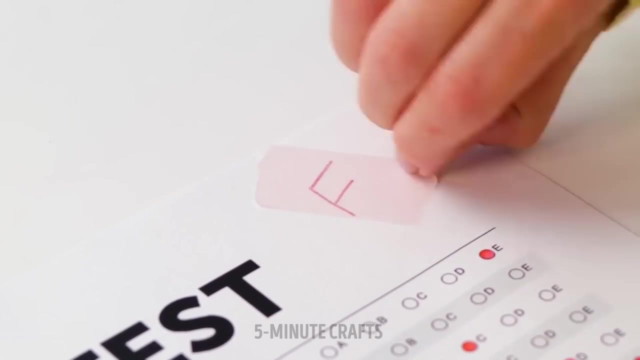 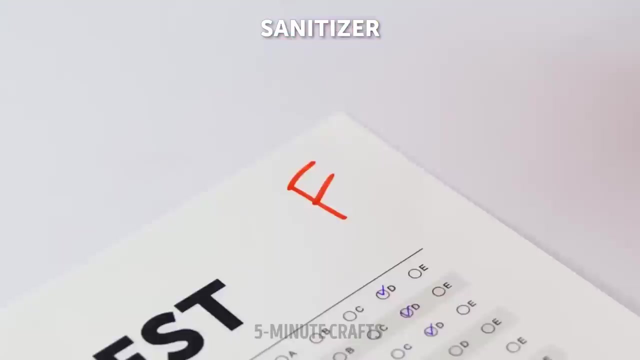 i'll be your light. ooh, if it gets too dark, oh-oh, i'll be your light. i'll be your light. be your light, be your light. I'll be your light. if it gets too dark, Yeah, I can carry all that you've got. 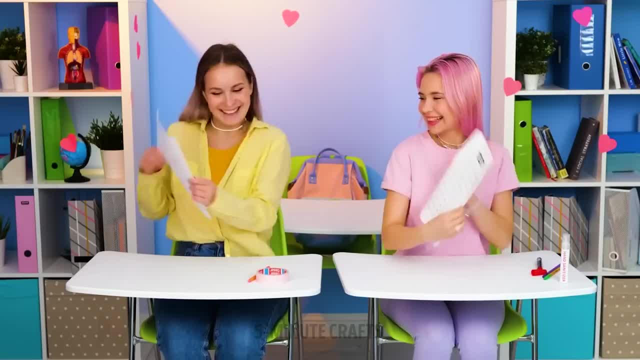 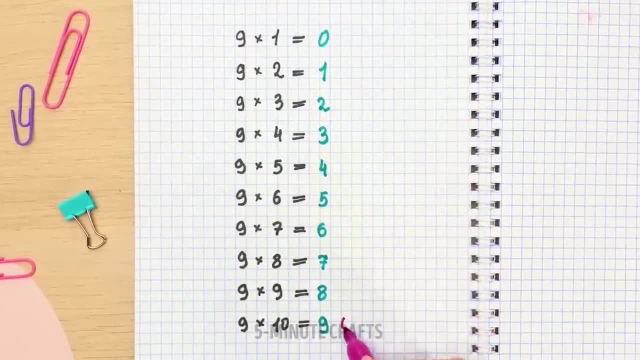 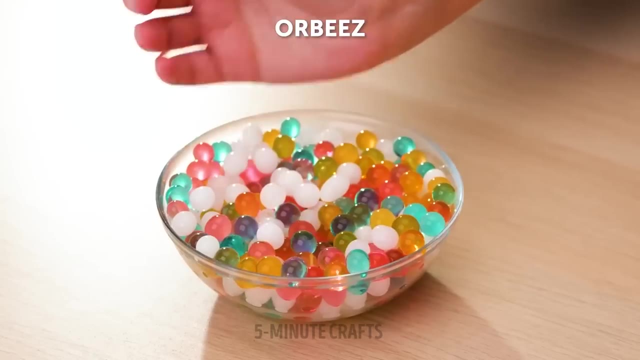 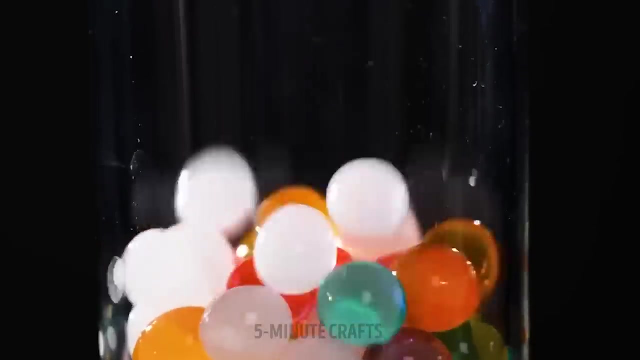 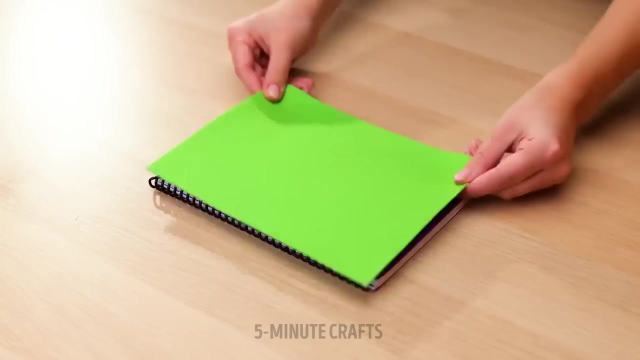 Two heavy hearts is not a lot. I will put out all of the fire. We stumble and fall And it's not a lie That I die. I can't hide What this is. Yeah, I'm too proud to use blue eyes And you can tell me all of your lies. 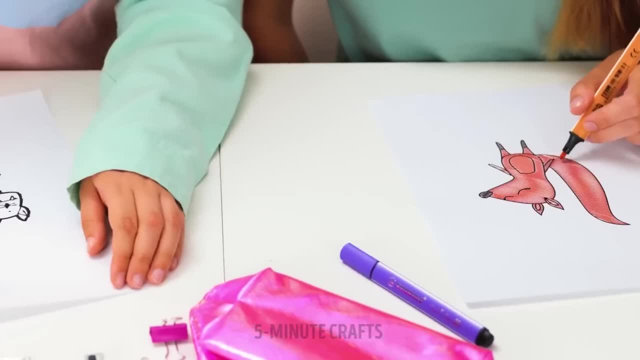 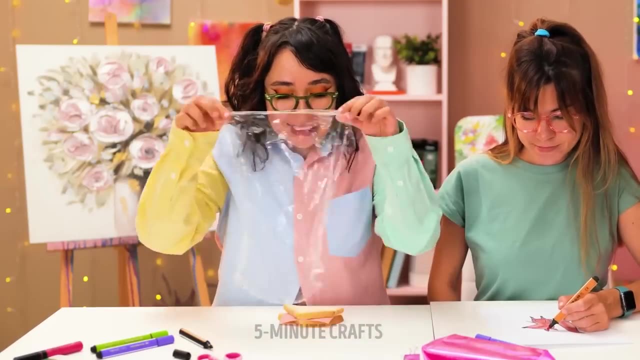 I will put out all of the fire. If it gets too dark, I'll be your light. I'll be your light. I'll be your light. If it gets too dark, I'll be your light. I'll be your light. I'll be your light If it gets too dark. 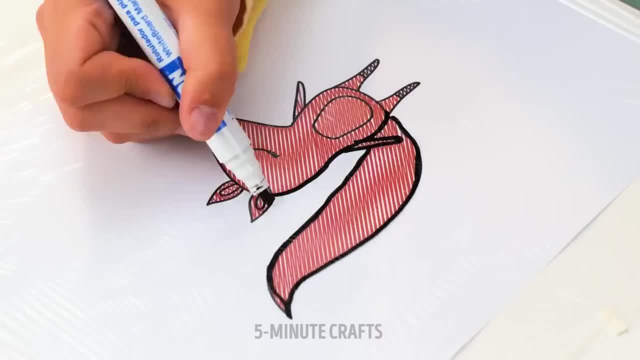 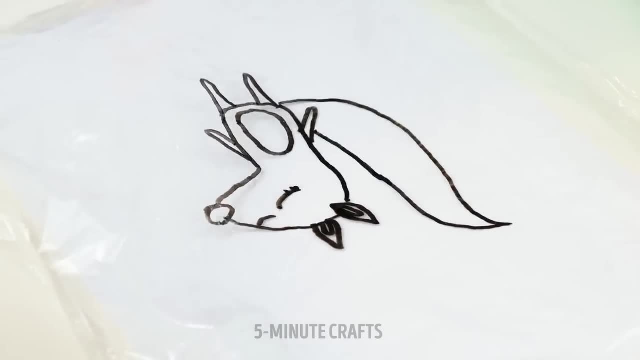 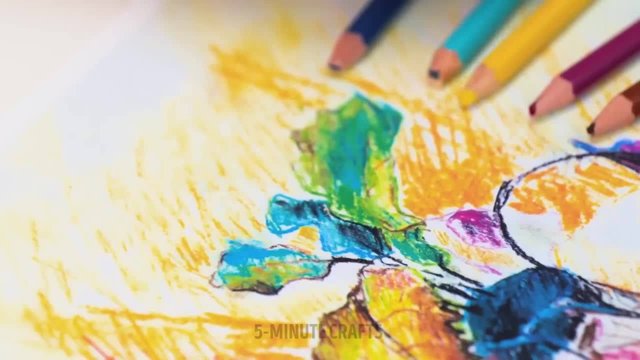 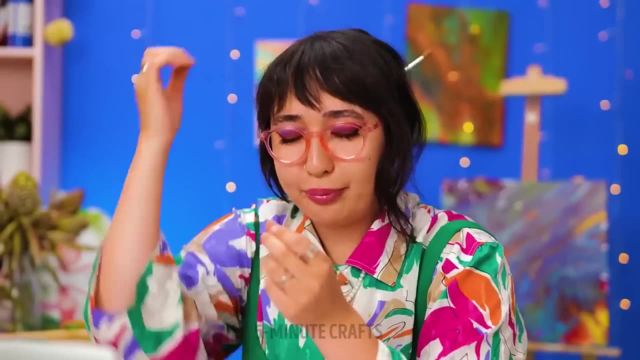 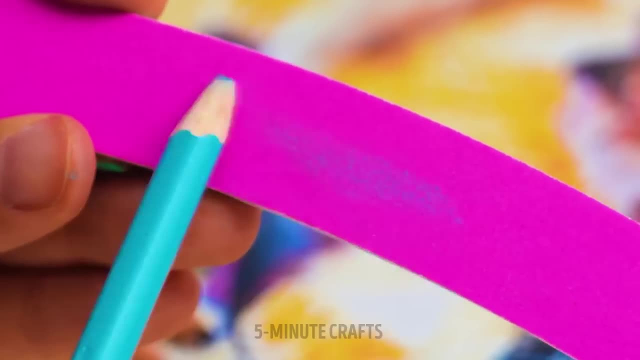 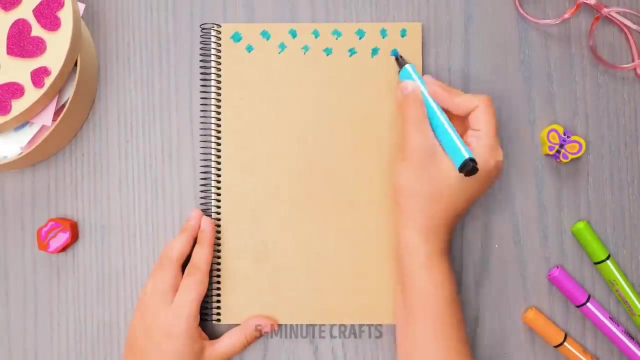 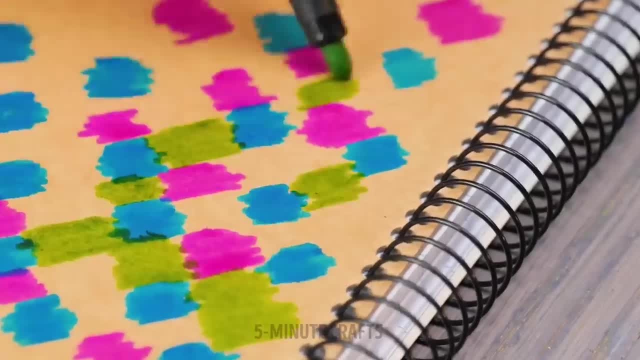 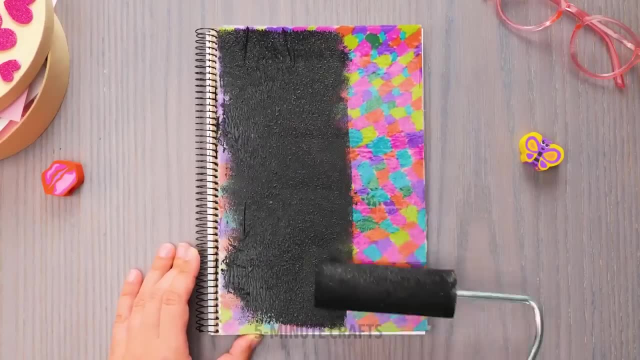 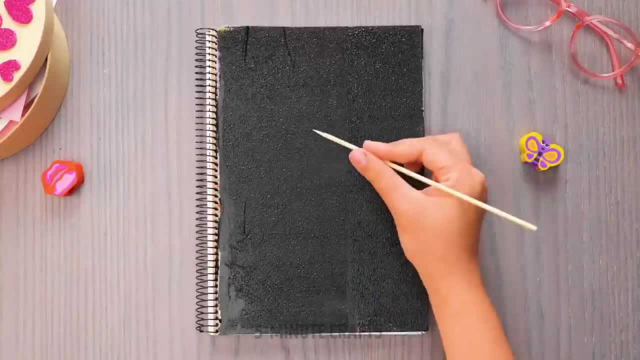 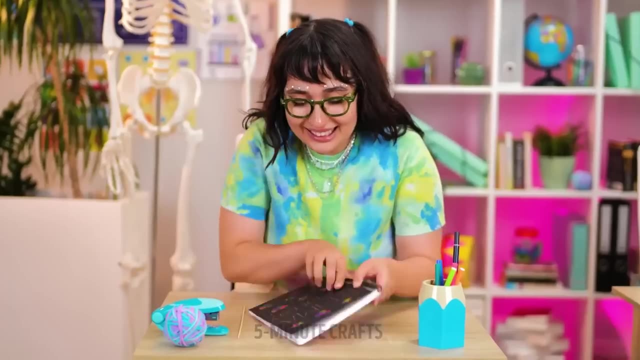 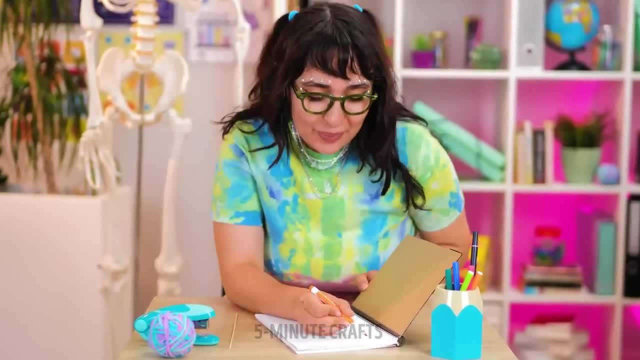 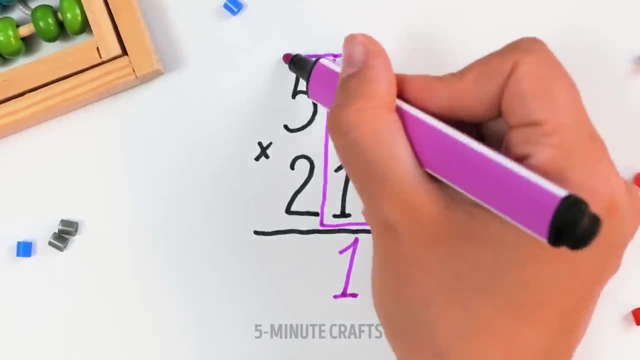 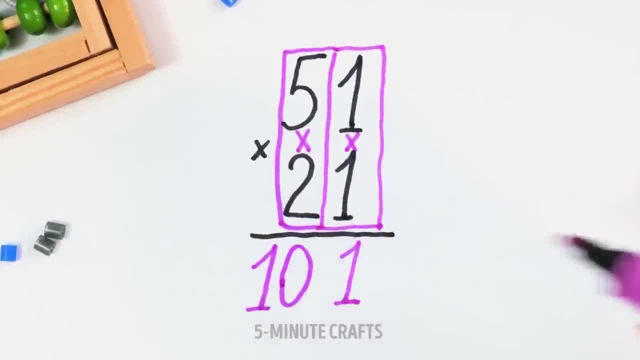 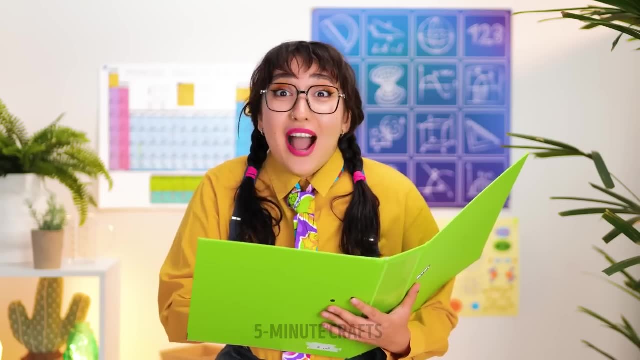 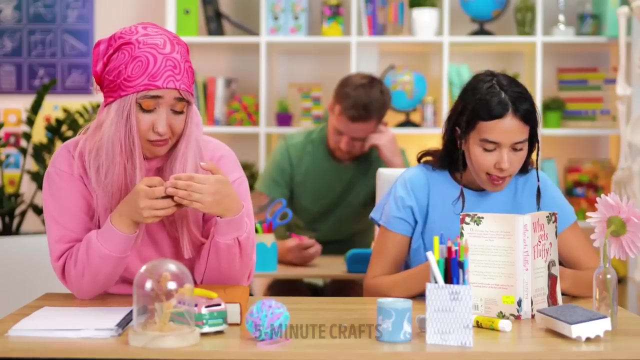 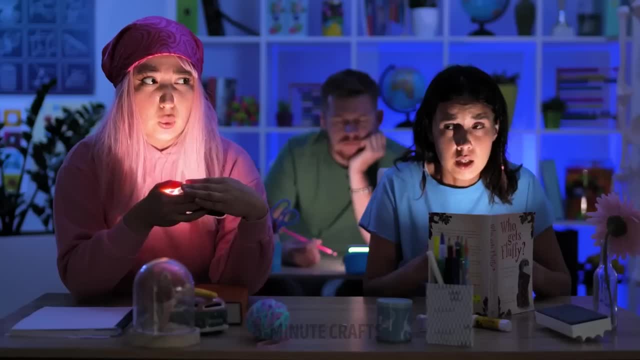 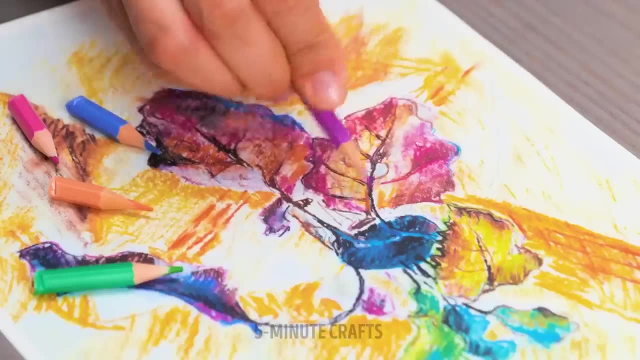 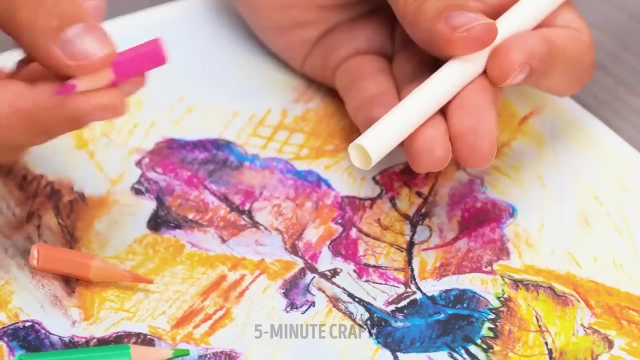 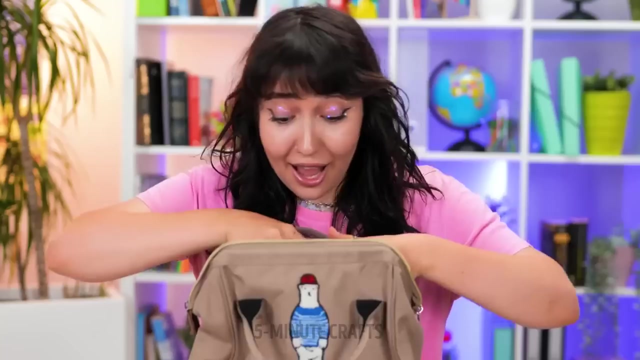 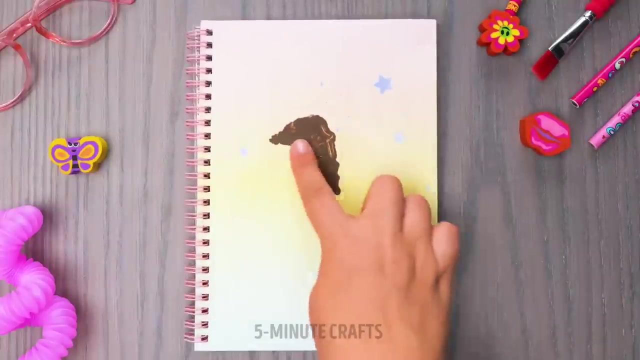 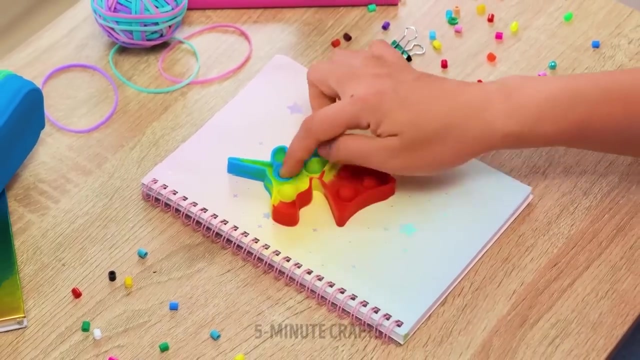 One touch The feet asking me, The feet asking me. The picture. perfect, I'm a serving, I'm a serving, I'm a serving. Ooh, Ooh, Ooh, Ooh. Everything will probably go In and out. I know One thought and we break Airborne as we face. 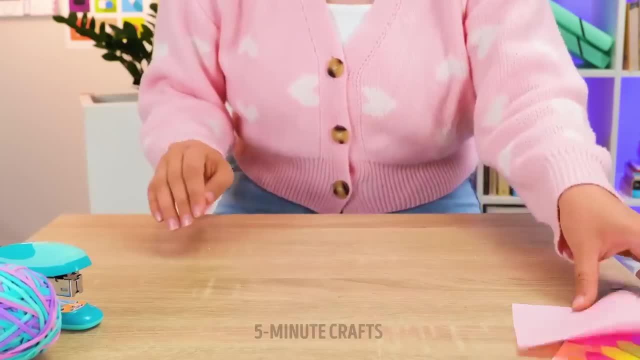 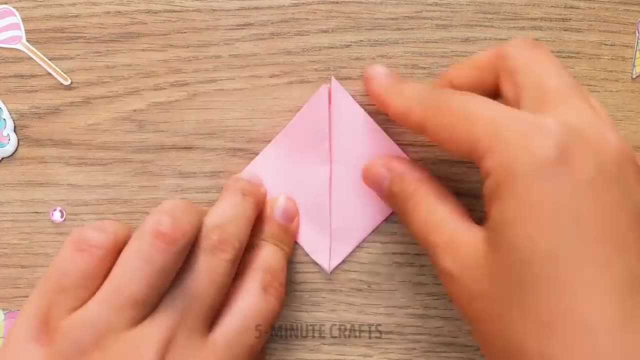 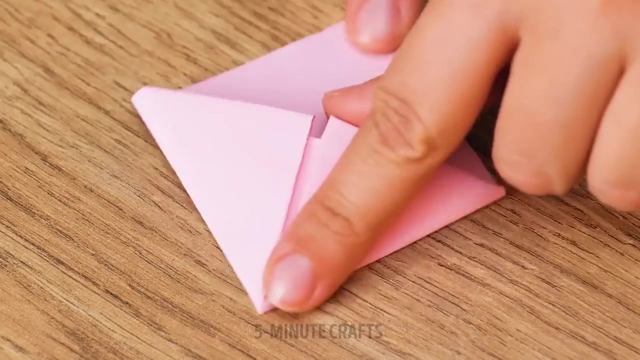 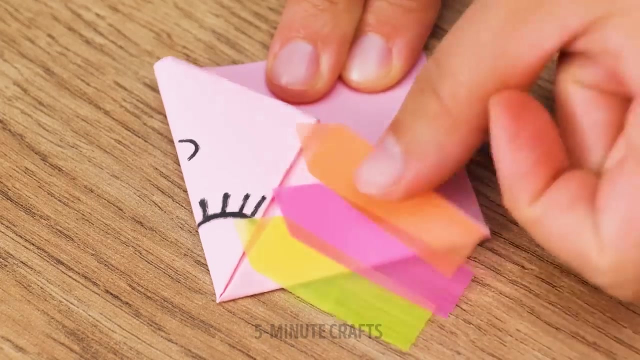 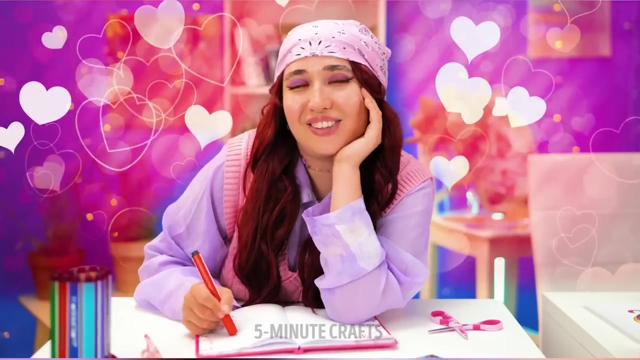 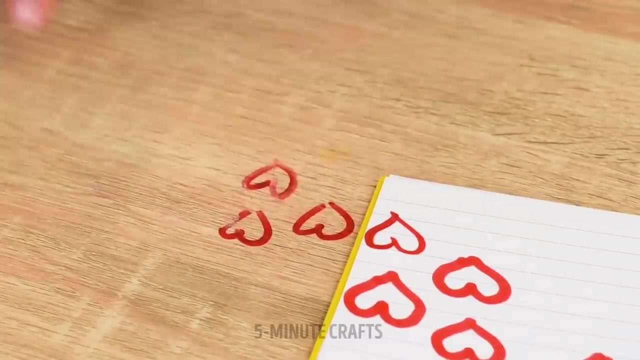 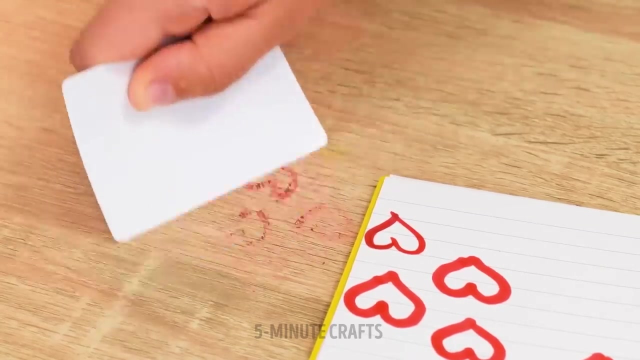 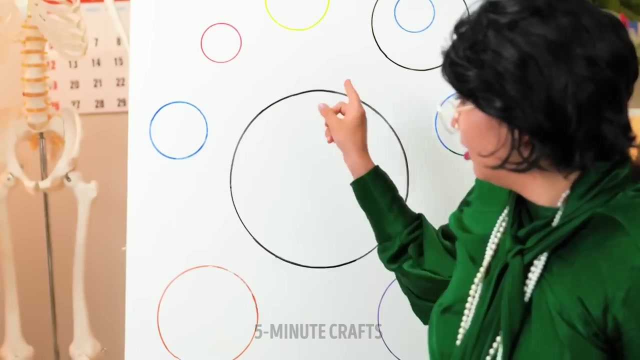 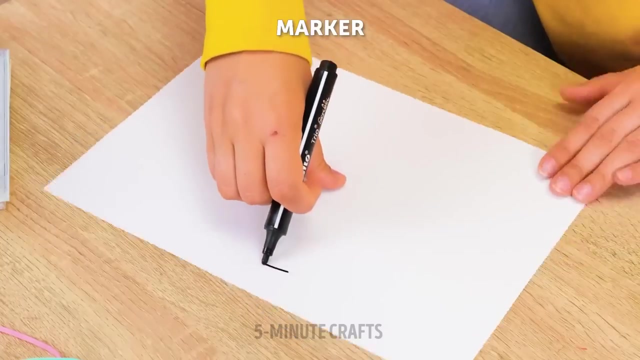 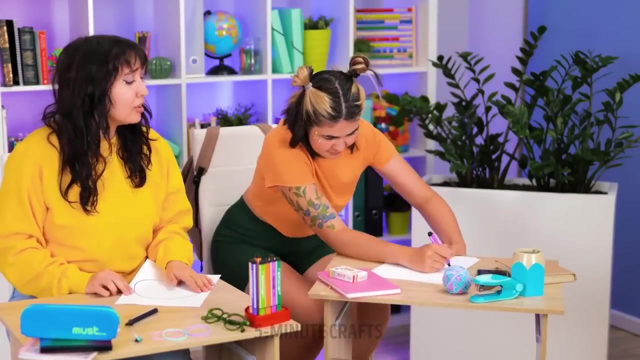 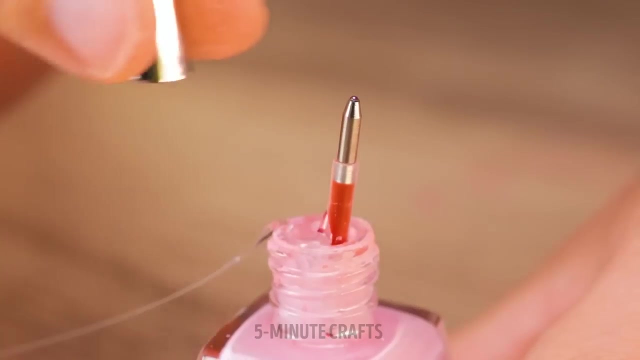 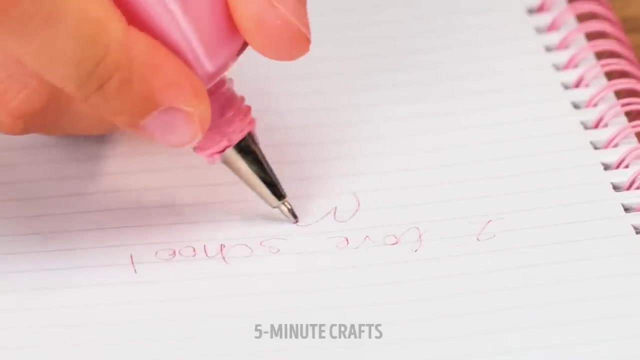 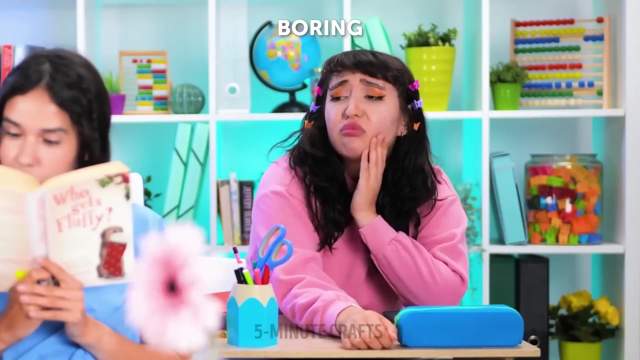 Misconceptions, picture perfect, A balanced plan. let's all pretend: In and out, I know. Give me through, give me through All the layers of you, Give me through, give me through. In and out, I know. In and out, I know. 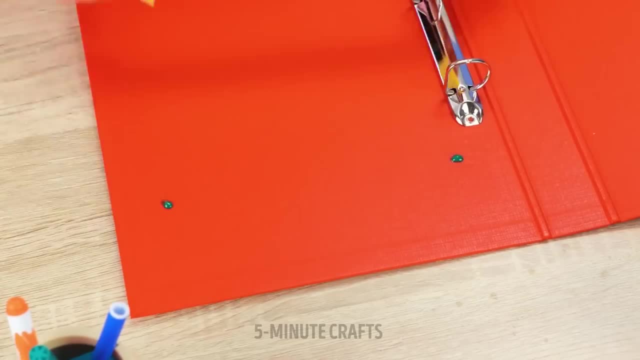 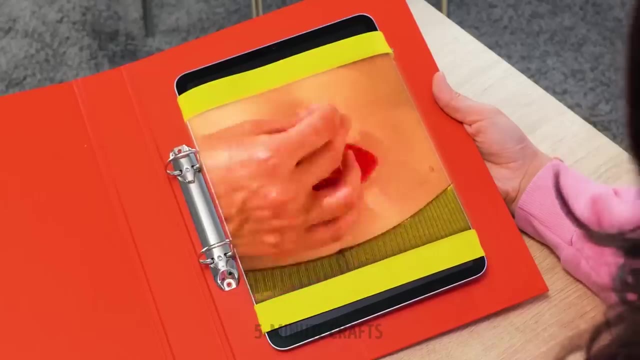 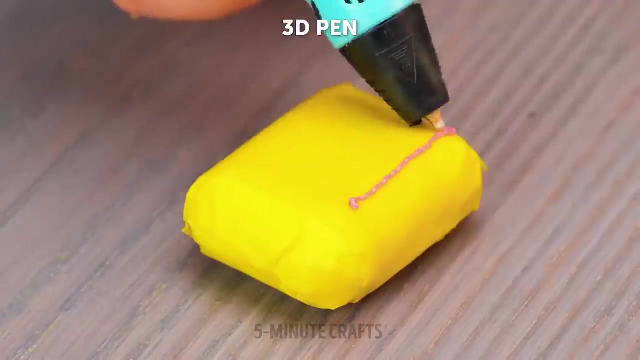 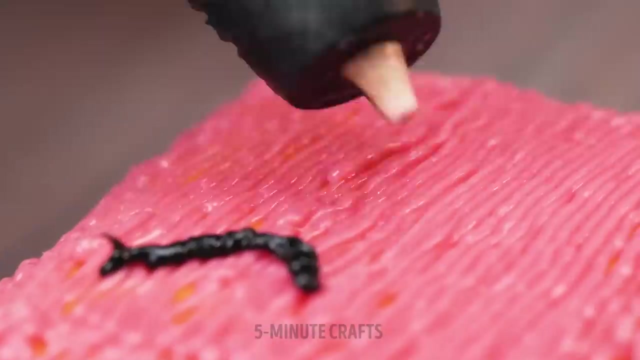 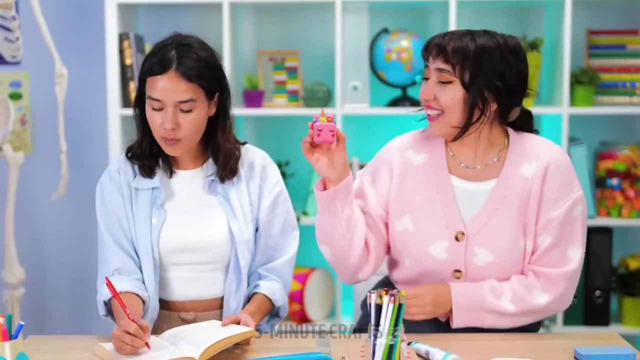 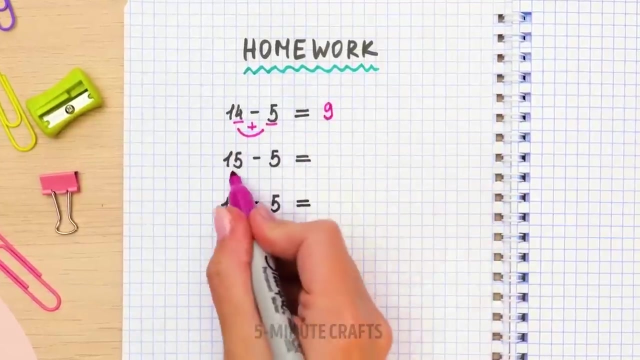 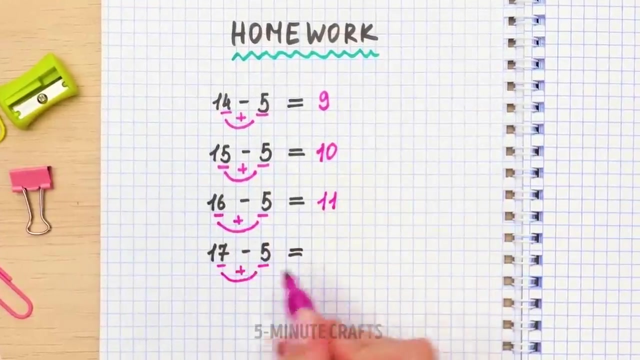 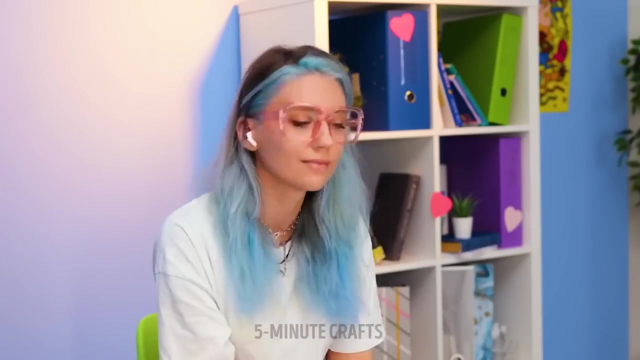 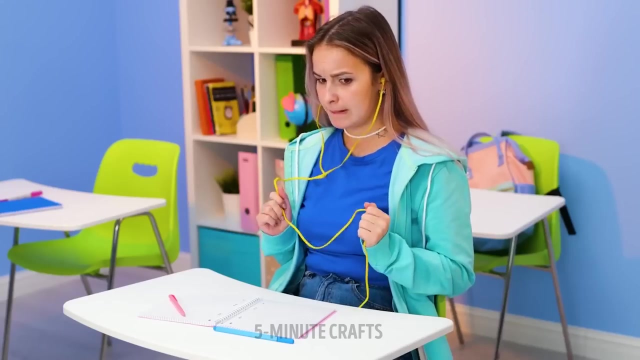 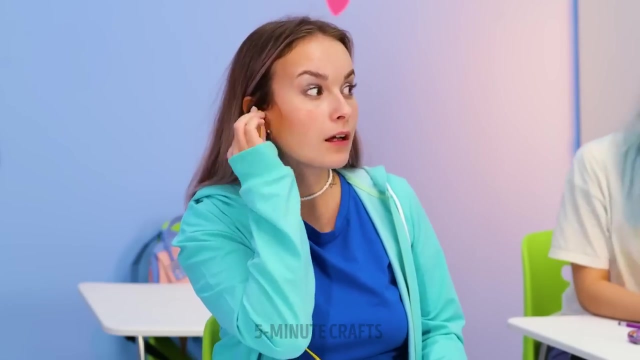 In and out. I know. Put your body on the kitchen table And move the dishes to the side Girl, you always tend to drive me crazy, Looking at me with those eyes. Put some music on. Turn the lights down low. Throw the pillows off the bed. Throw the candles out. 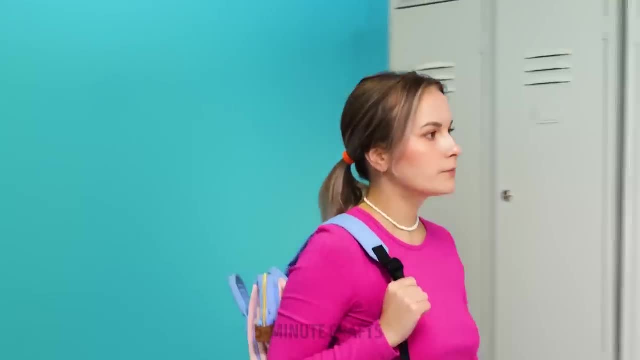 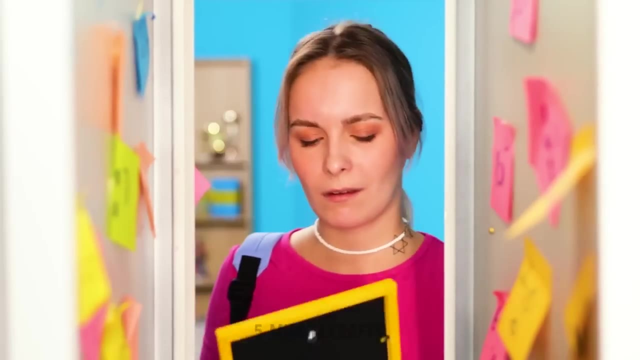 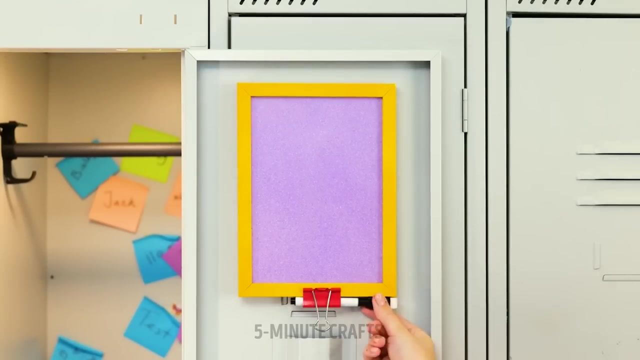 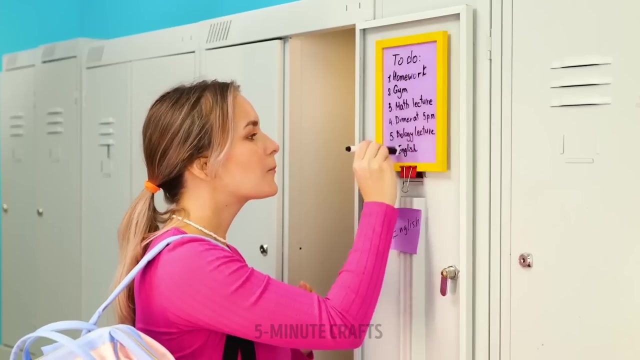 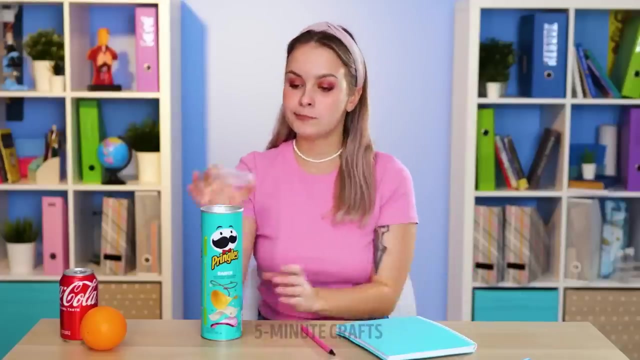 Move your body slow. You got something on your mind. I'ma try to help you, let it go. Try to help you, let it go. Try to help you, let it go. Baby, I still wear the shirt you gave me, Cause it reminds me of the times. 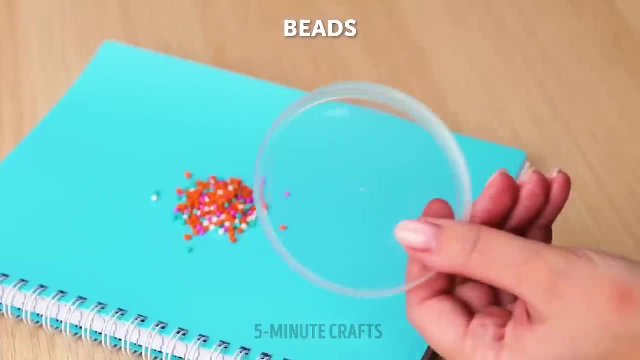 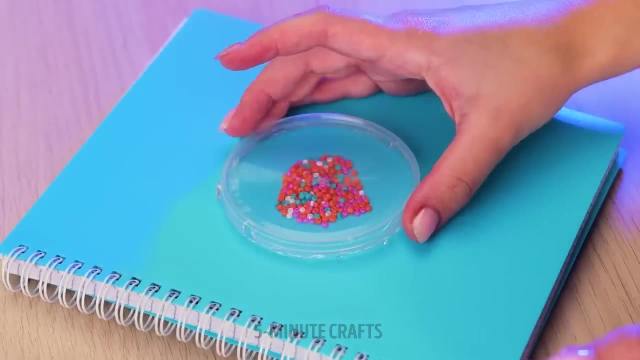 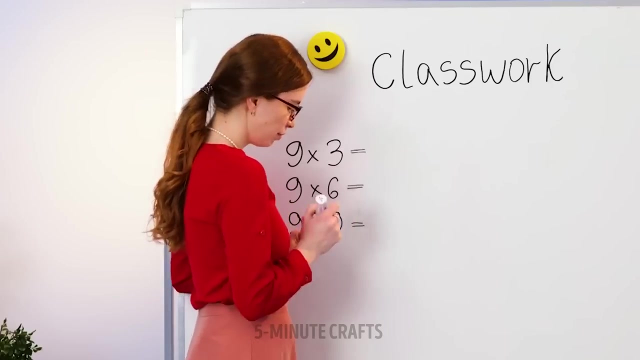 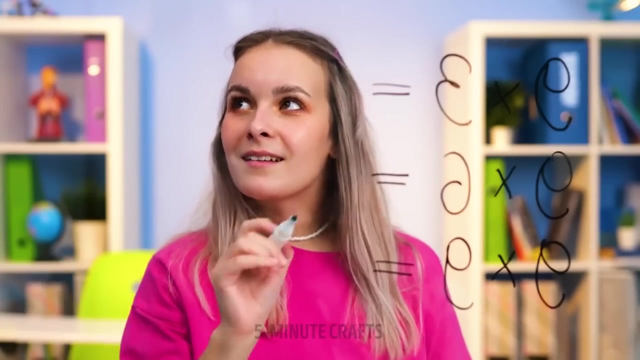 When I was down and you were there to save me, Telling me that I'll be fine. Put some music on. Turn the lights down low. Turn the lights down low. Throw the pillows off the bed. Throw the candles out. Move your body slow. You got something on your mind. 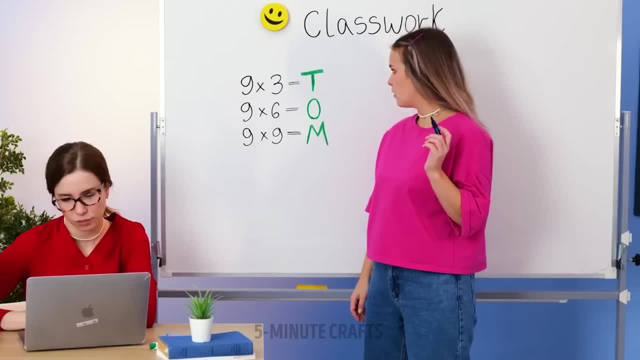 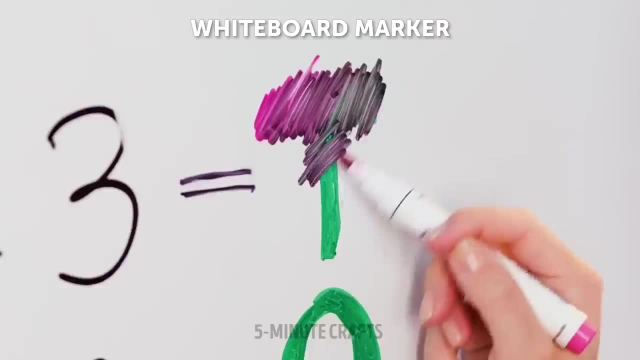 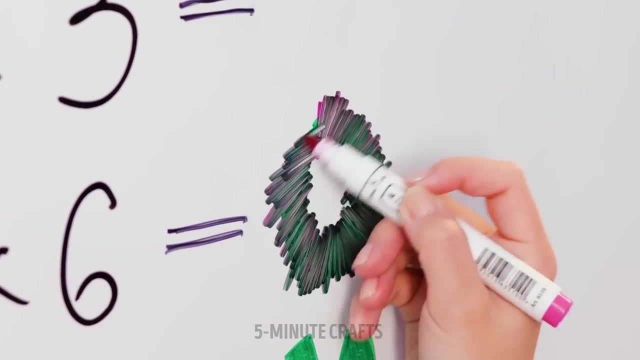 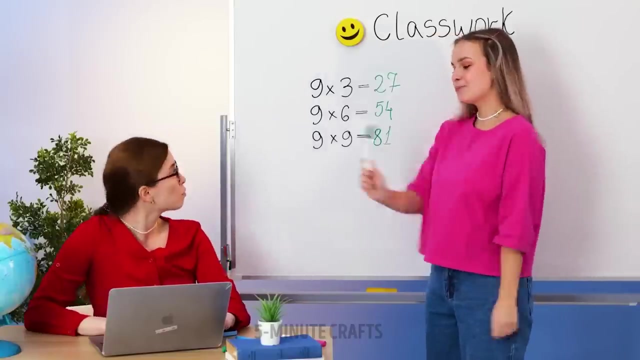 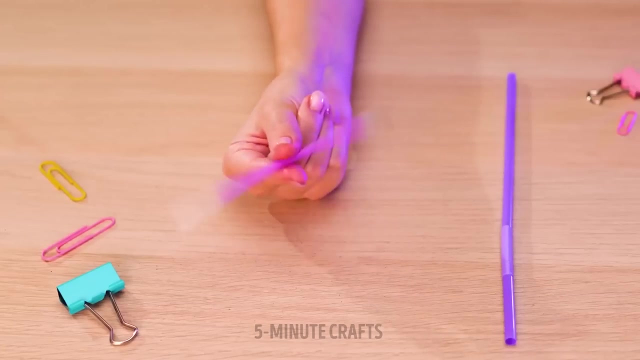 I'ma try to help you, let it go. Try to help you, let it go. Try to help you, let it go. If you got something on your mind, I'ma try to help you. let it go. You got, you got. you got something on your mind. 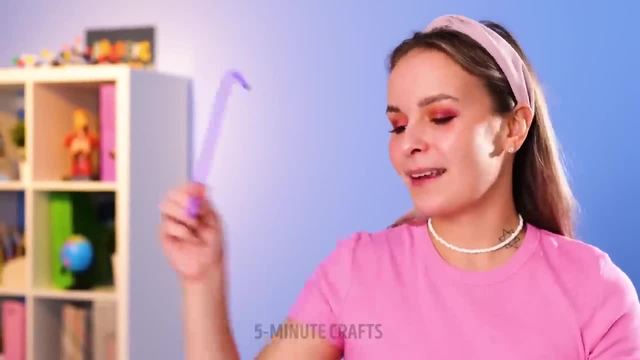 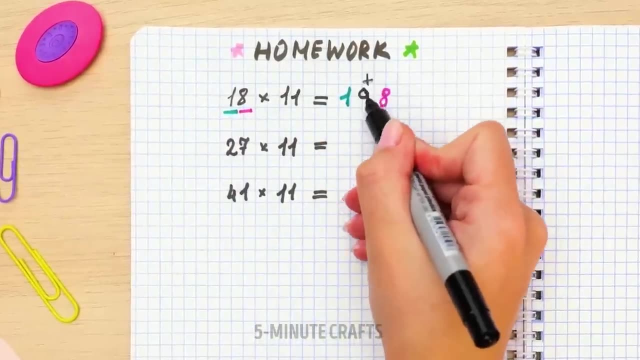 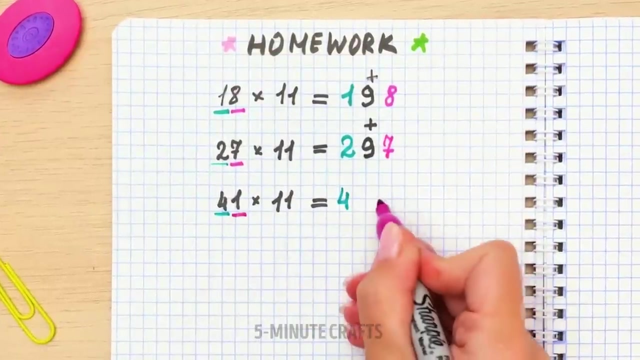 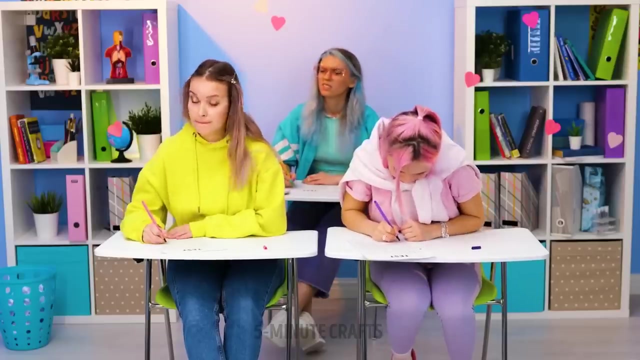 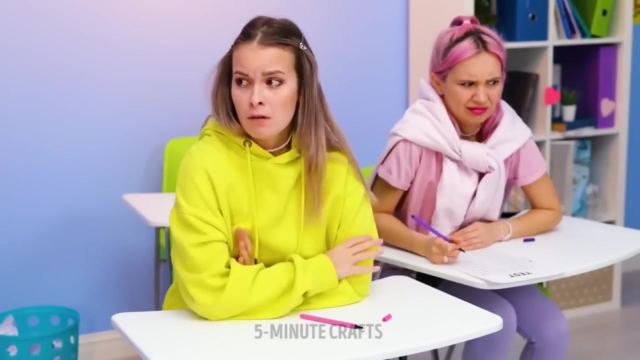 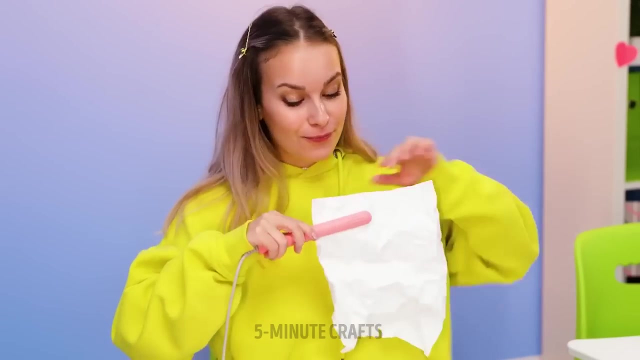 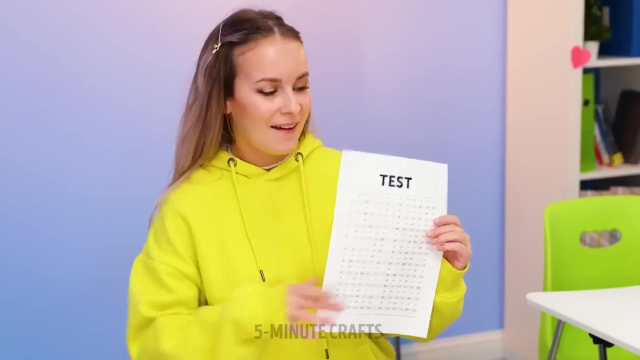 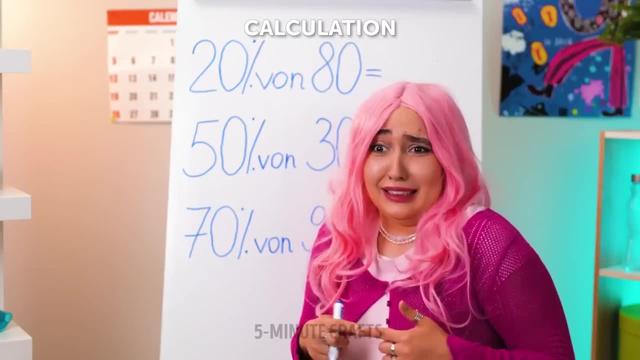 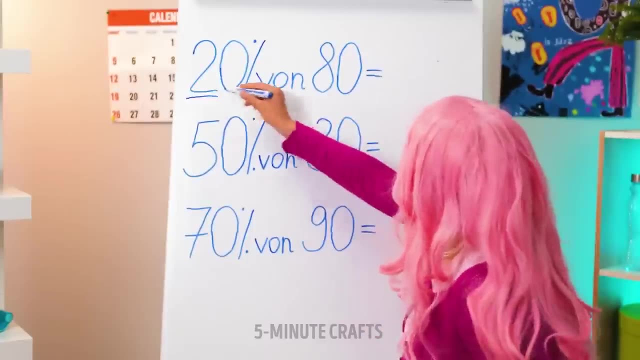 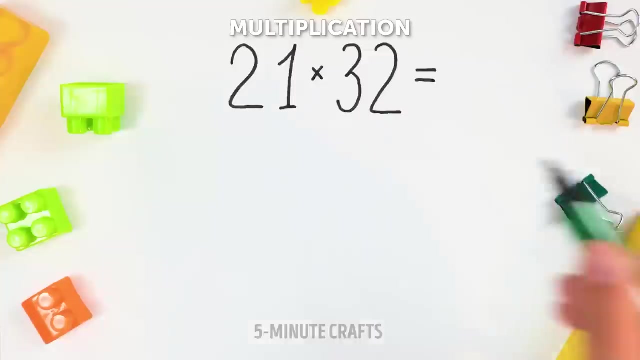 We're gripping on mistakes. See, that's so head over heels crazy. Need to apologize. We went too far this time. Come a little closer. There's something I have to say: I love you and I hate you, And I hope you feel the same. Come a little closer, baby. 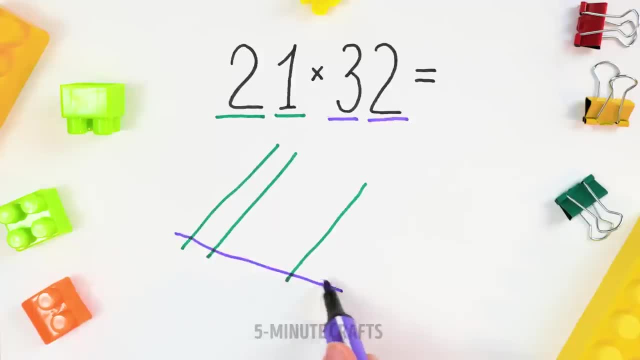 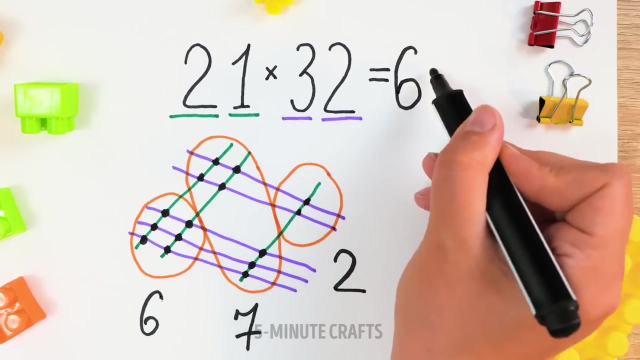 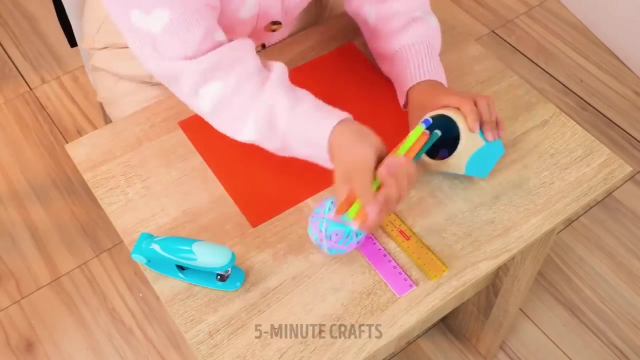 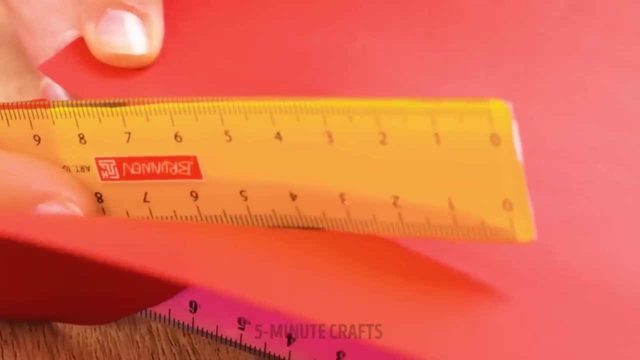 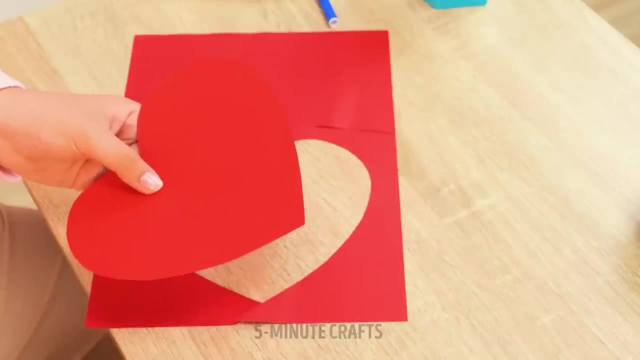 Please don't walk away. I love you and I- yeah, You got nothing to prove. oh baby, I know, Don't drive by me, I'll drive by you. You got nothing to prove. oh baby, I know, We got this. It's way too easy to say stuff I never do. 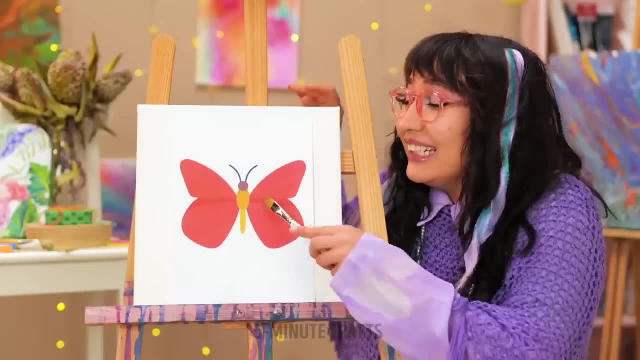 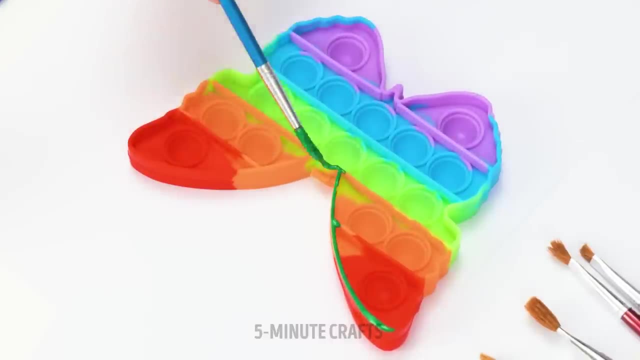 You know it's not how I feel, baby, So can we let this slide? Can't stand to see you cry. You got nothing to prove. oh, baby, I know, Come a little closer. There's something I have to say: I love you and I hate you. 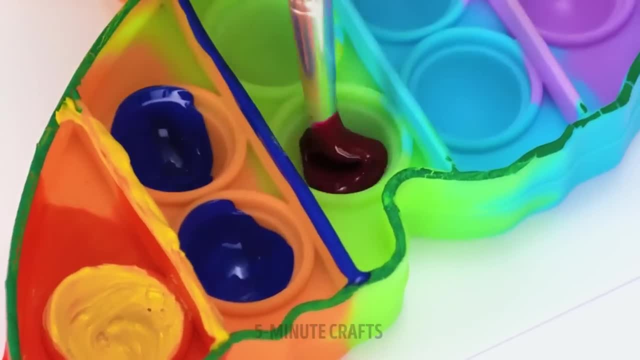 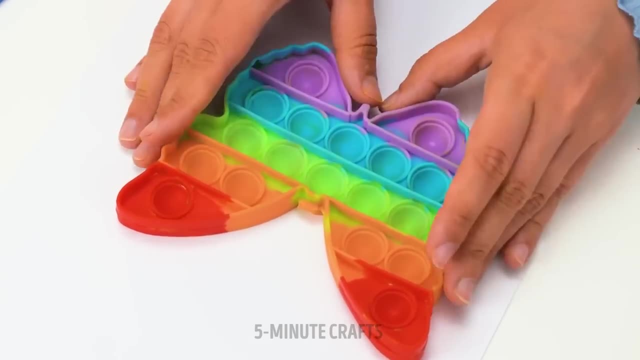 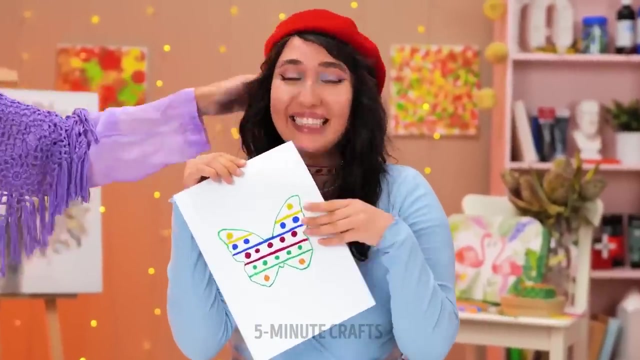 And I hope you feel the same. Come a little closer, baby. Please don't walk away. I love you and I- yeah, You got nothing to prove. oh baby, I know. Don't drive by me, I'll drive by you. You got nothing to prove, oh baby, I know. 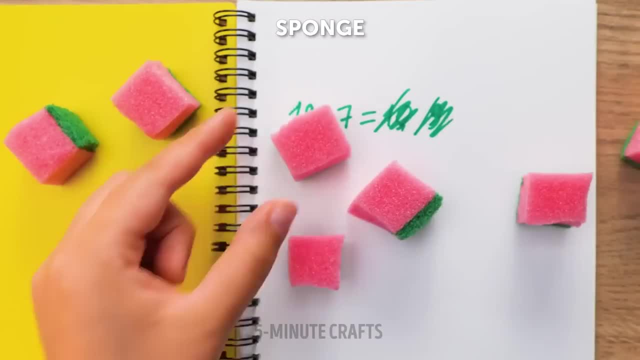 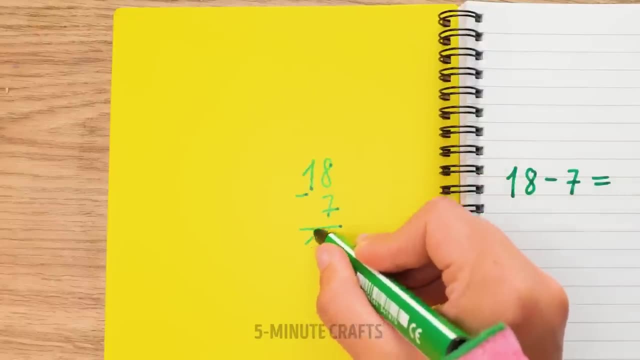 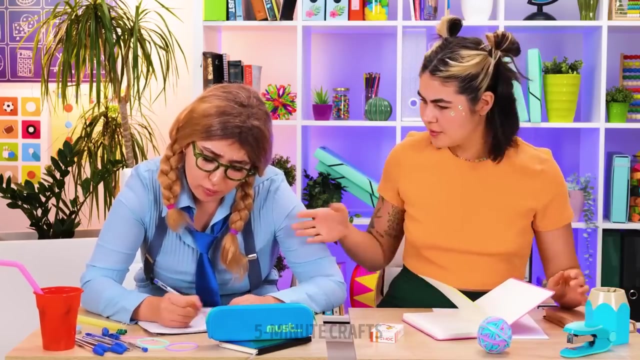 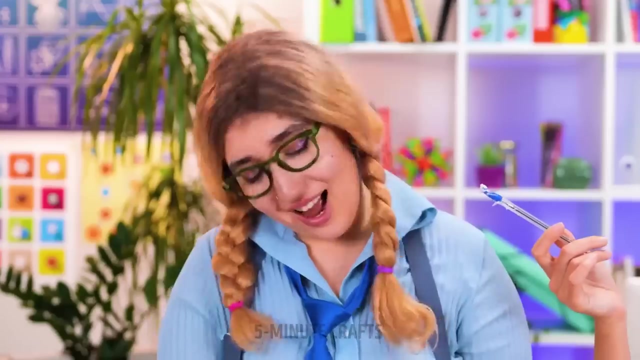 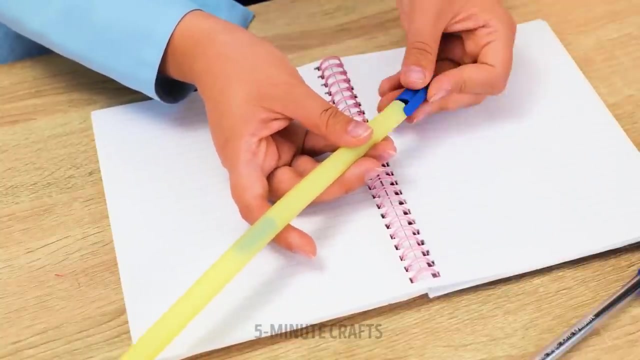 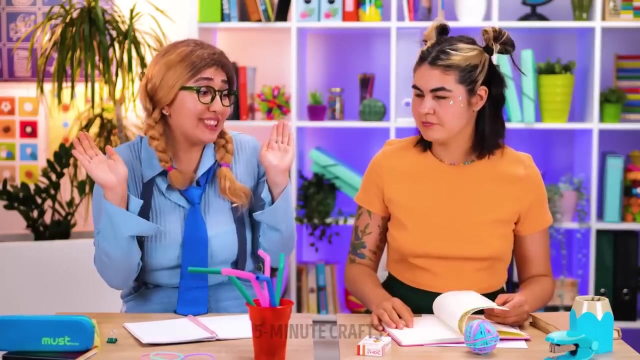 Ohhh, olvidin' to know, Leave it to me- said the bicycle: You got this A little closer. baby, I know We got this, Come a little closer. there's something I have to say: I love you and I hate you and I hope you feel the same. 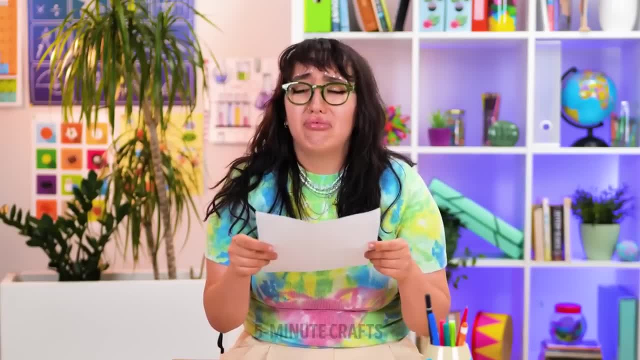 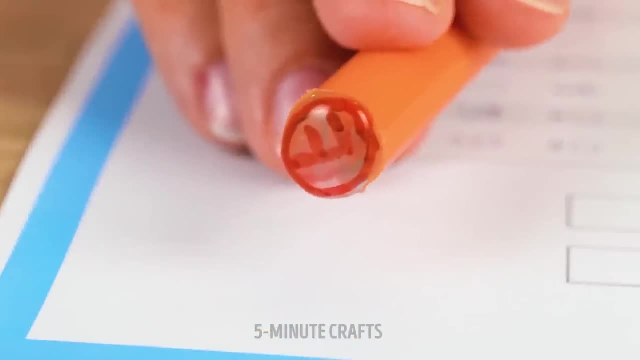 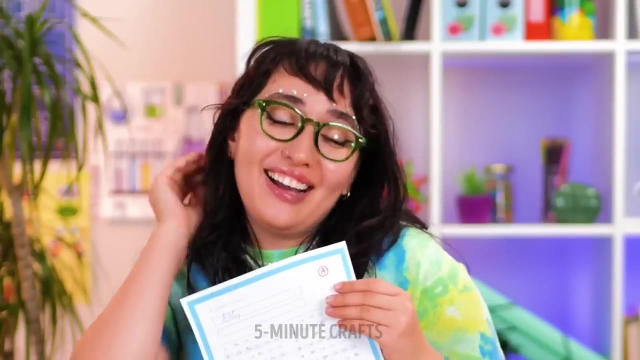 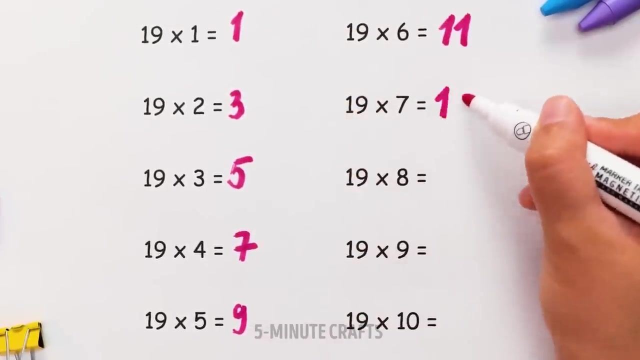 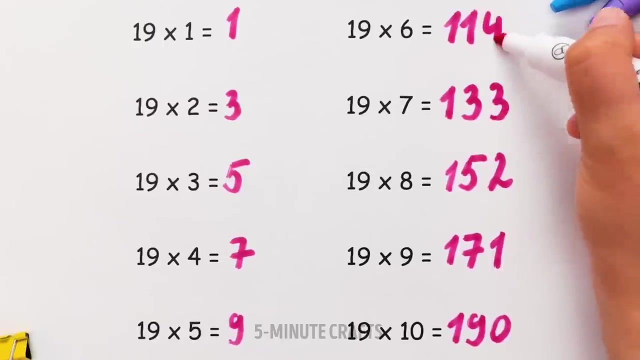 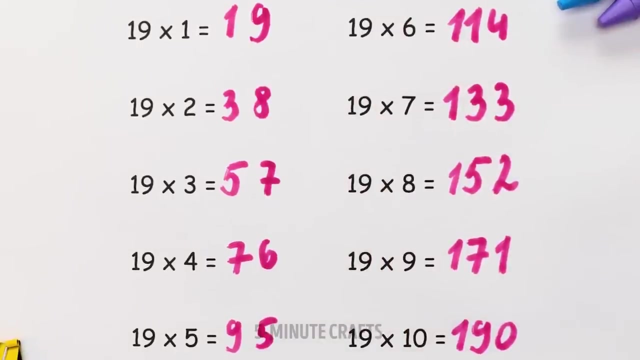 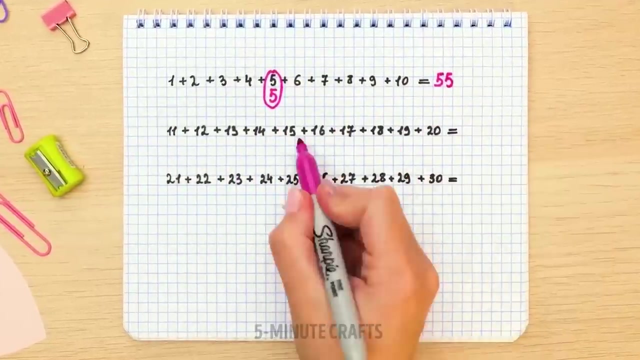 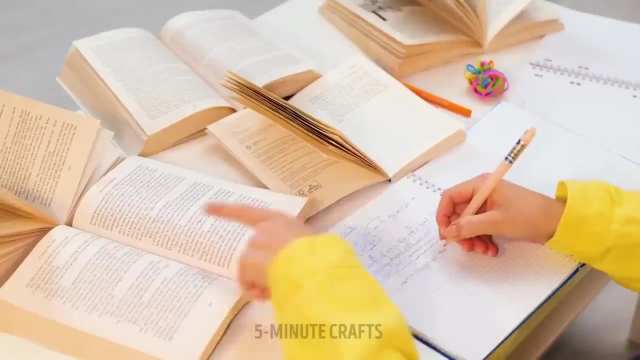 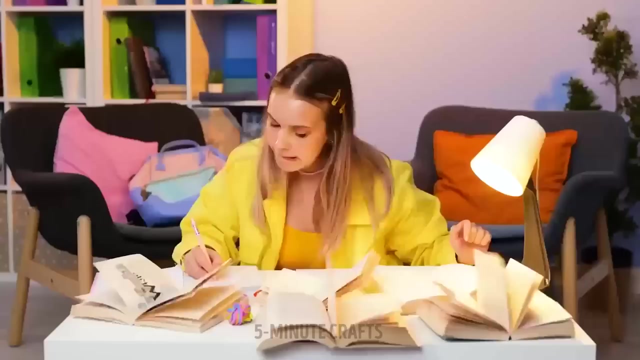 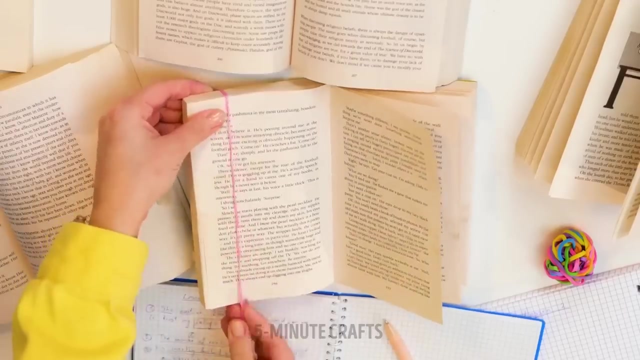 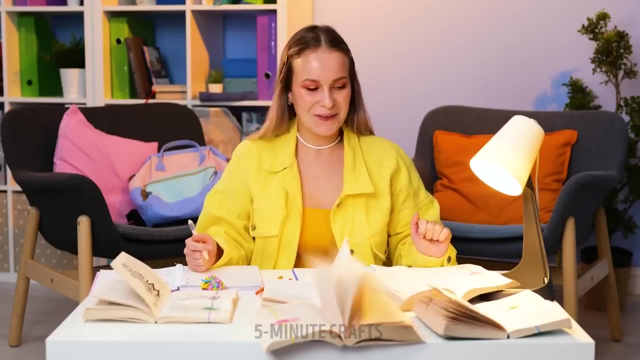 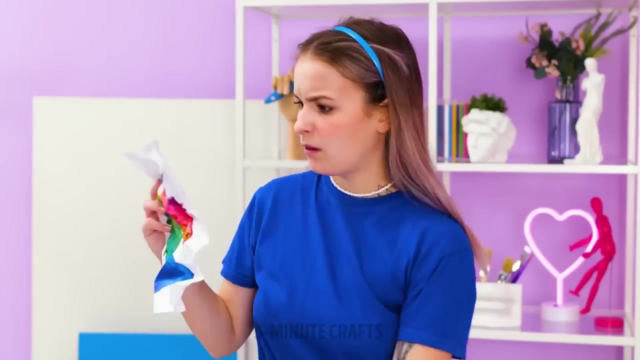 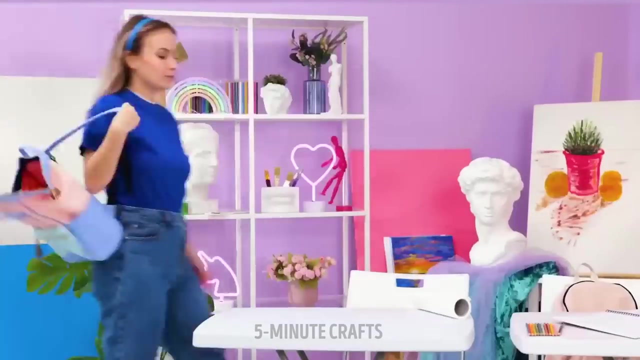 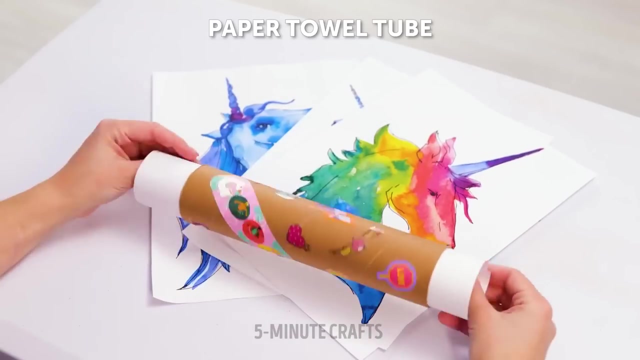 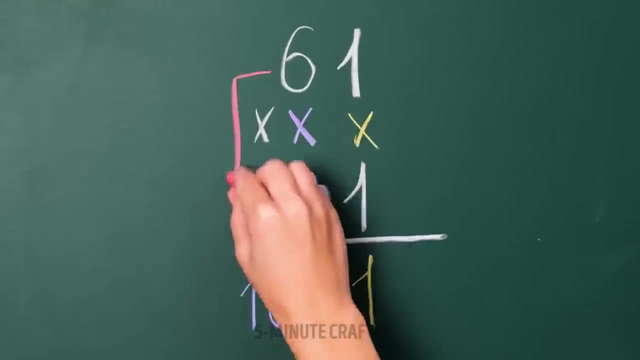 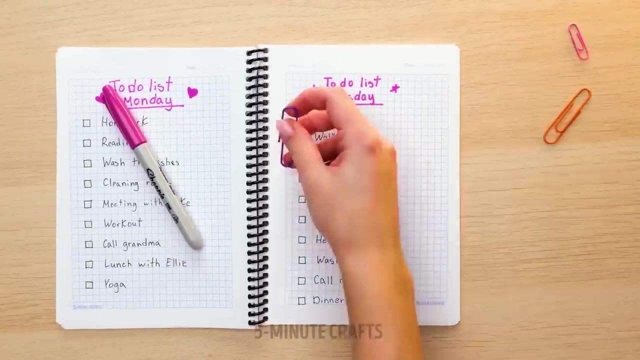 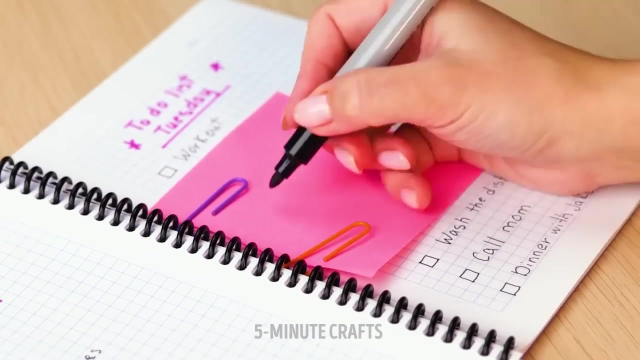 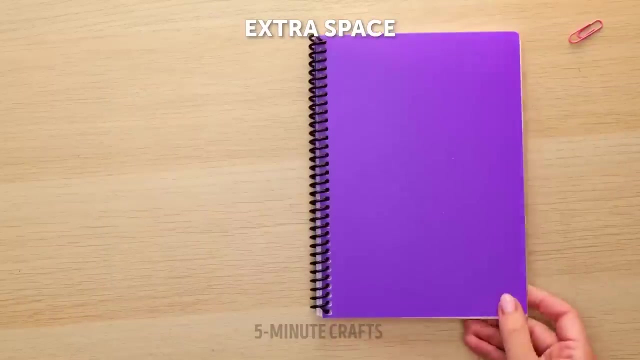 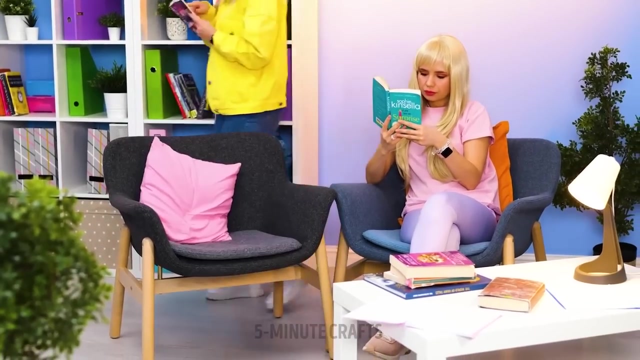 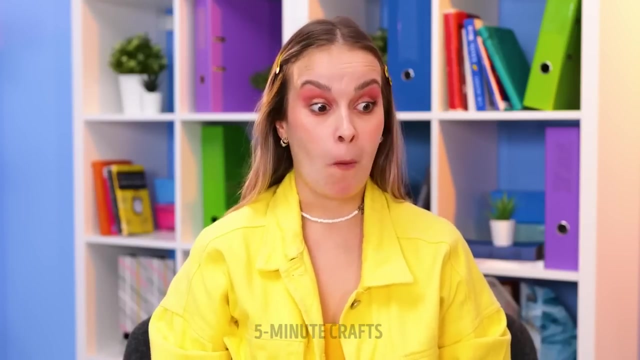 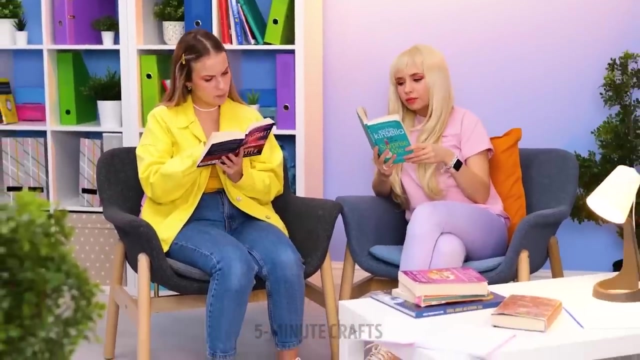 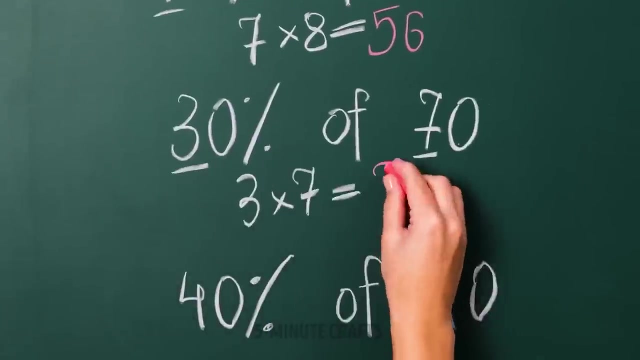 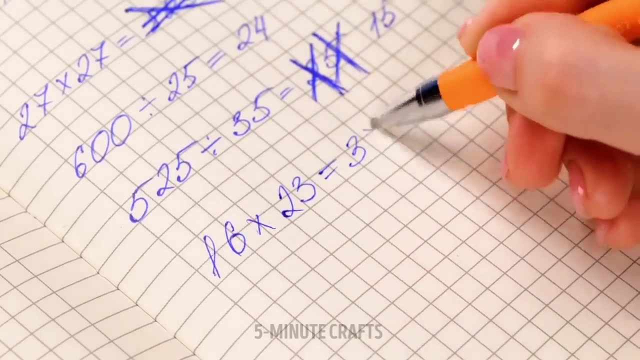 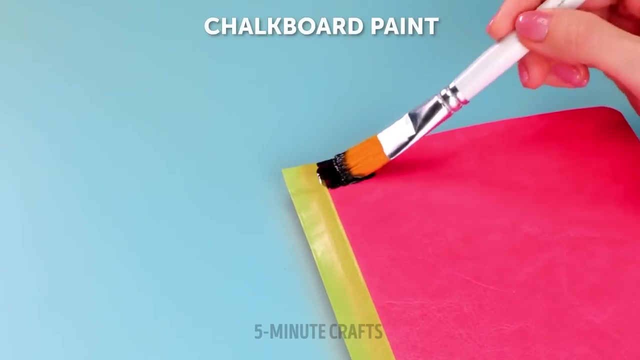 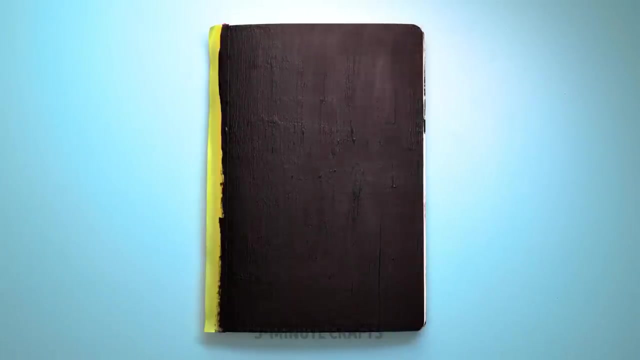 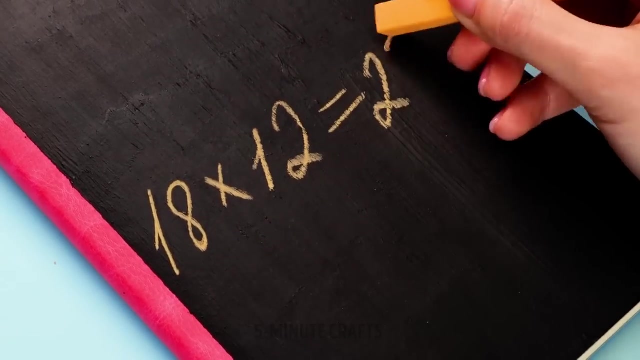 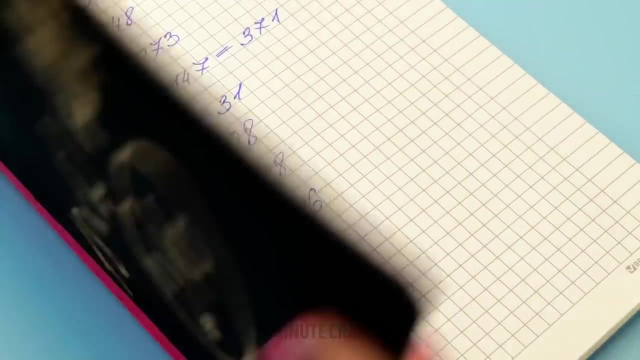 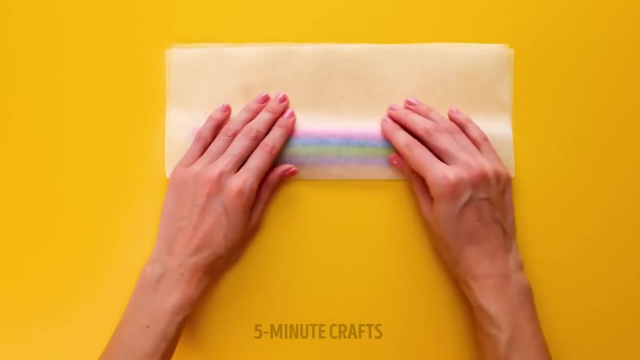 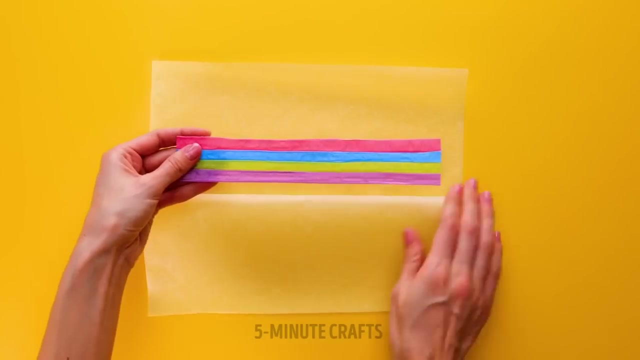 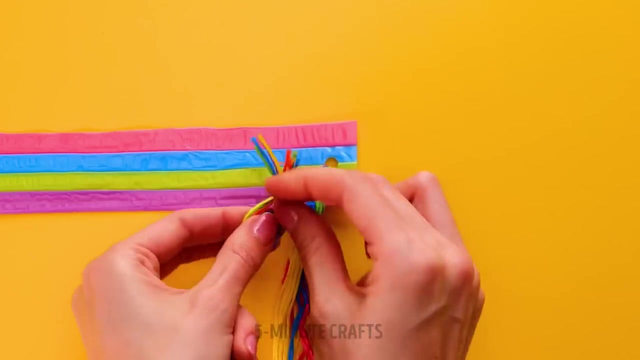 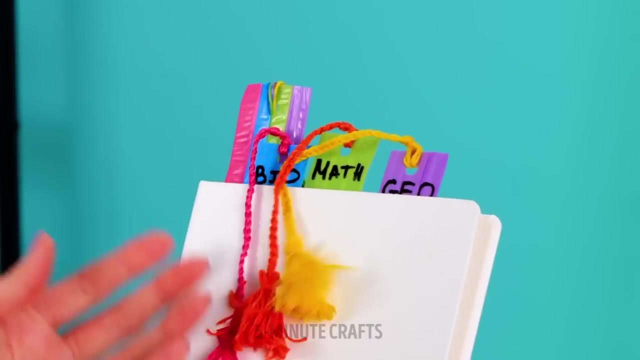 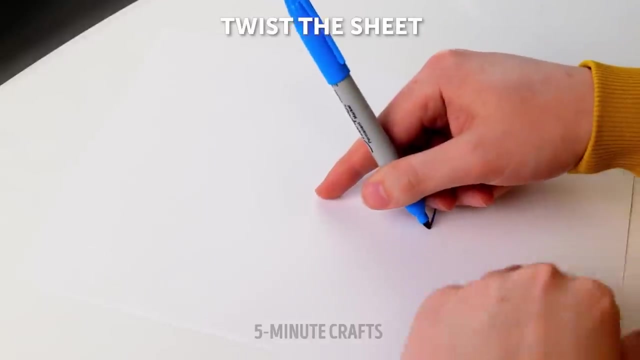 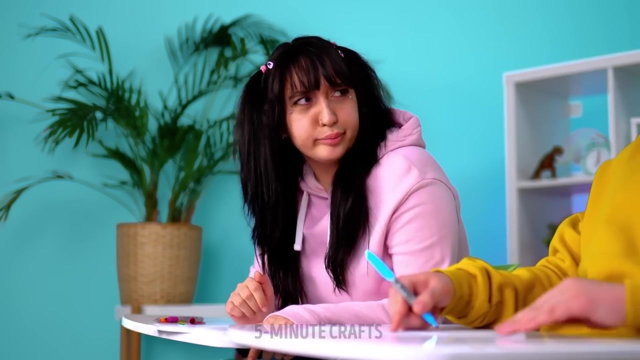 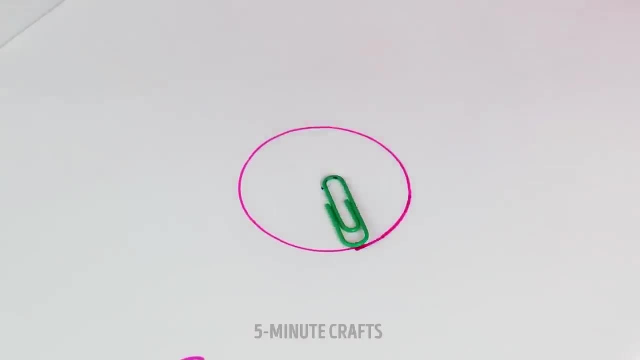 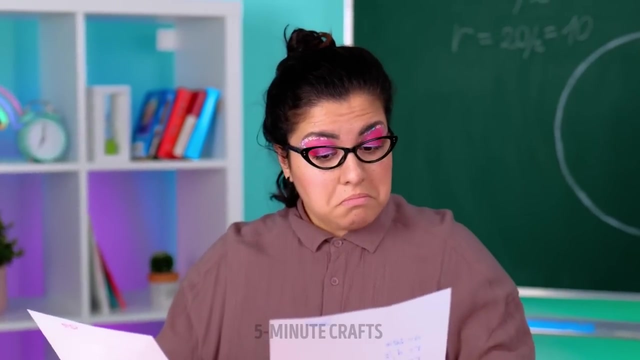 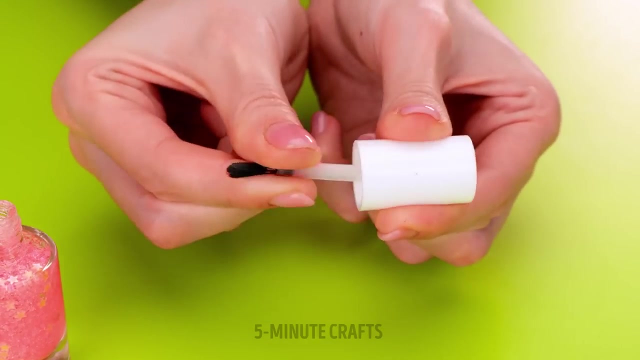 I just want to shout: Don't make me dance to the tune that you're humming. No, my body don't move like that. Don't make me pretend I don't see a Sean Cummings. You'll be running when I raise a black flag. 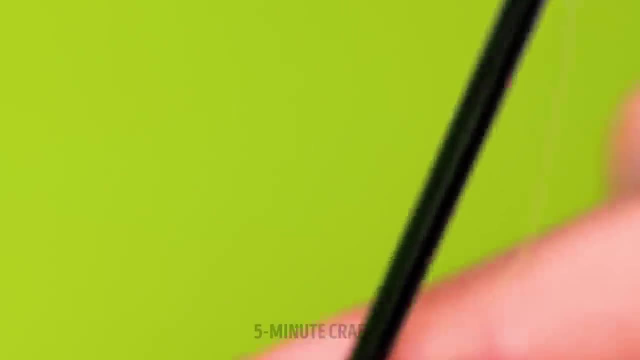 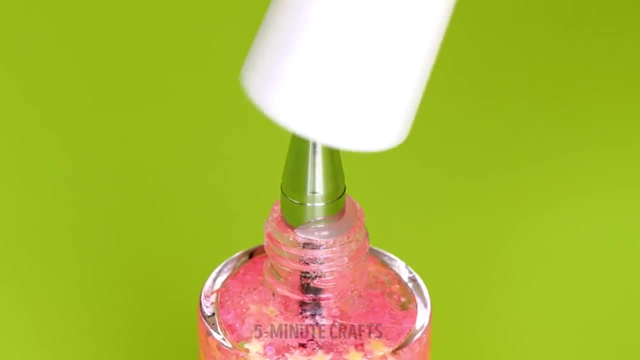 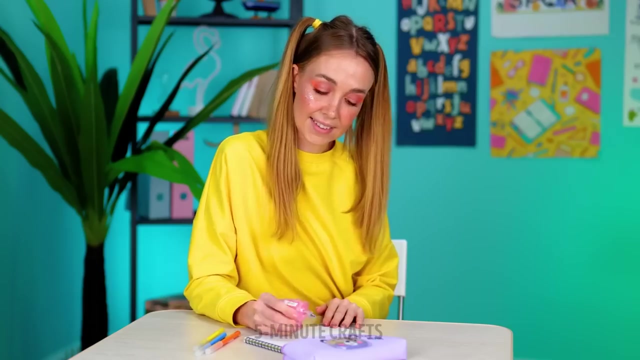 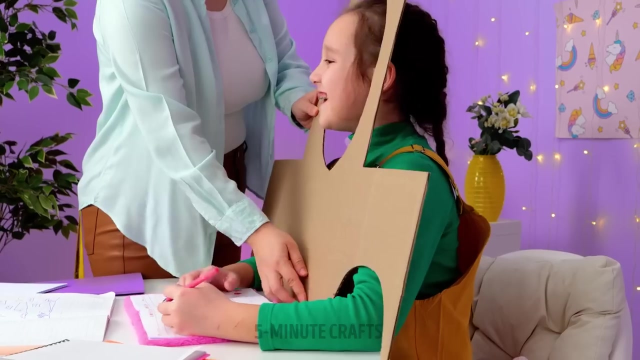 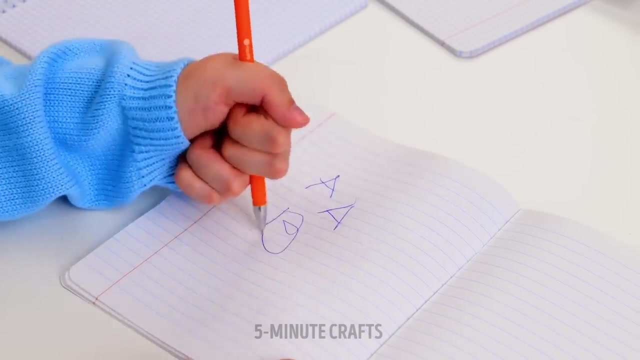 Get out your bomb and fly away. We'll be dancing with our heads in the air When our new dawn is rising To the break of dawn. You can't keep me in a cage made of tired ideas. It's rusting out faster by the day. 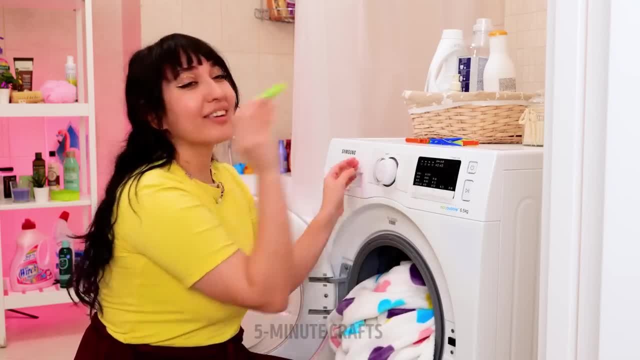 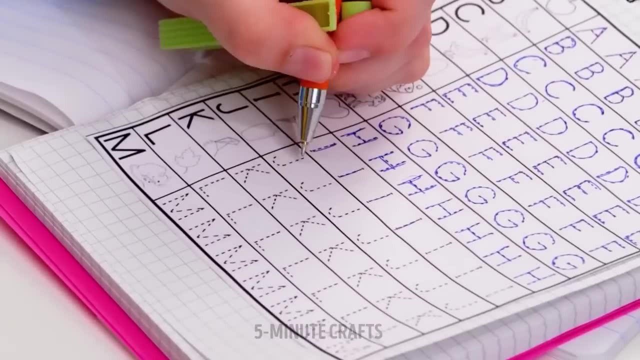 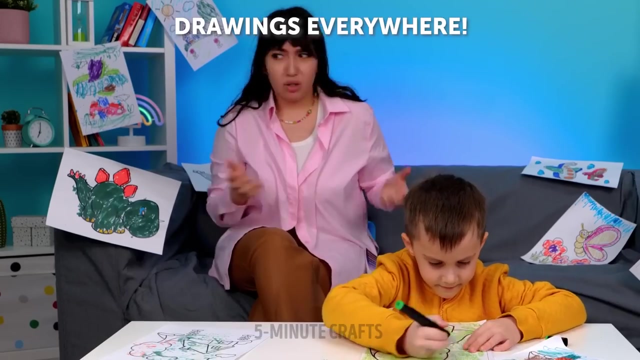 I don't want to wear your leash, I don't take no deals. I won't stay quiet when there's so much left to say I'm not buying the rise of suburban life, When there's a fire raging just outside our door. 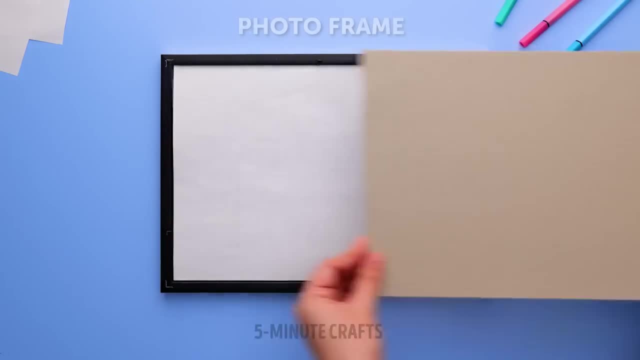 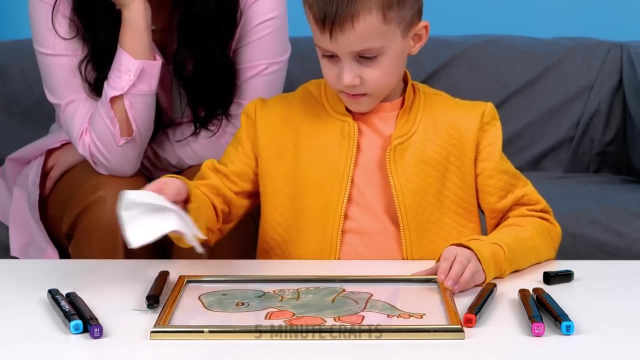 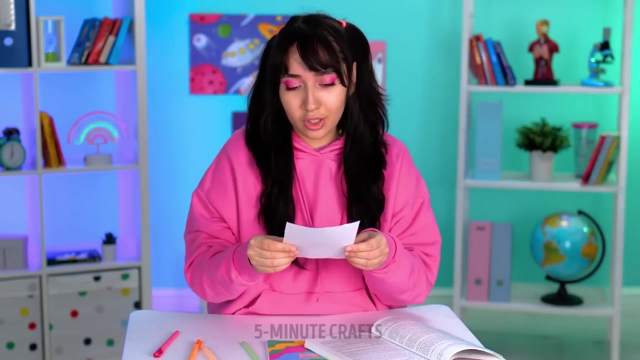 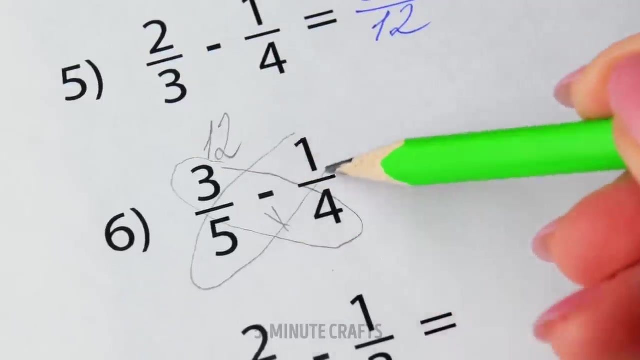 You talk about peace so much, Then the summer of life. Why are you sleeping on pills through the war? Get out your bomb and fly away. We'll be dancing with our heads in the air When our new dawn is rising. We'll be dancing with our heads in the air. 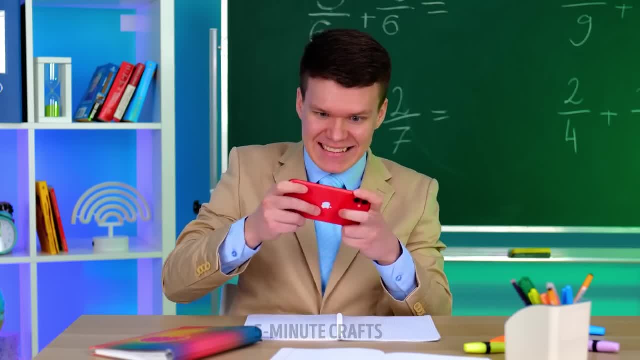 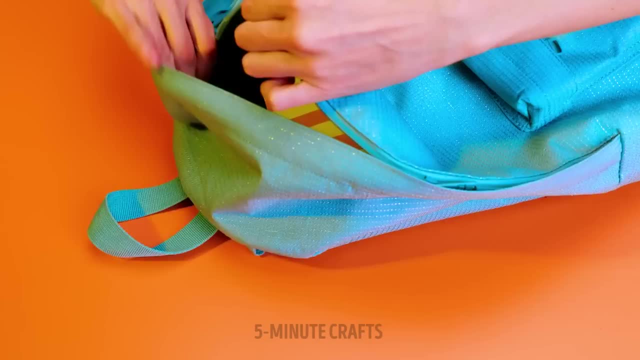 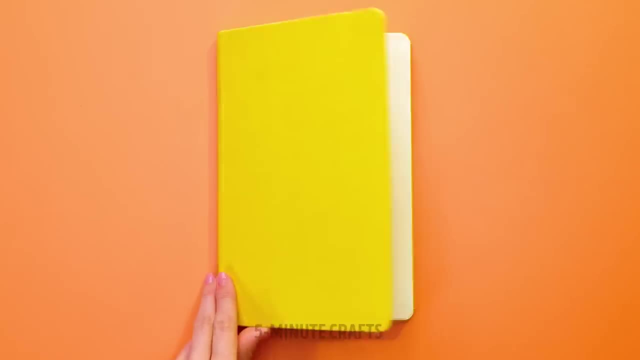 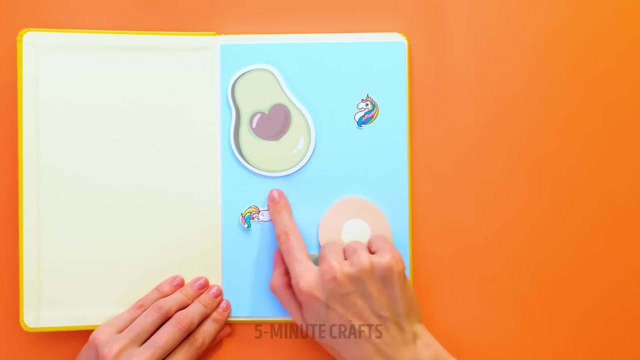 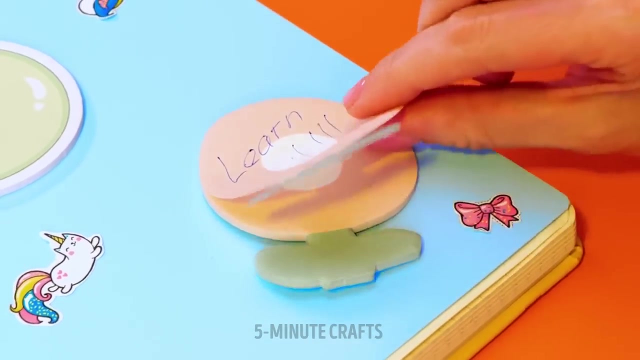 When our new dawn is rising, We'll be dancing. We'll be dancing. We'll be dancing To the break of dawn. When our new dawn is rising, We'll be dancing with our heads in the air. When our new dawn is rising. 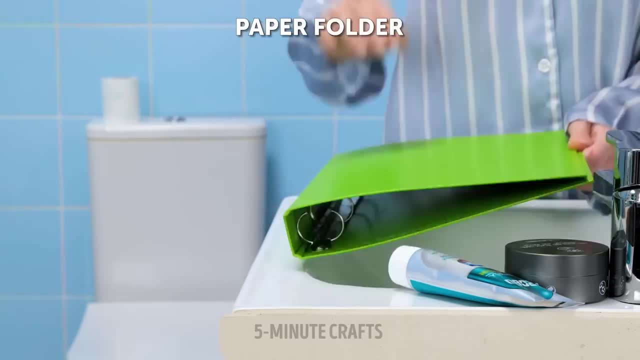 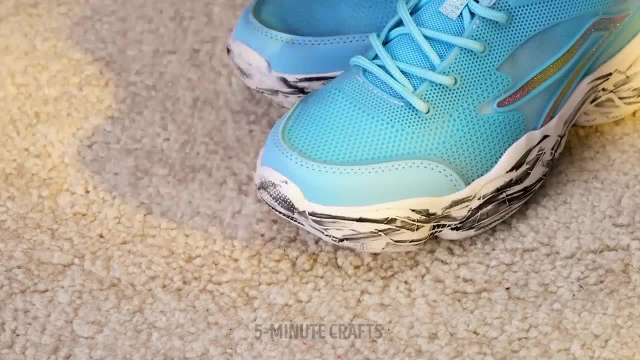 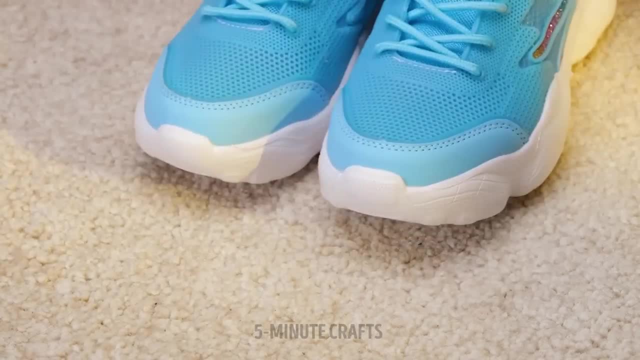 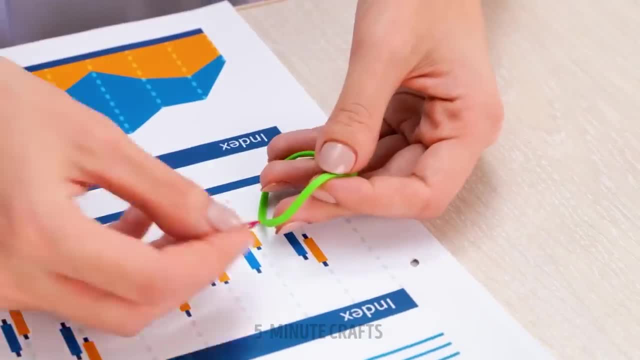 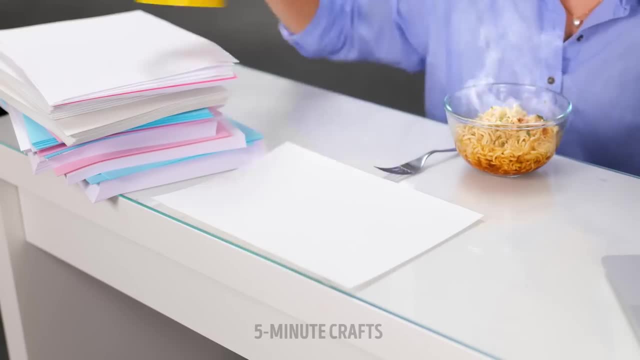 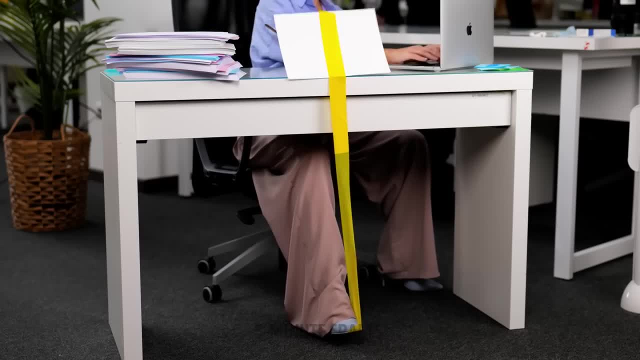 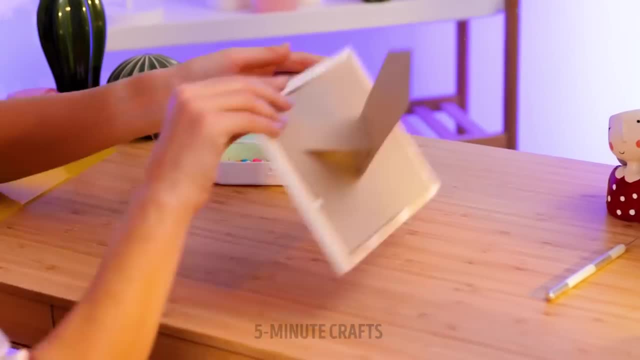 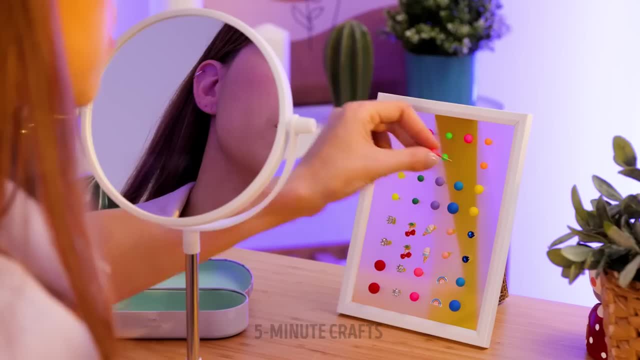 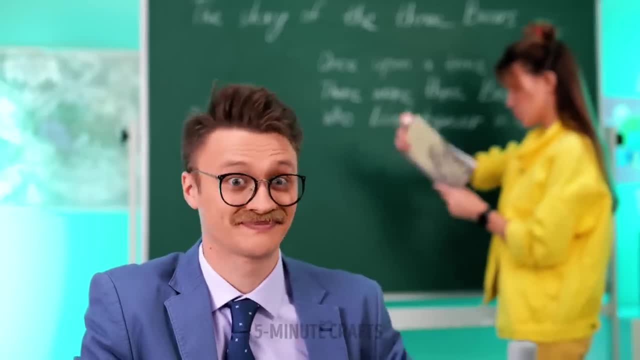 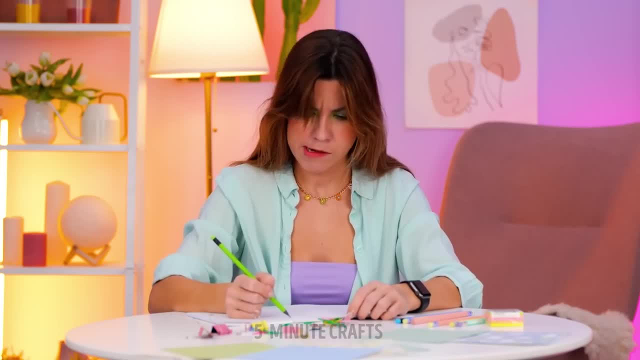 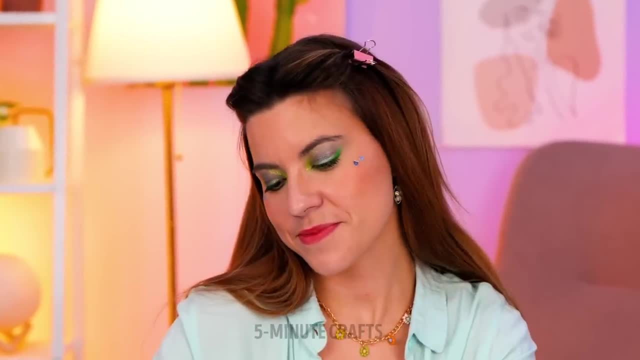 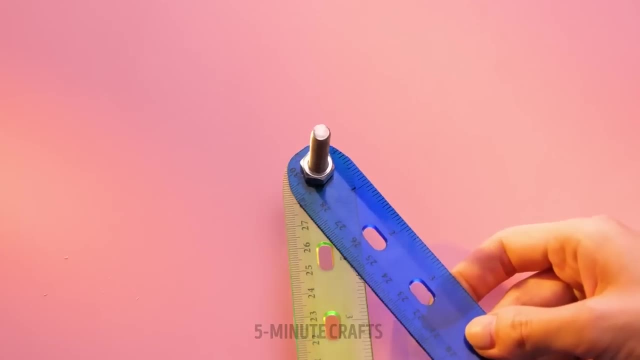 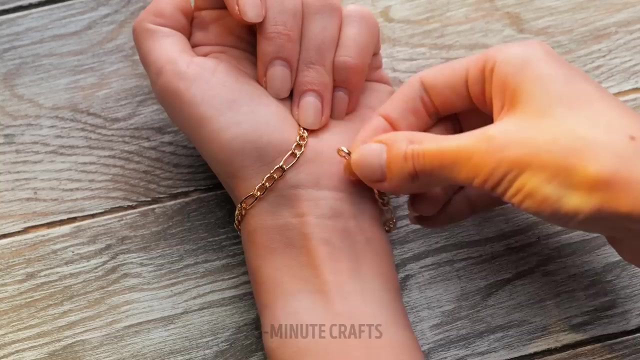 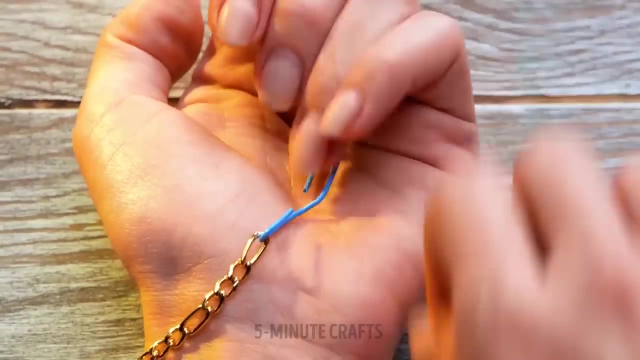 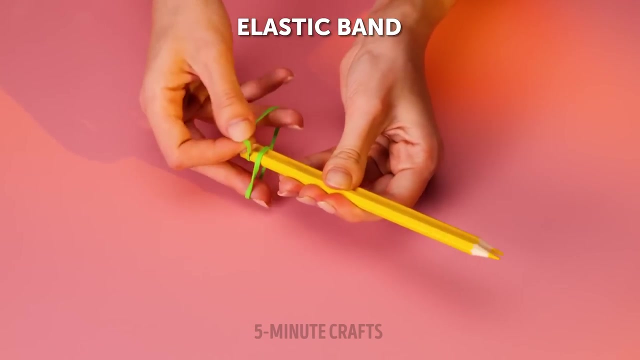 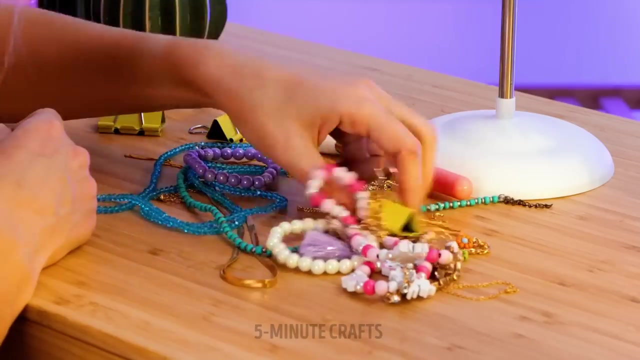 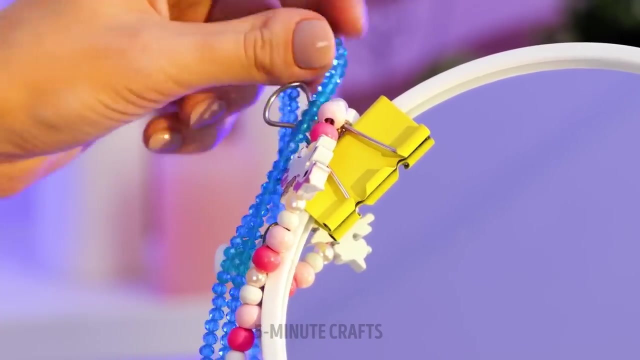 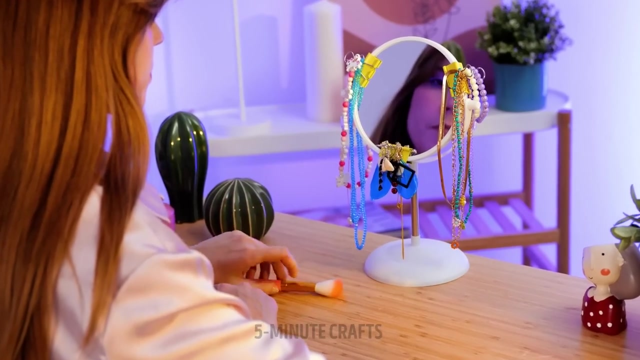 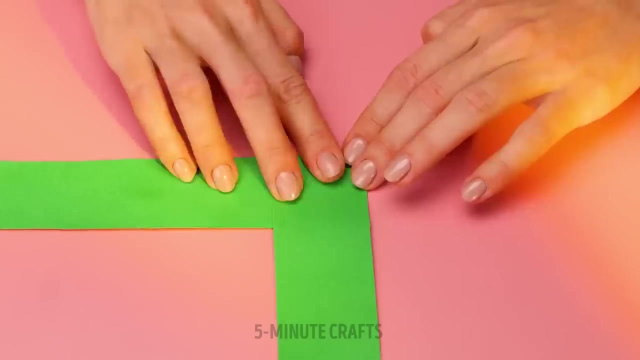 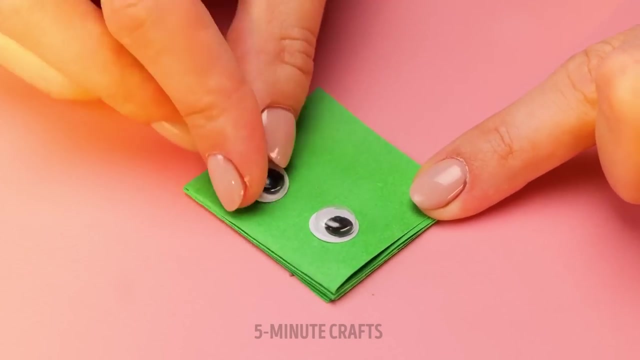 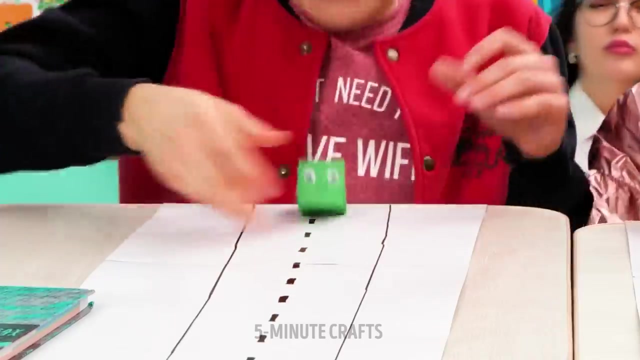 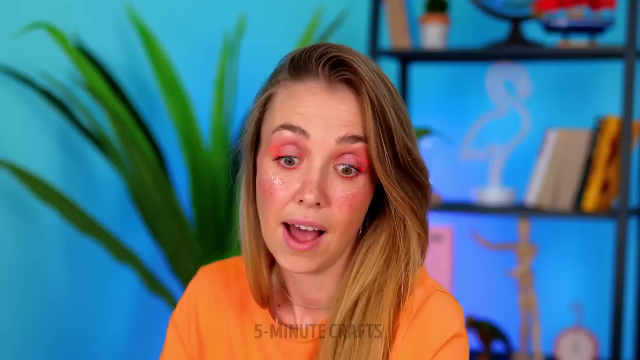 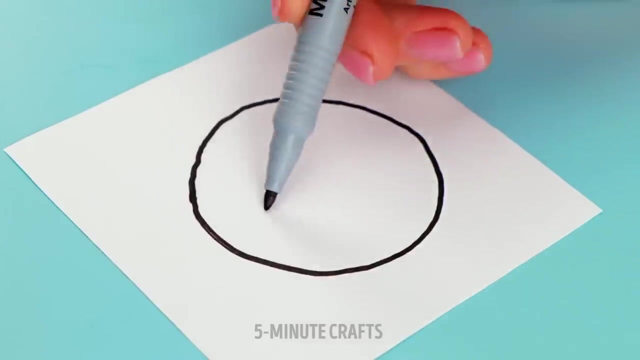 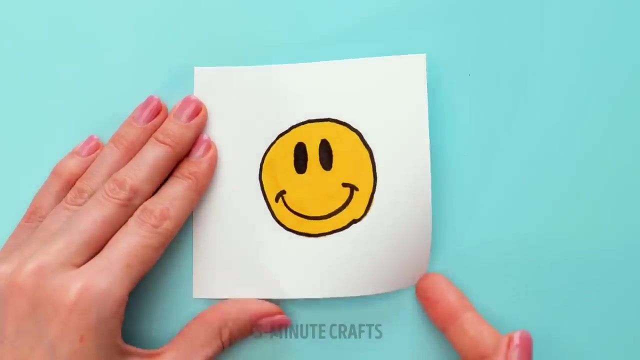 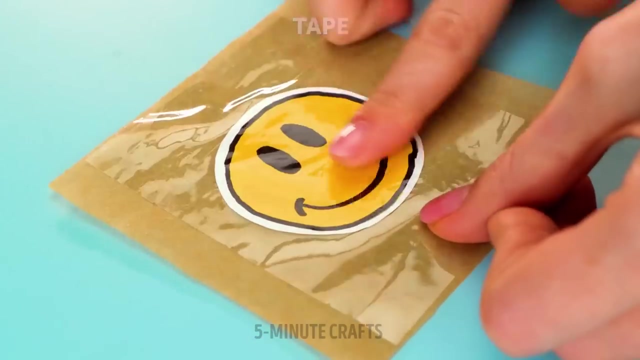 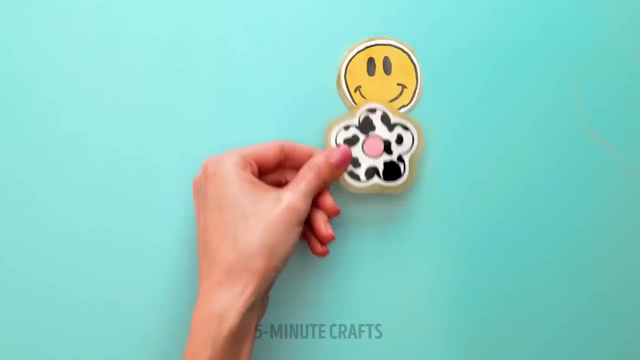 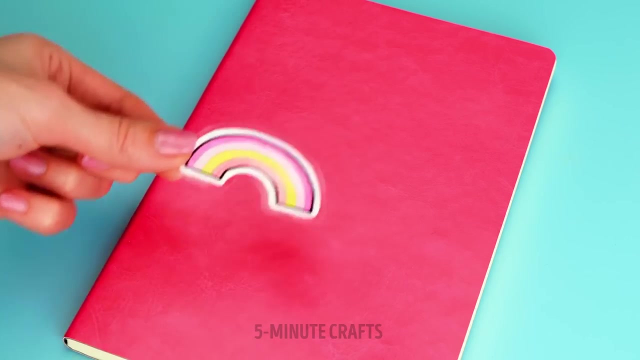 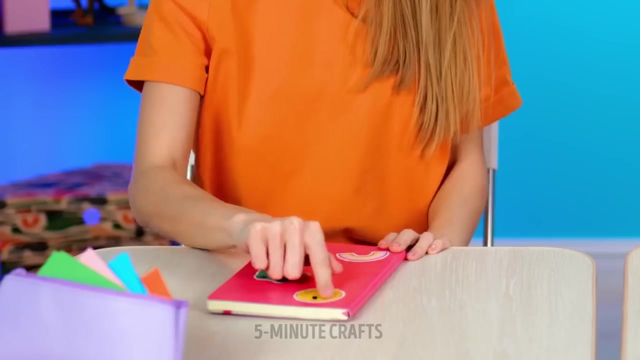 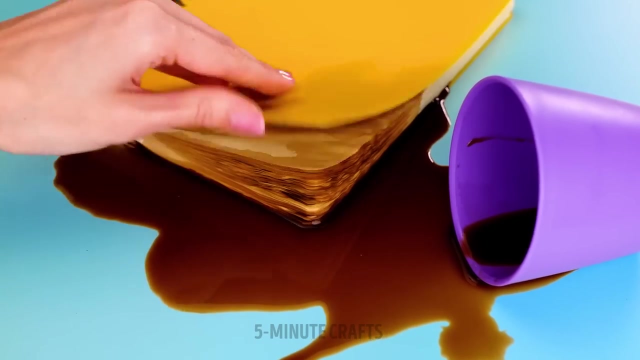 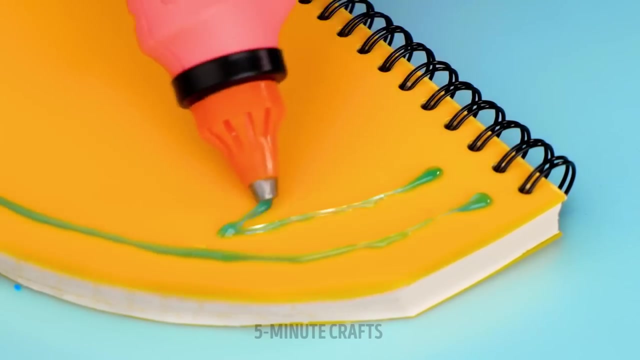 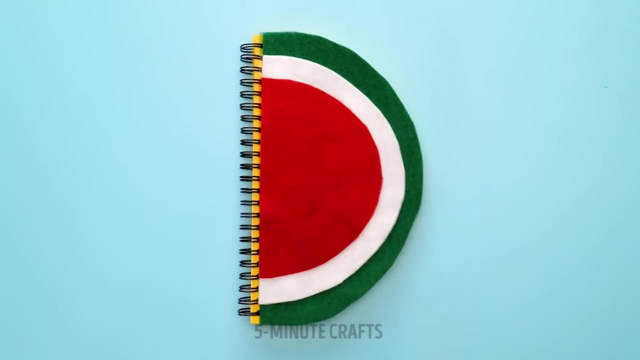 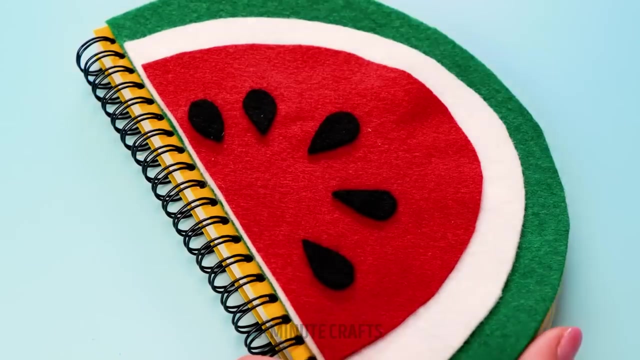 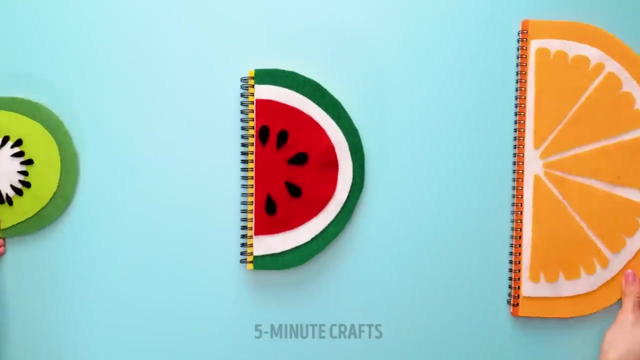 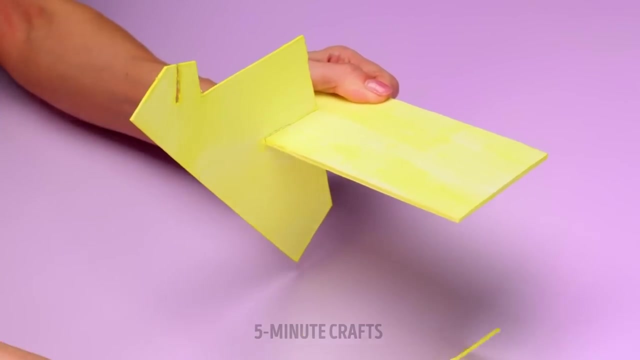 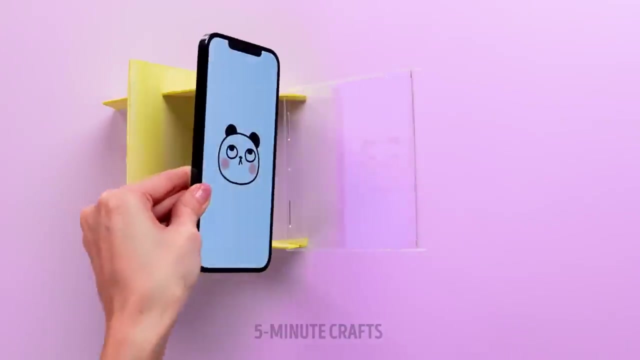 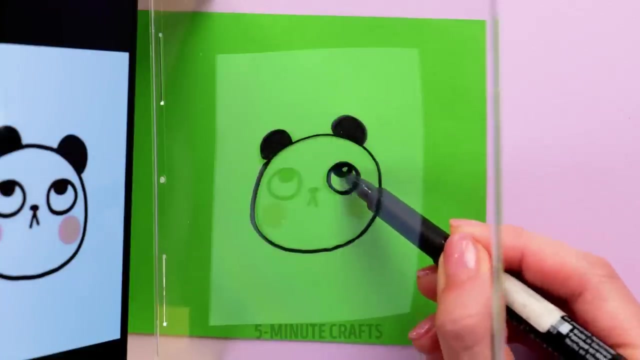 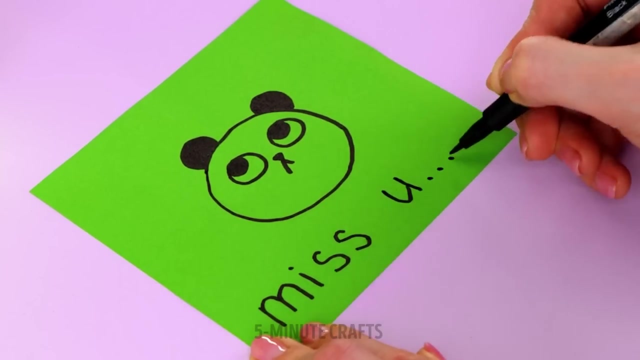 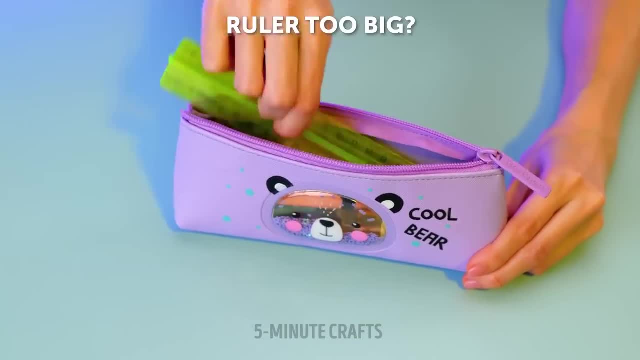 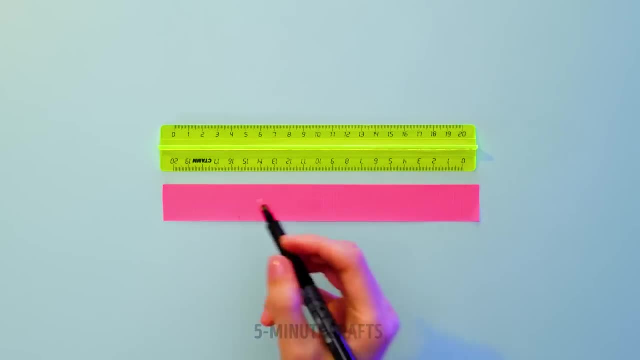 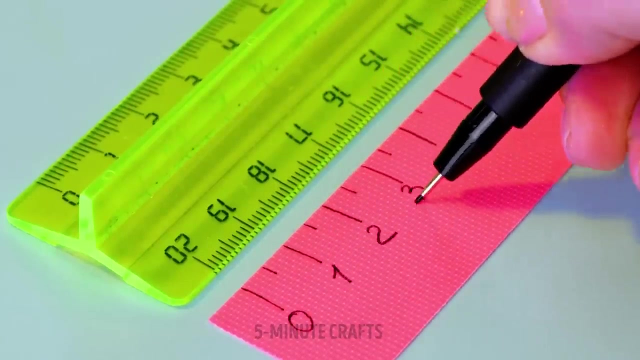 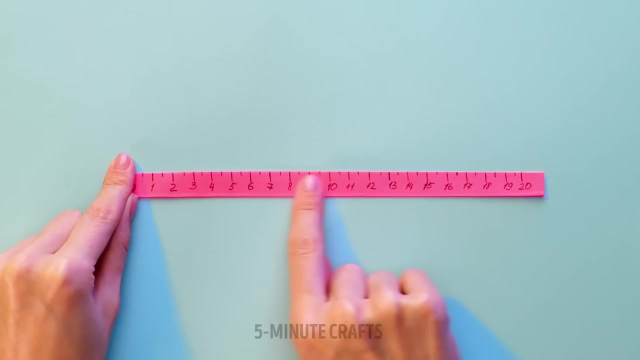 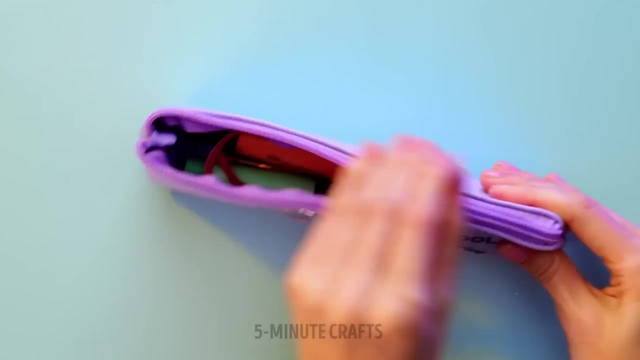 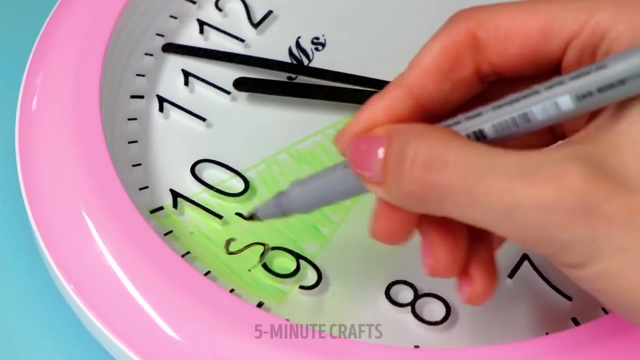 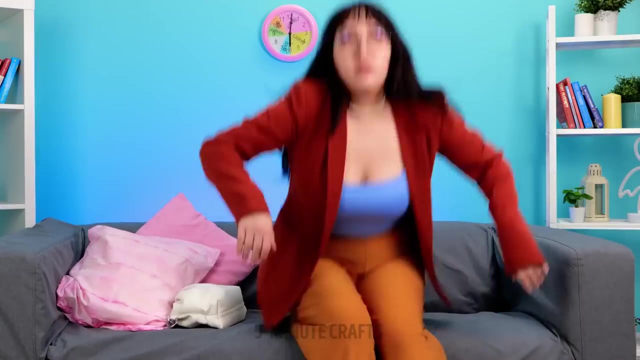 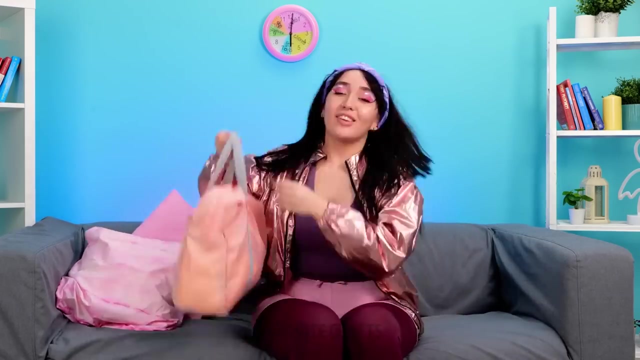 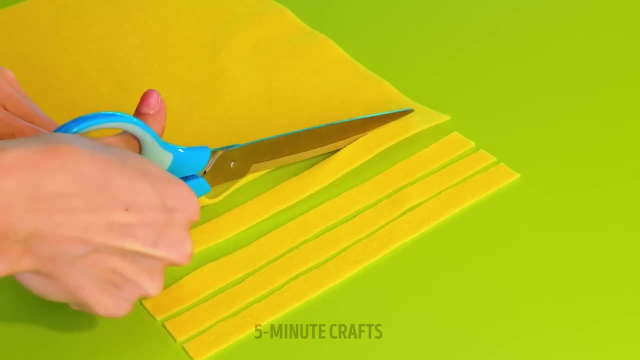 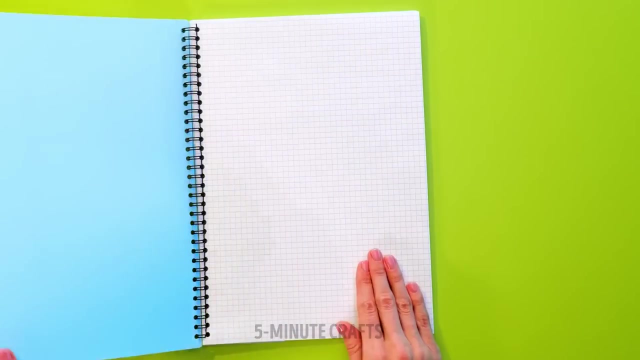 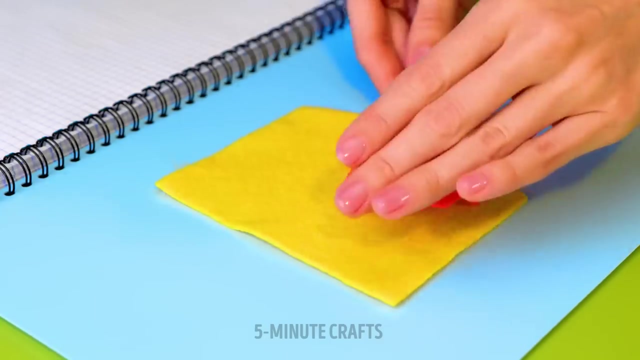 And me, baby. I've been waiting for a lifetime. Just keep on fading in all these photos Caught in the memories and captured in the highlights. Just keep on wasting Glass after glass. I keep hoping you'll come around, Drowning, I fight to win. 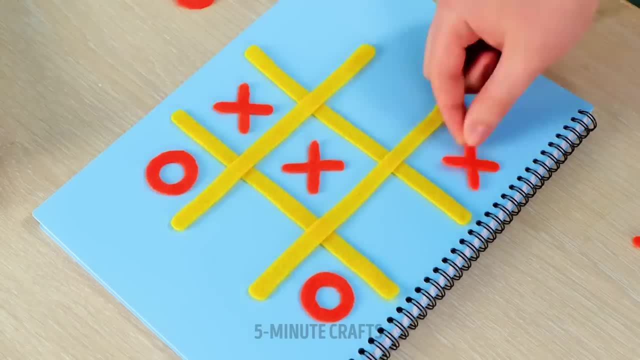 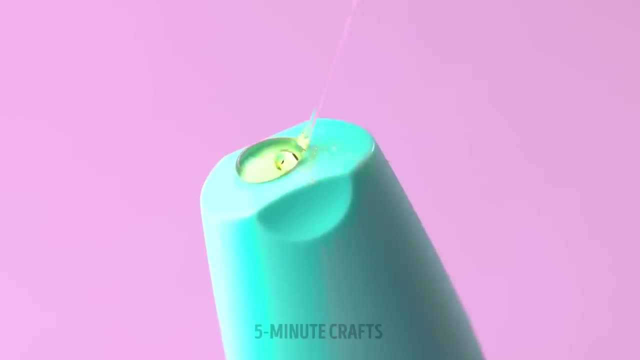 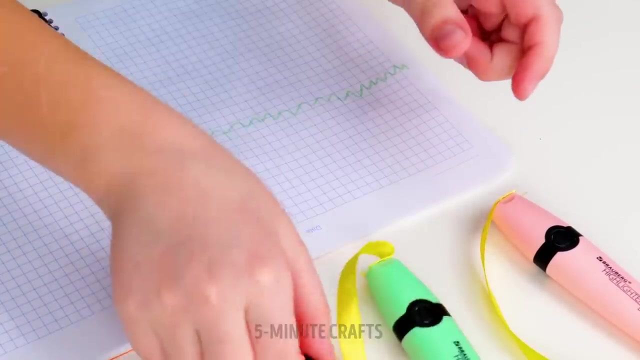 Whatever can be found, Cause I've given in to all my demons lately. You know I'm not alone. Might be easier just to let it go, Cause the cable's short and the problem's solved. Might be easier For you. I'd do it all night. You're my only next life. 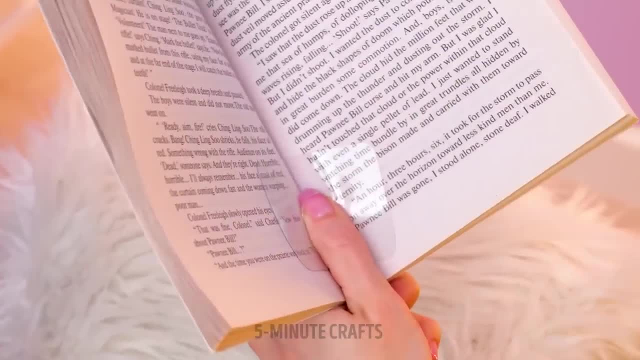 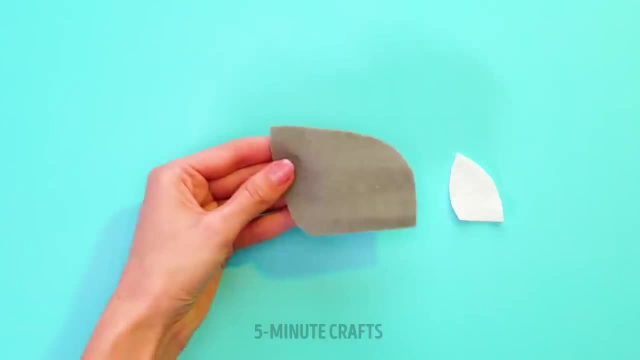 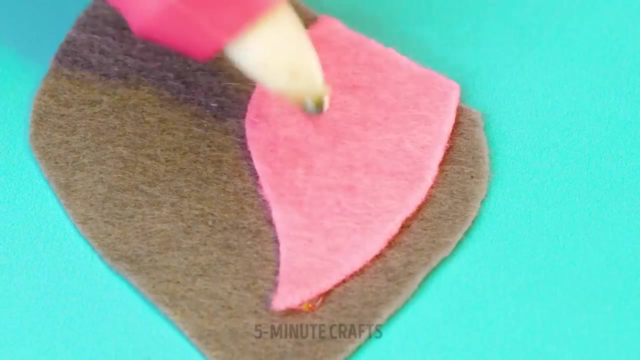 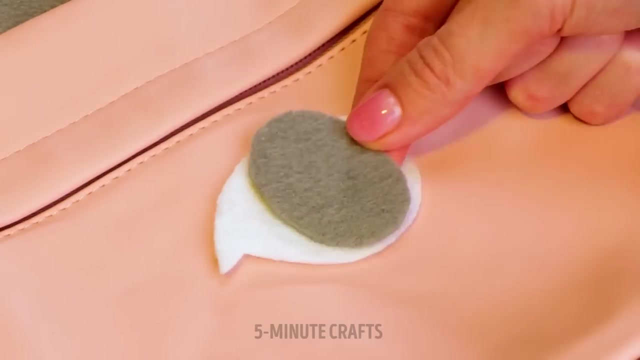 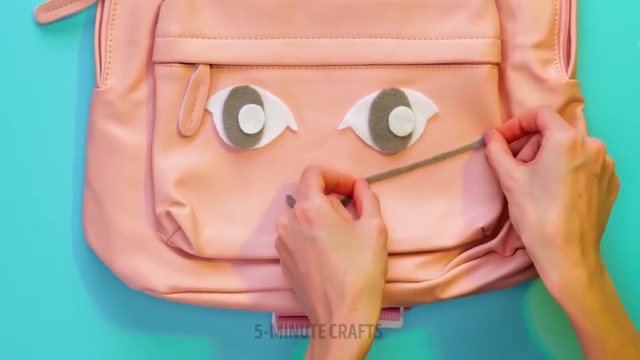 You're the only one I can count on. I'm saying for me, darling, it's been quiet for a day now. Can't bear the silence inside my own head. I can't bear the silence inside my own head. Keep on hoping somehow we can make this all right. 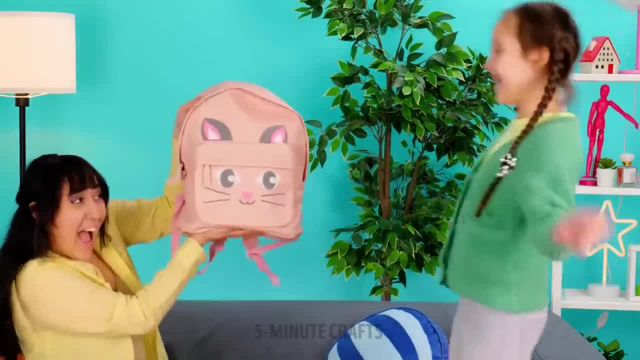 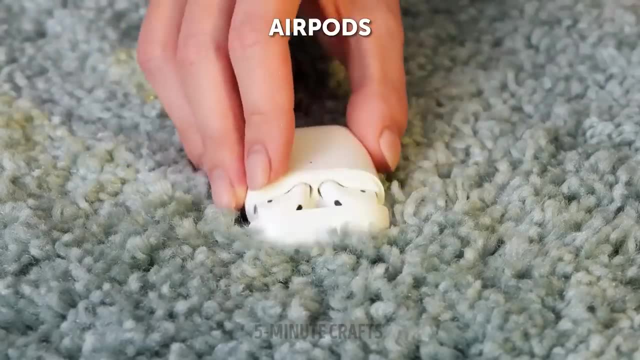 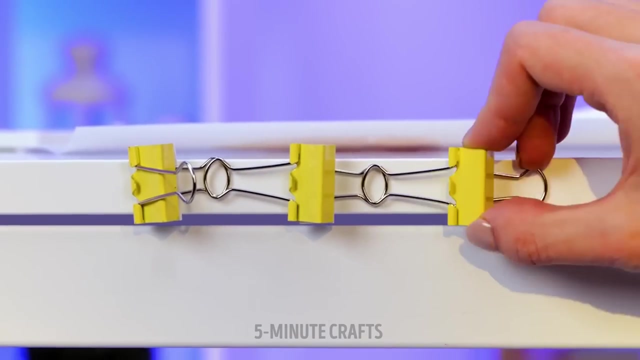 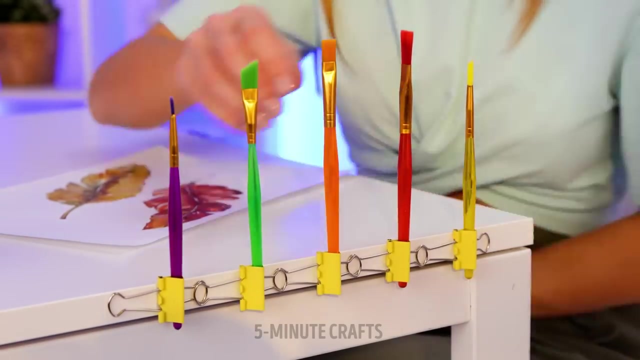 Just keep on trying Glass after glass. I keep hoping you'll come around Drowning. I'm fighting what, whatever can be found, Cause I've given in to all my demons lately. You know, Might be easier just to let it go. Cut the cables short and the problems solved. 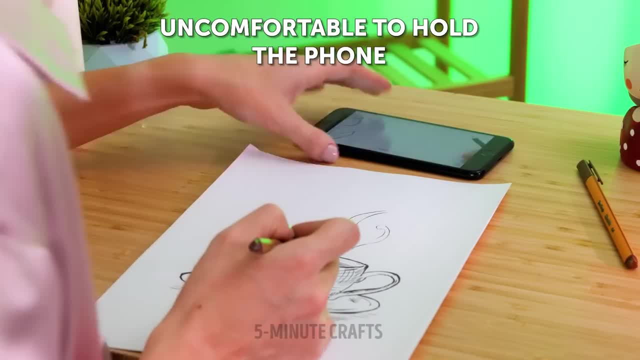 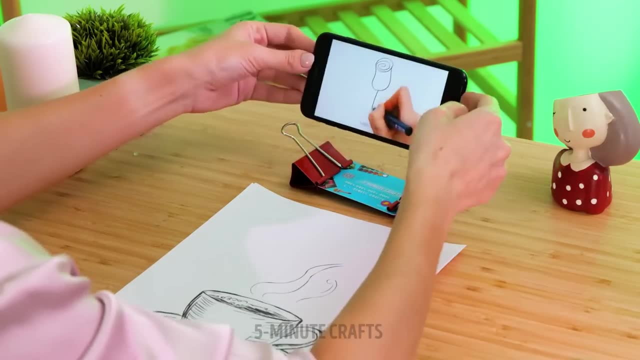 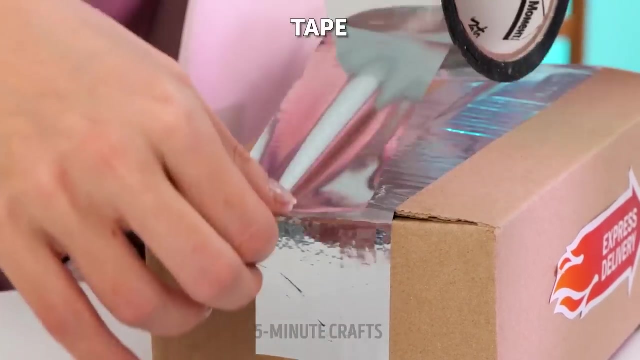 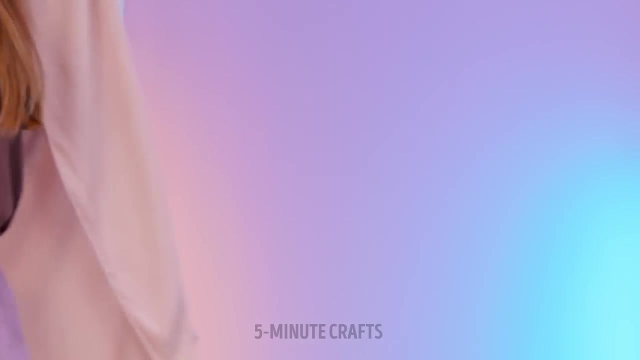 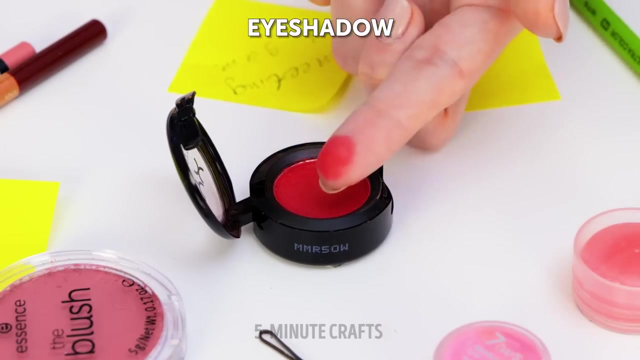 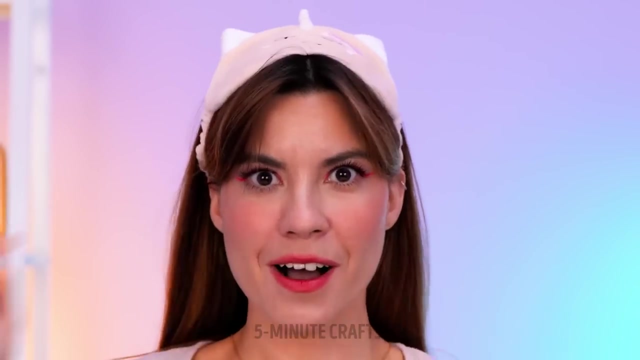 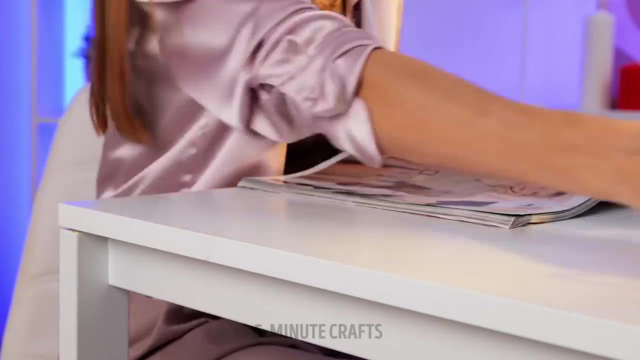 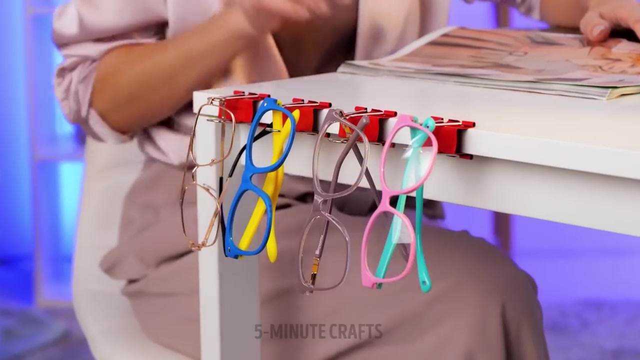 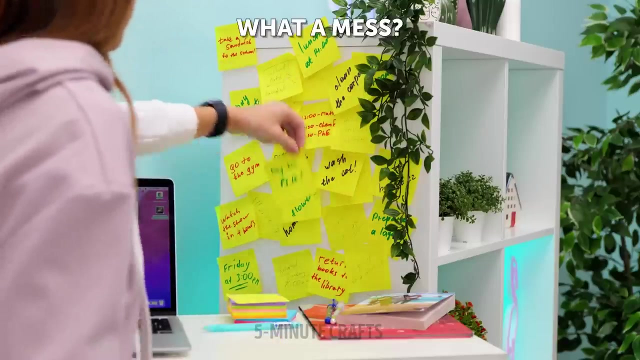 Might be easier For you. I'd do it all night. you're my only life. Talk to me, baby. I've been waiting for a lifetime. Just keep on fading in all these photos Caught in the memories and captured in the highlights. Just keep on wasting. Might be easier, just to let it go. 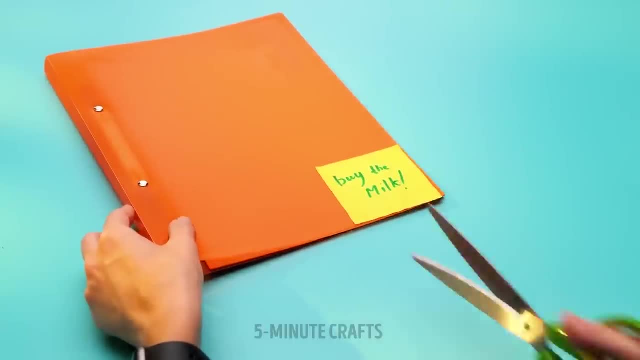 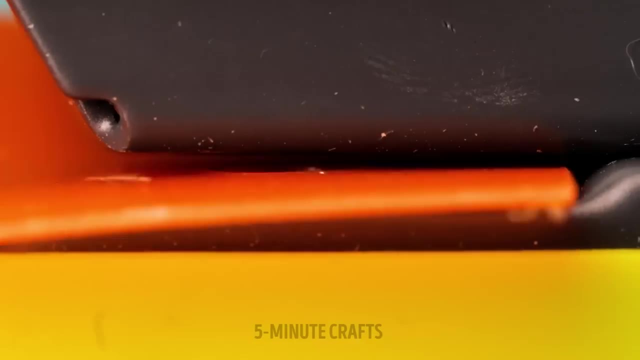 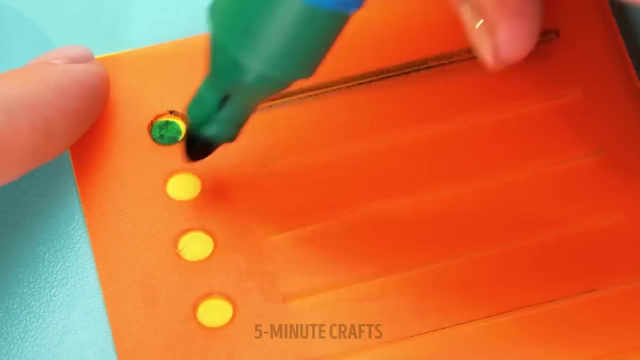 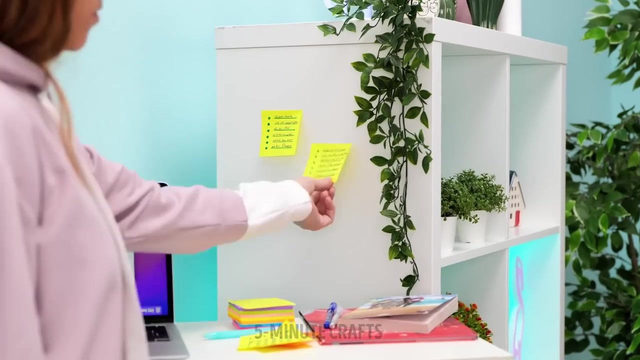 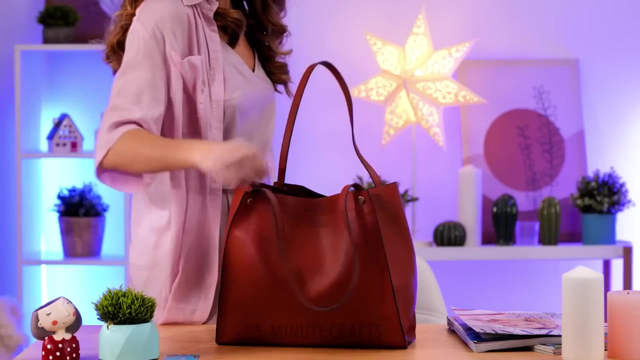 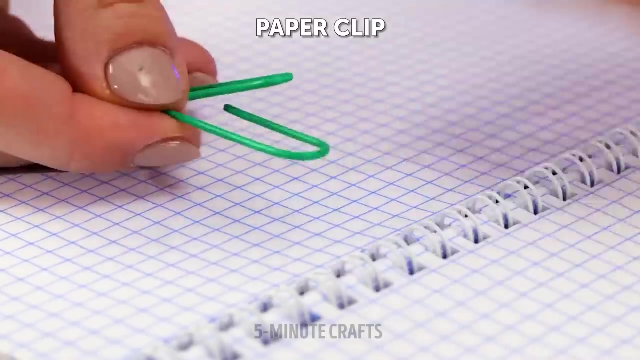 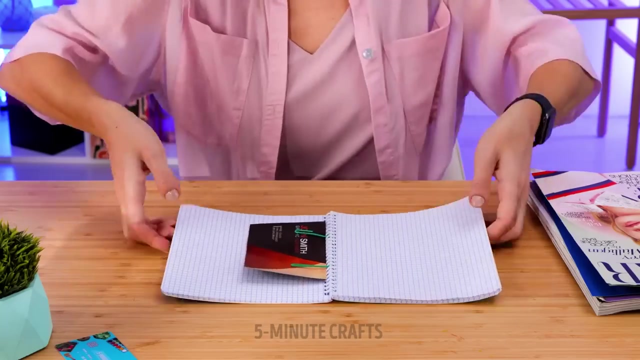 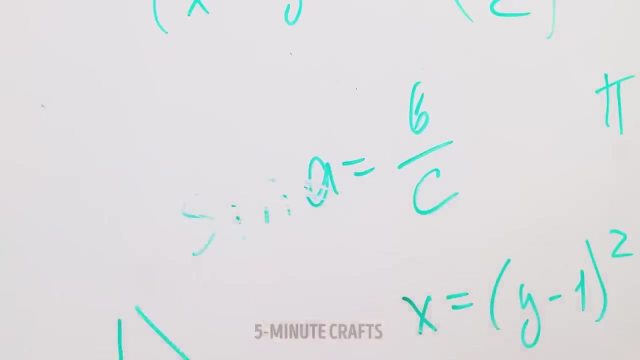 Cut the cables short and the problems solved. Might be easier For you. I'd do it all night. you're my only life. Cut the cables short and the problems solved. I get so caught up in the middle, Thinking of drowning in his blue eyes. I'm losing sight of what I see. 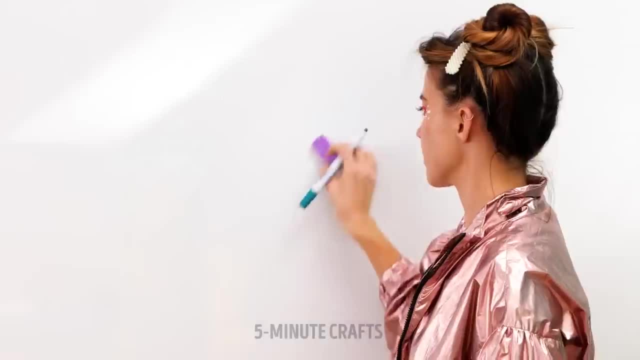 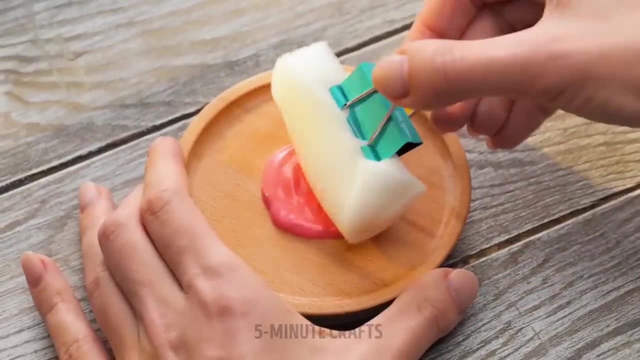 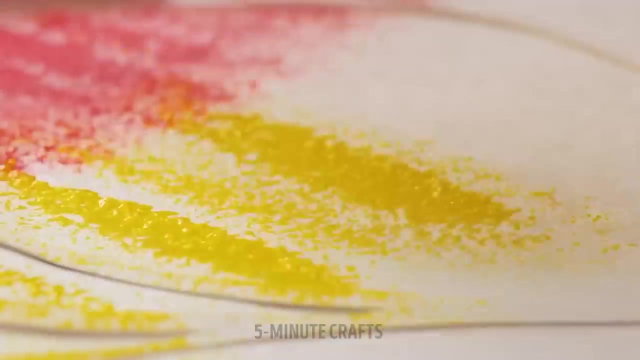 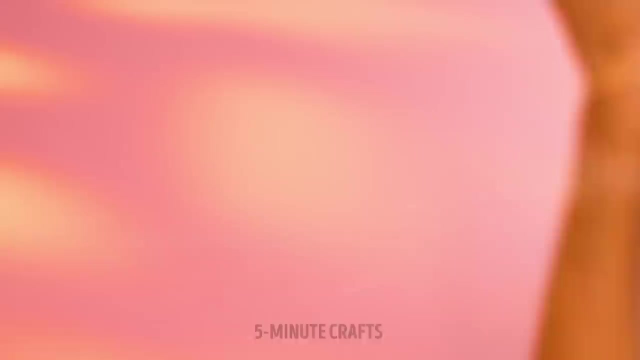 Cause I am falling. I'm so deep down, deep down, And it's not a lie That I die. I can't hide, Hide, oh, What this is, Oh, oh Yeah. I keep drowning in his blue eyes And you can tell me all of their lies. 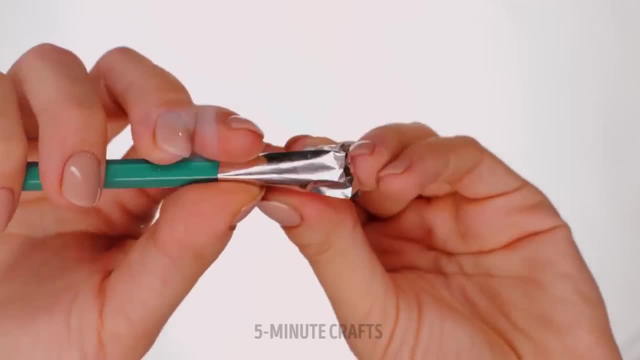 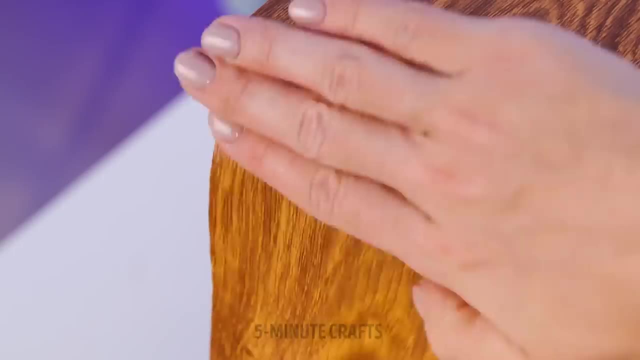 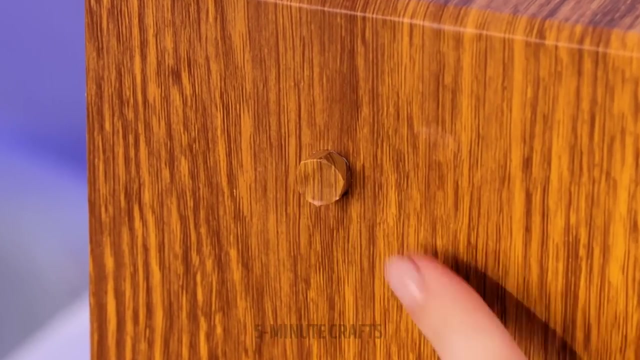 And you can tell me all of their lies. I will put out all of the fire If it gets too dark. Oh oh, I'll be your light. Ooh, ooh, Be your light. Ooh, ooh, I'll be your light. Ooh, ooh. 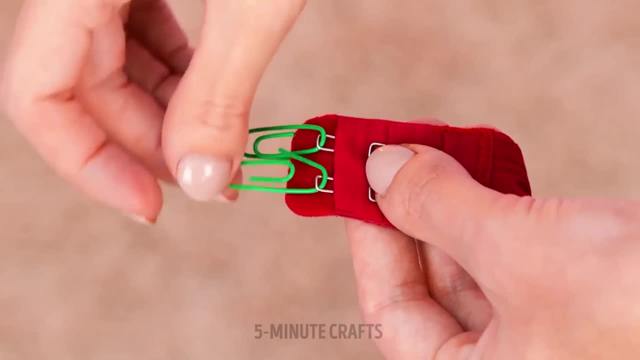 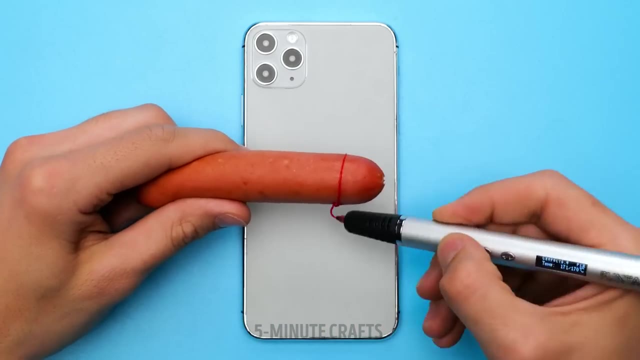 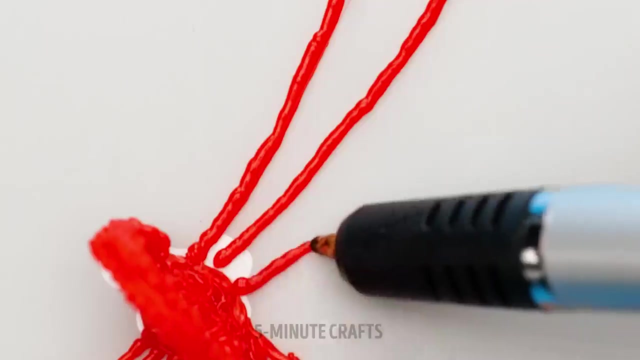 If it gets too dark, Oh, oh, I'll be your light. Be your light, Be your light, Ooh, ooh. If it gets too dark, Ooh, ooh. If it gets too dark, Oh, oh Yeah, I can carry all that you've got. 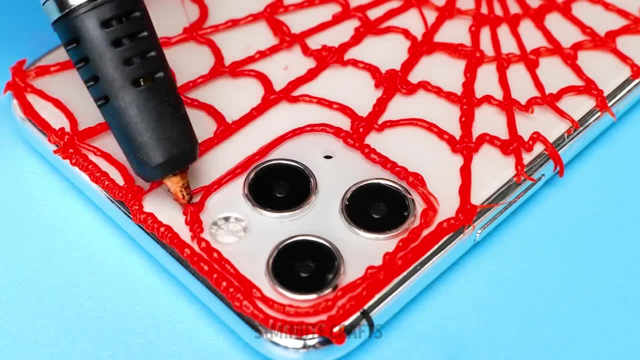 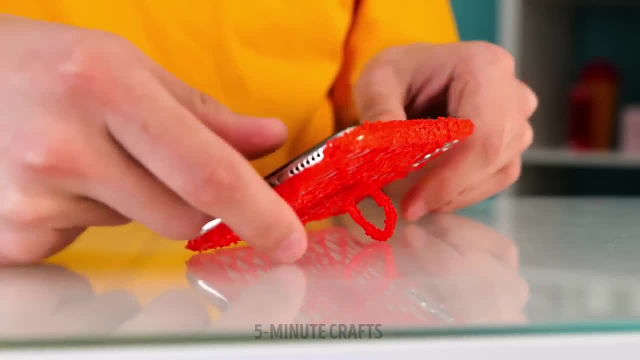 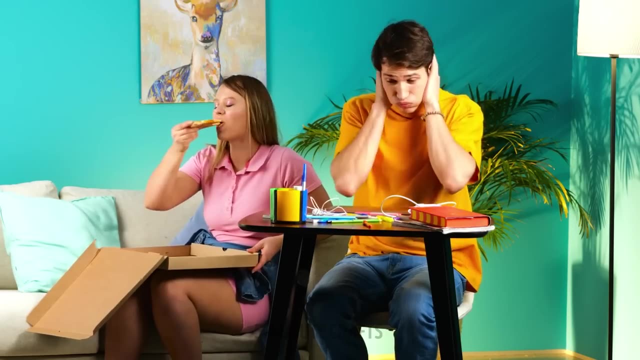 Too heavy hearts is not a lie. Too heavy hearts is not a lie. I will put out all of the fire. I will put out all of the fire. We stumble and fall, We stumble and fall, And it's not a lie, And it's not a lie That I die. 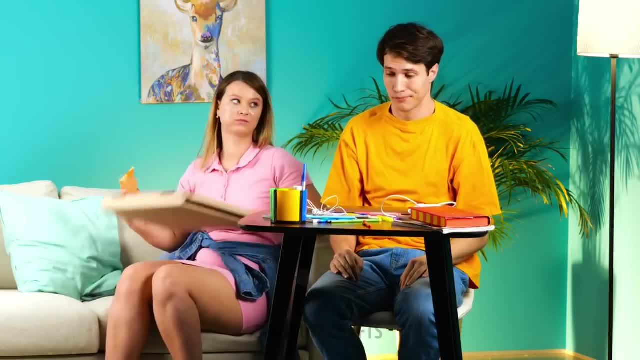 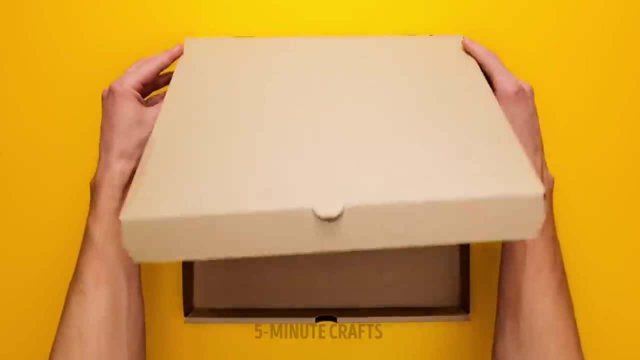 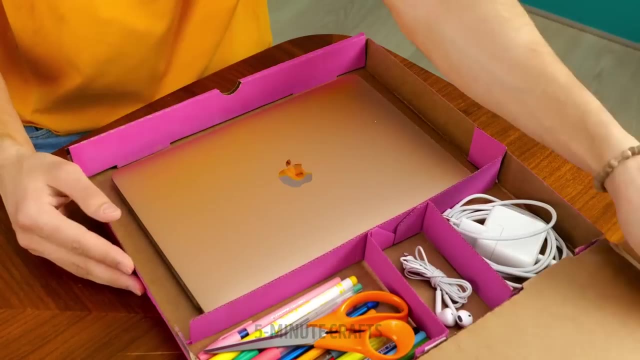 And it's not a lie That I die. I can't hide What this is, What this is. Oh, oh Yeah. I keep drowning in his blue eyes And you can tell me all of their lies. And you can tell me all of their lies. I will put out all of the fire. 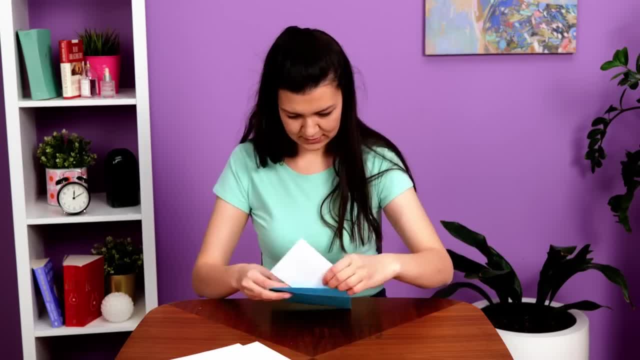 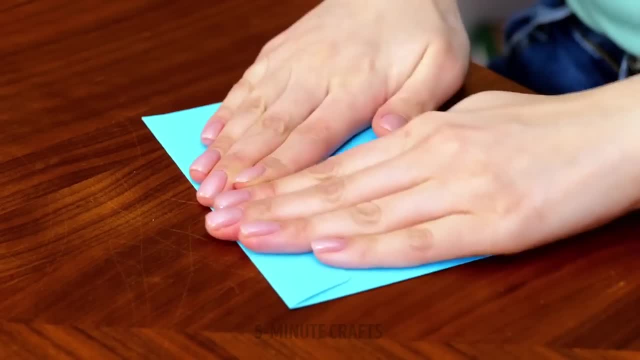 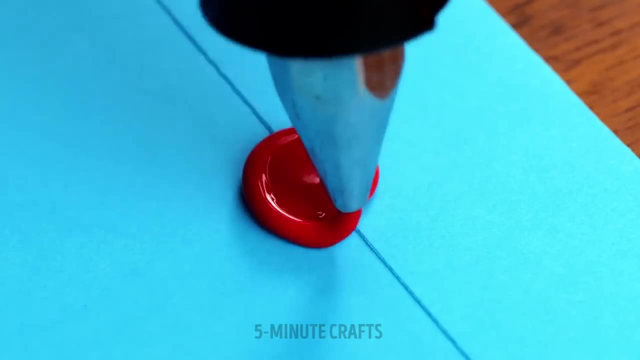 I will put out all of the fire If it gets too dark. Oh oh, I'll be your light. Oh oh, Be your light. Oh oh, I'll be your light, Oh oh. If it gets too dark, Oh oh, I'll be your light. 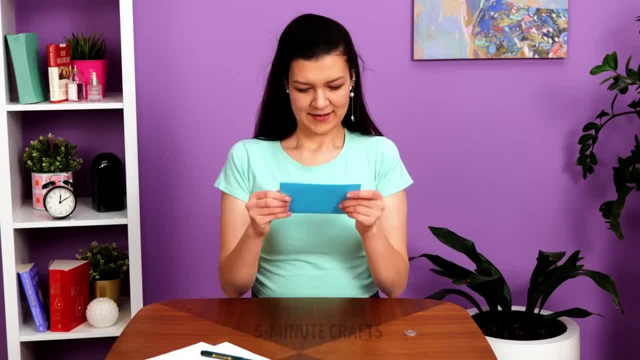 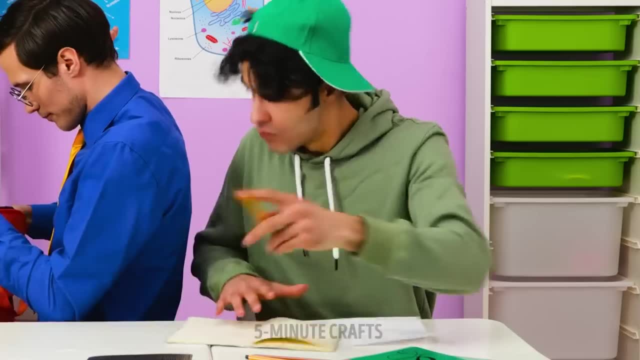 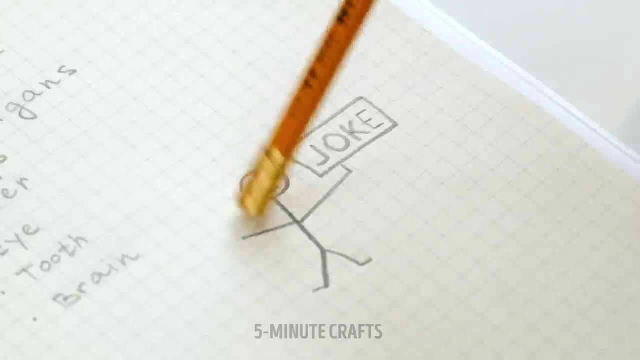 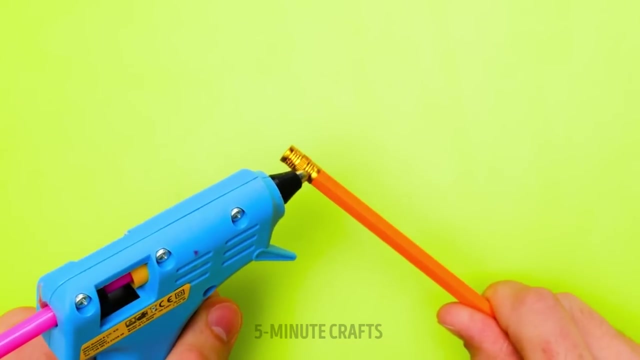 Oh, oh, Be your light. Oh, oh, I'll be your light. Oh, oh, If it gets too dark. Oh oh, I am running for you. Oh, oh, I am running for you. Oh, oh, I am running for you. Oh, oh, If it gets too dark. 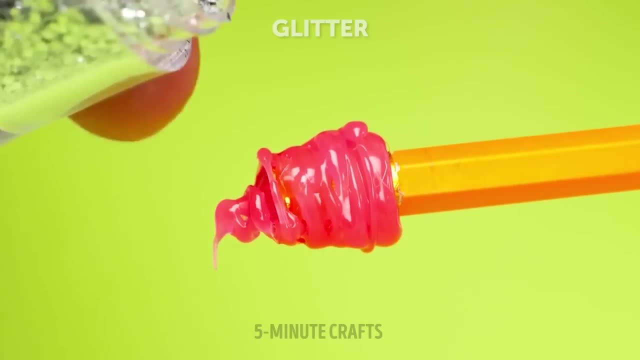 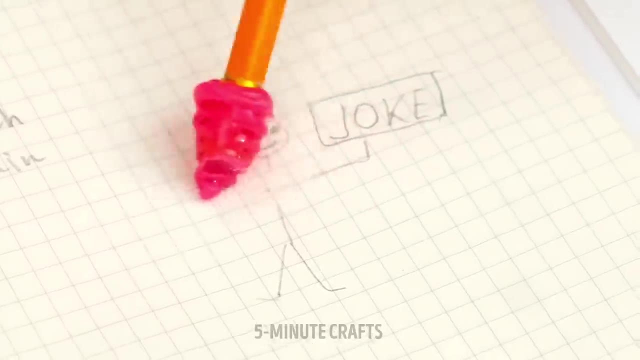 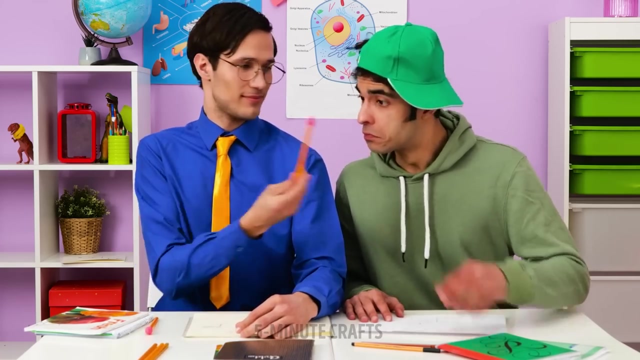 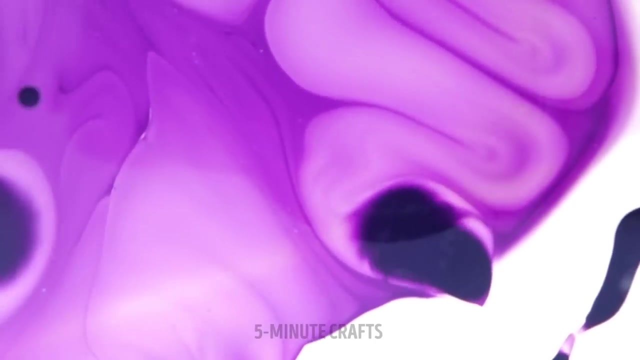 Oh, oh, Be your light. Oh, oh, I'll be your light. Oh, oh, Be your light. Oh oh, I'll be your light. Oh oh, If it gets too dark, Oh oh, I'll be your light. Oh, oh, I'll be your light. 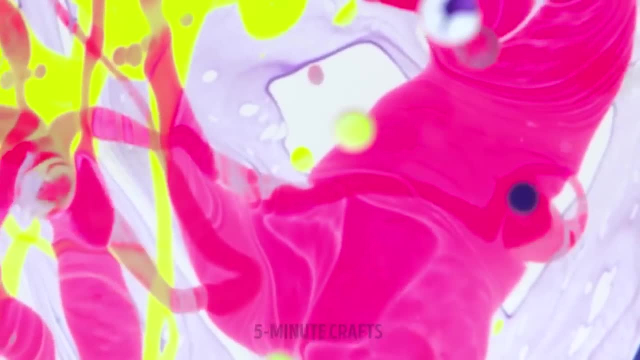 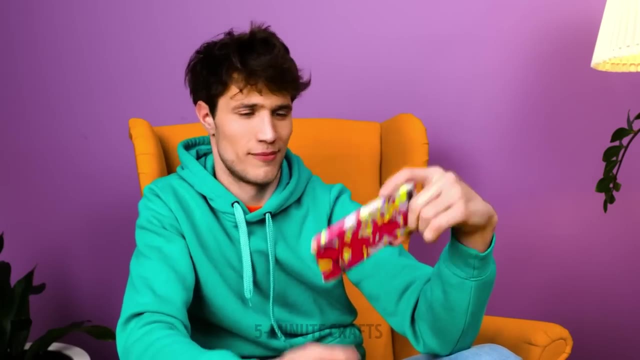 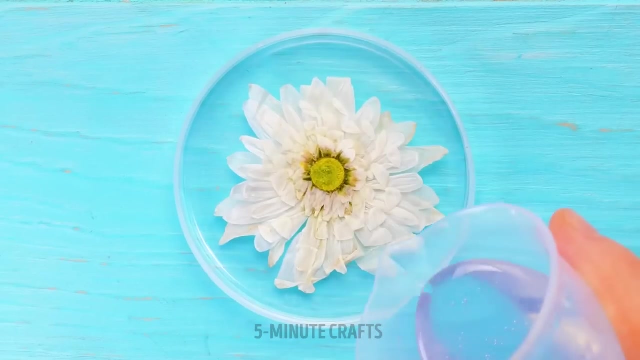 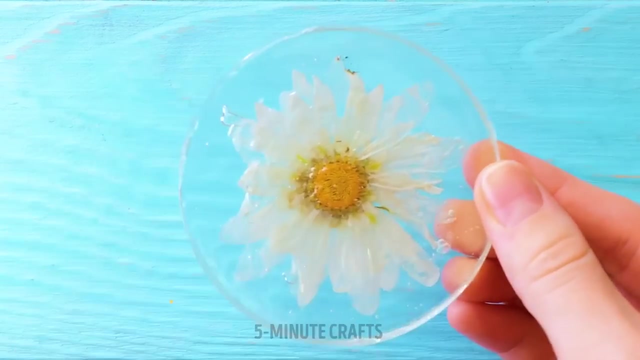 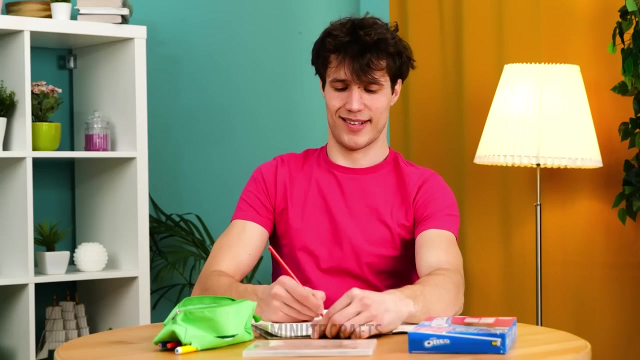 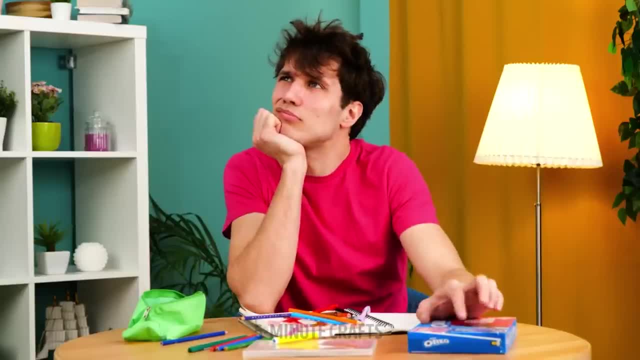 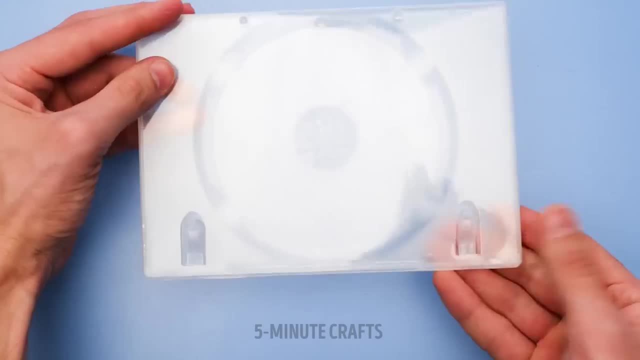 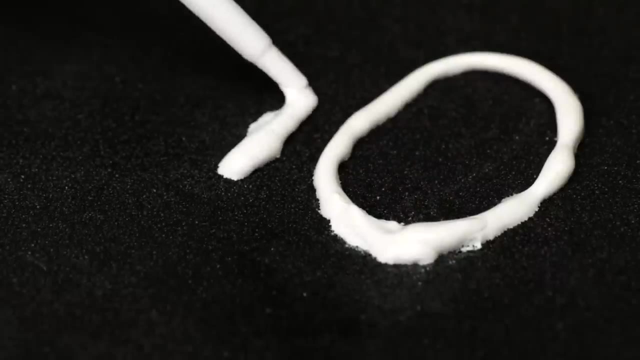 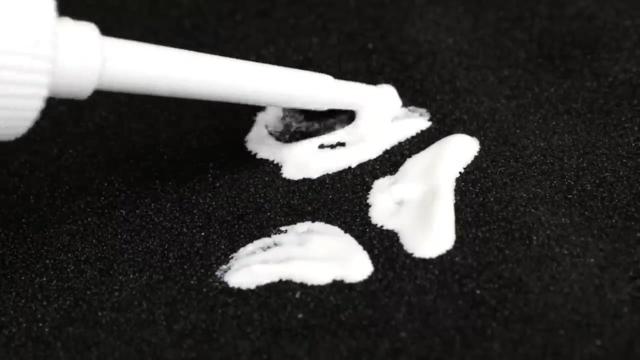 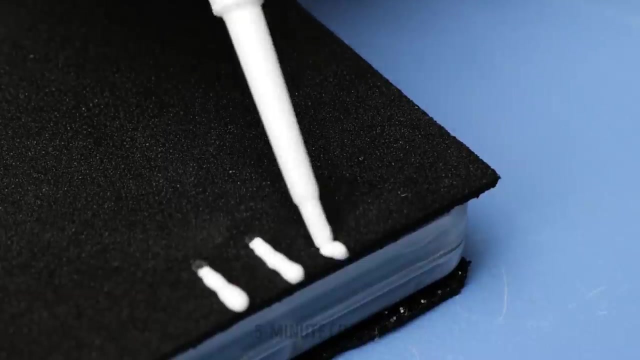 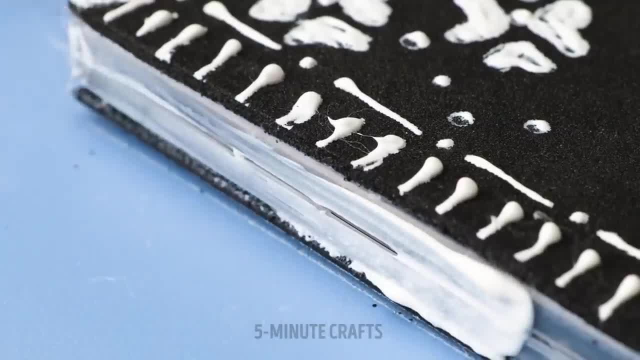 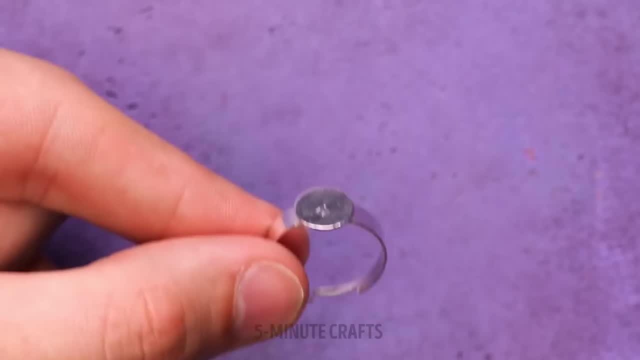 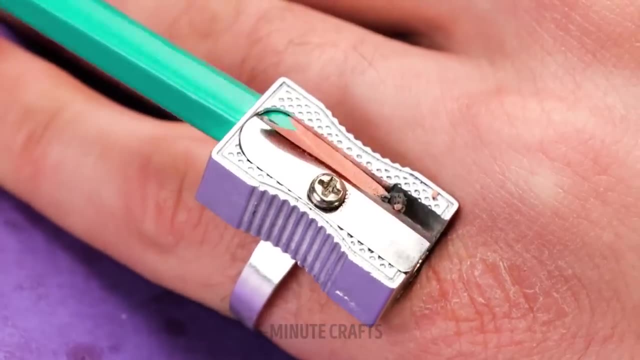 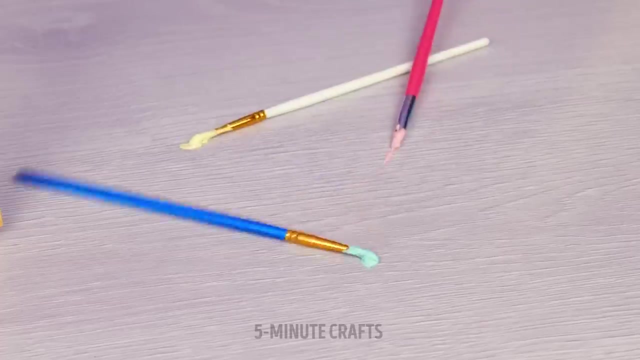 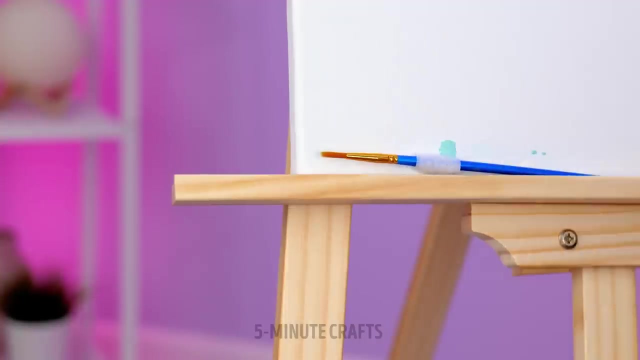 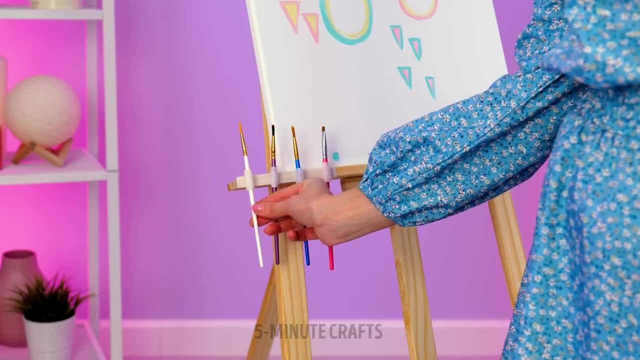 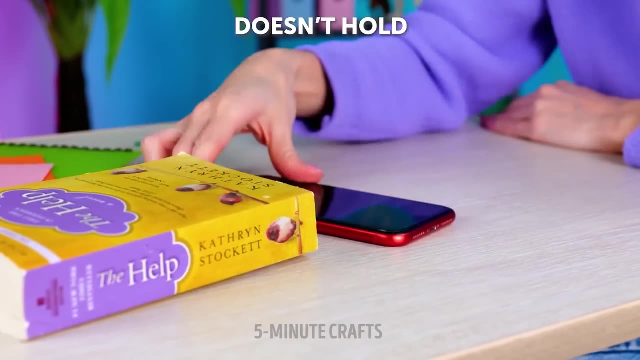 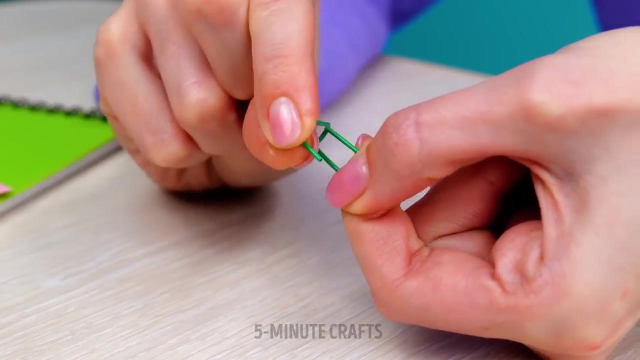 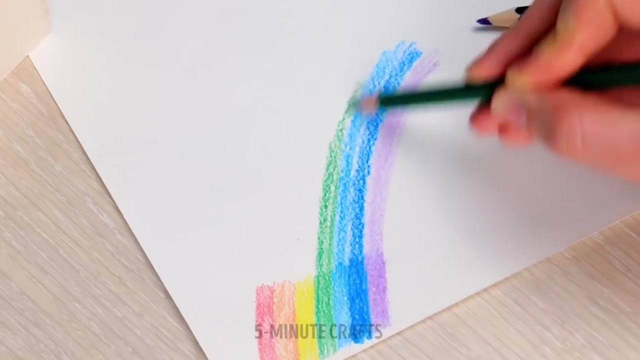 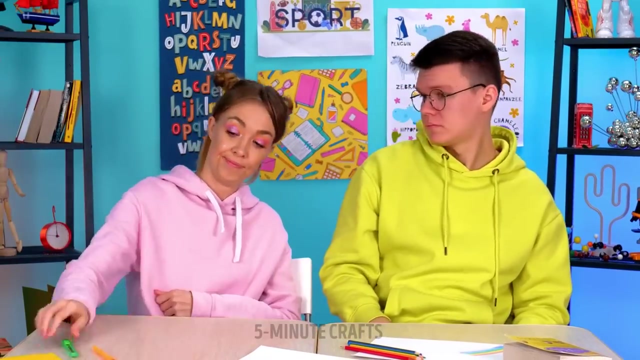 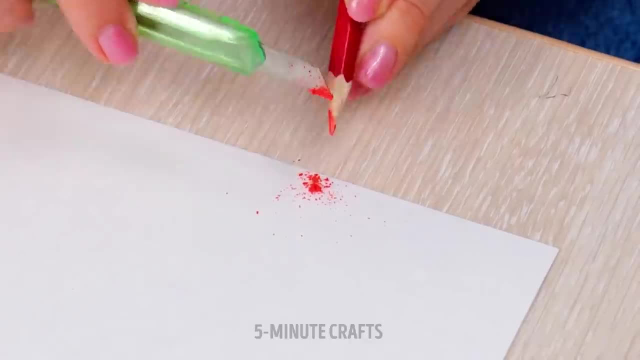 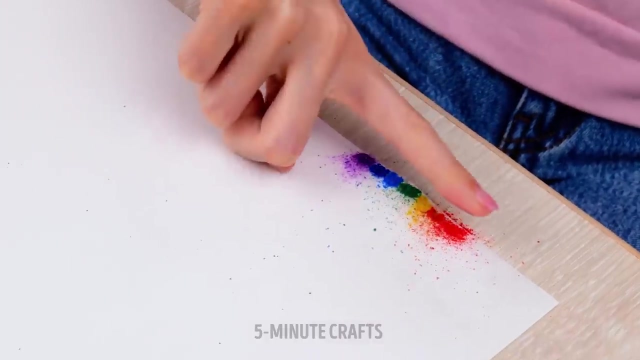 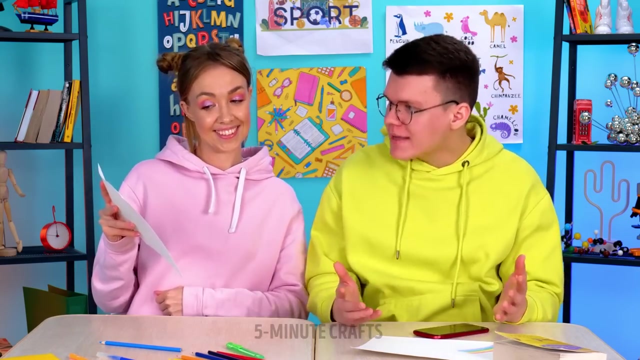 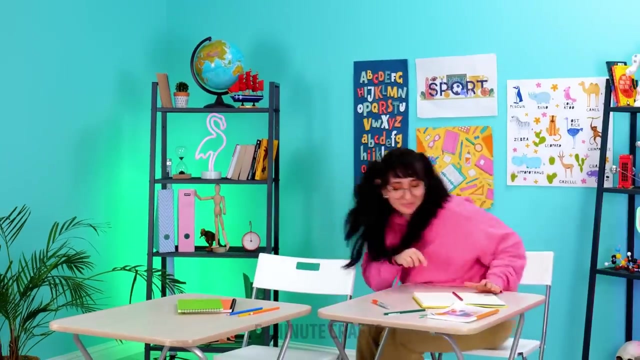 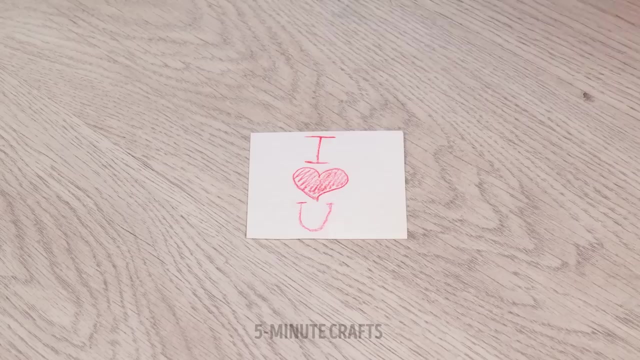 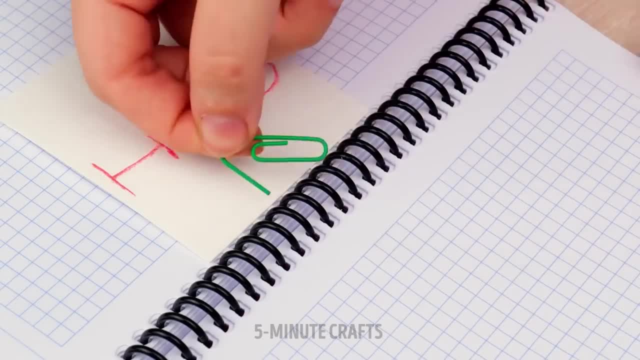 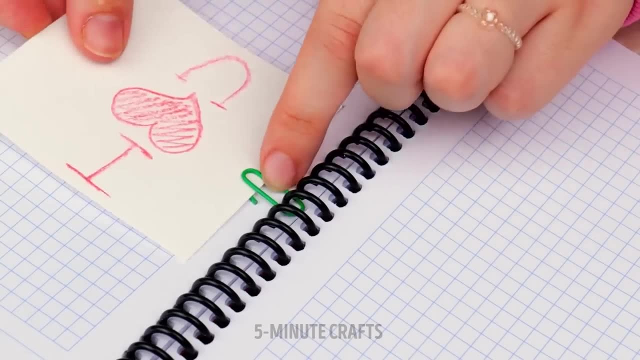 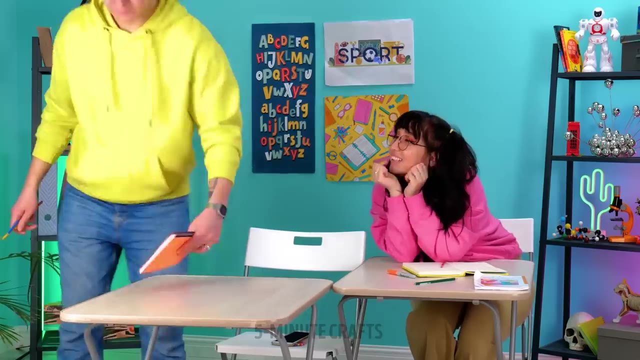 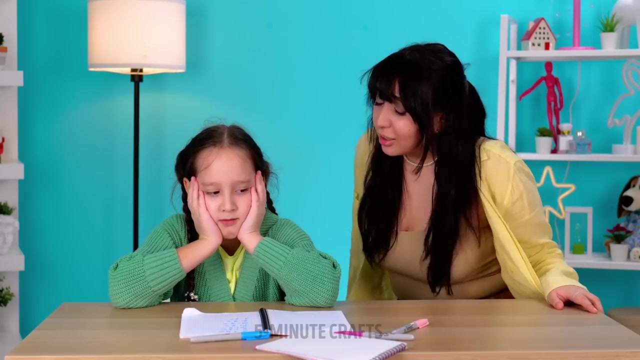 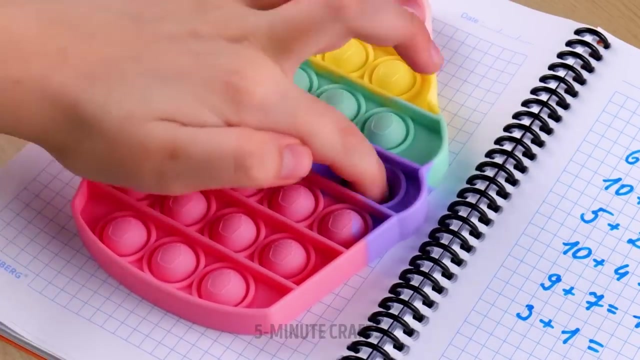 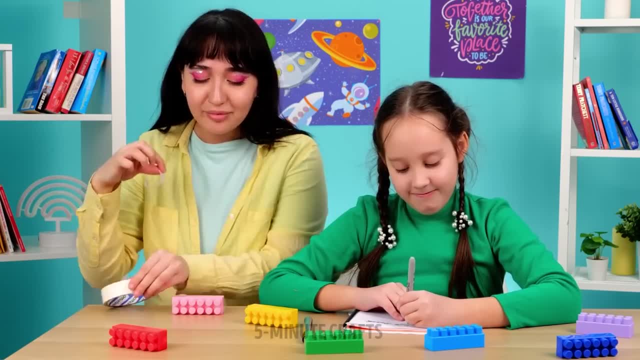 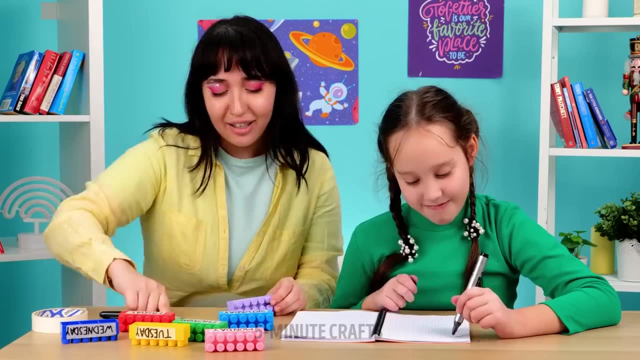 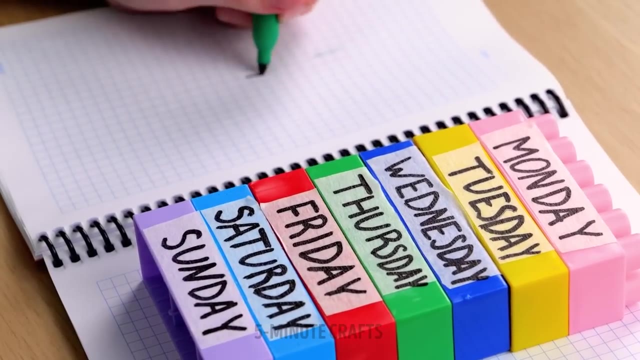 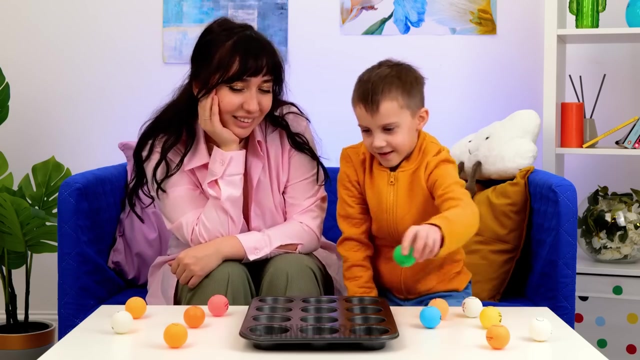 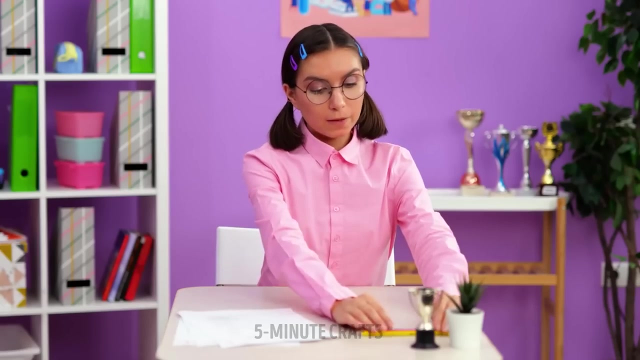 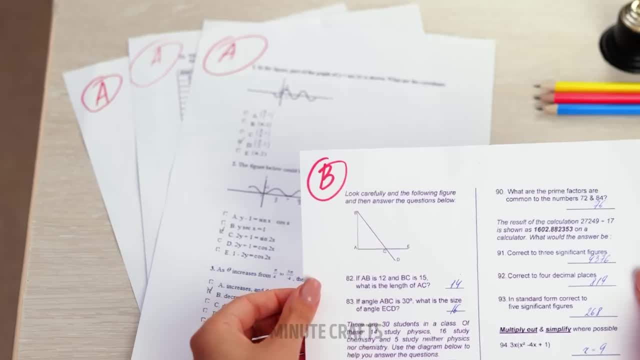 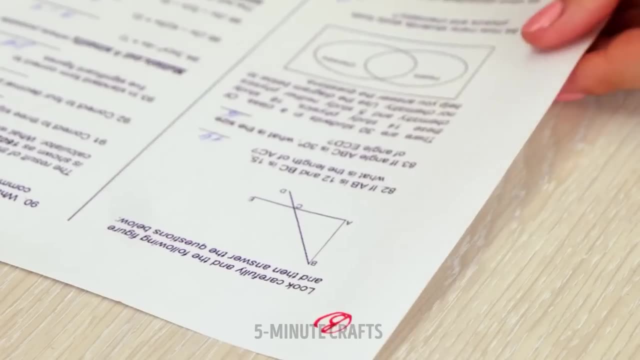 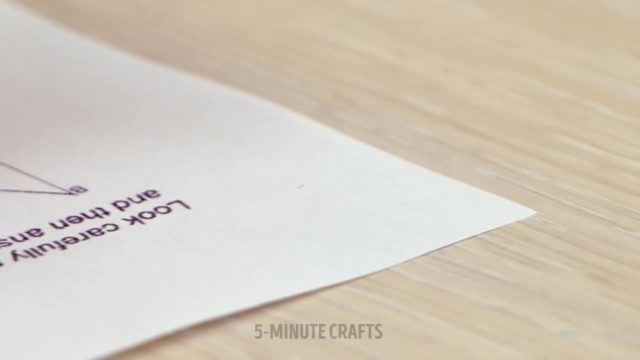 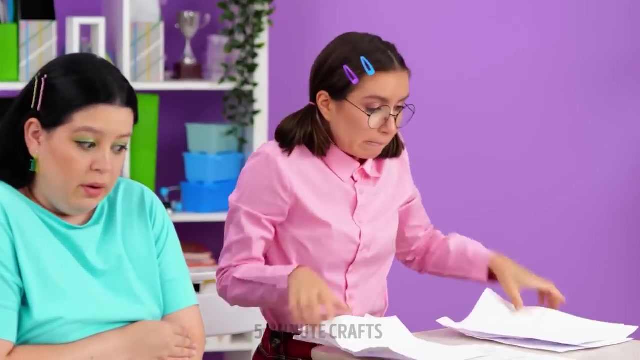 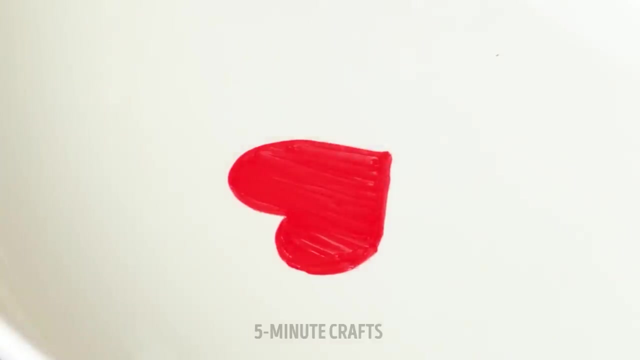 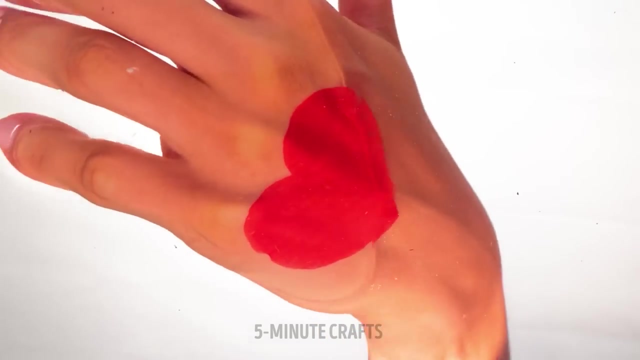 Be your light. Oh, oh, Be your light. Oh, oh, Be your light. Oh, oh, Be your light. Baby, I still wear the shirt you gave me, Cause it reminds me of the times When I was down and you were there to save me, Telling me that I'll be fine. 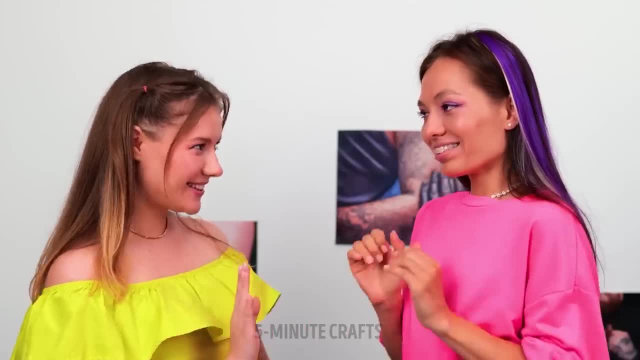 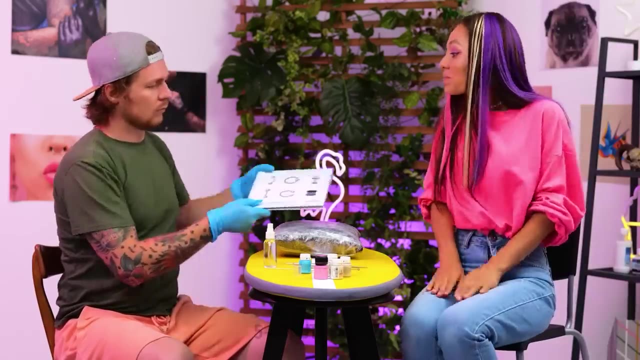 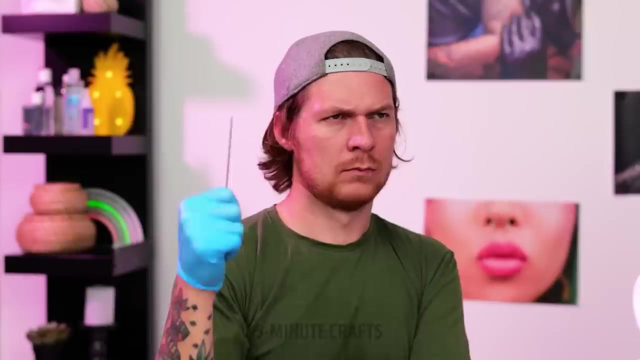 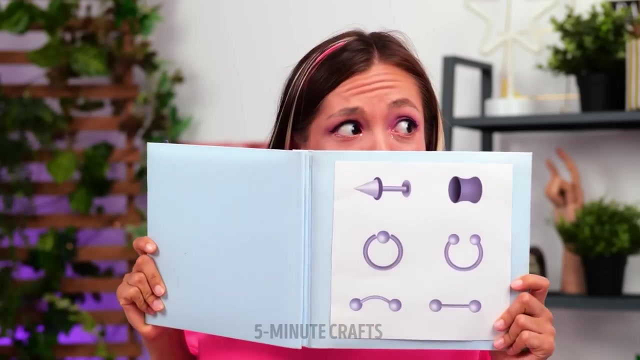 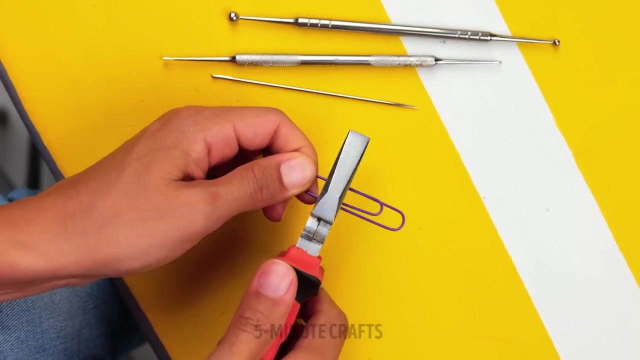 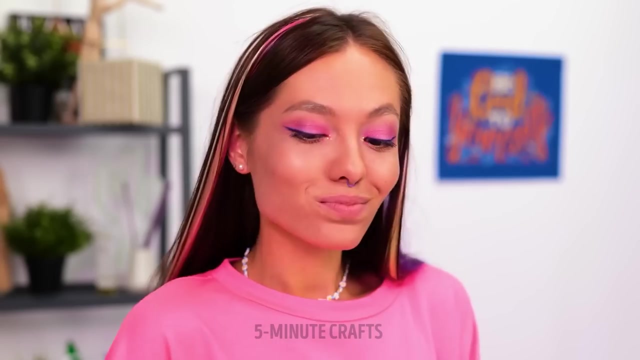 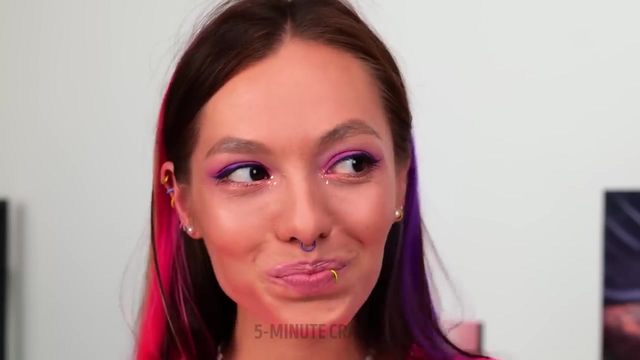 Put some music on, turn the lights down low, Throw the pillows off the bed, Blow the candles out. move your body slow. You got something on your mind. I'ma try to help you. let it go. Try to help you. let it go If you got something on your mind. 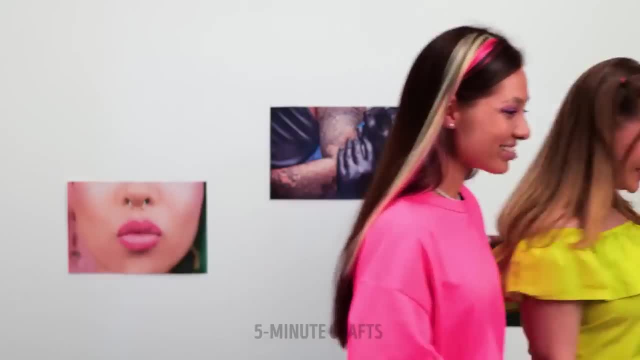 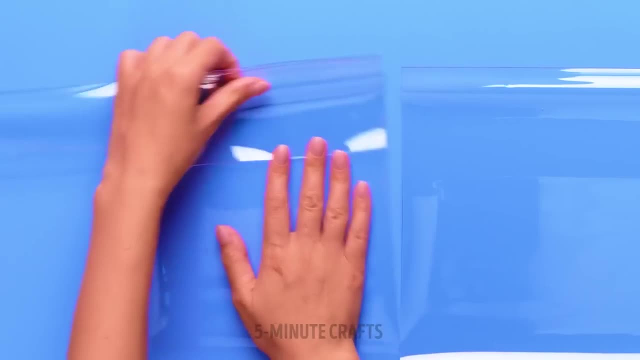 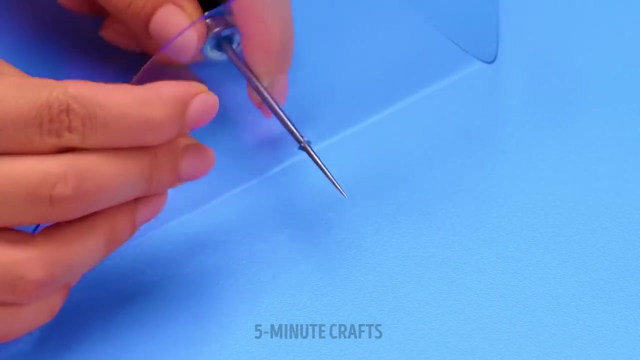 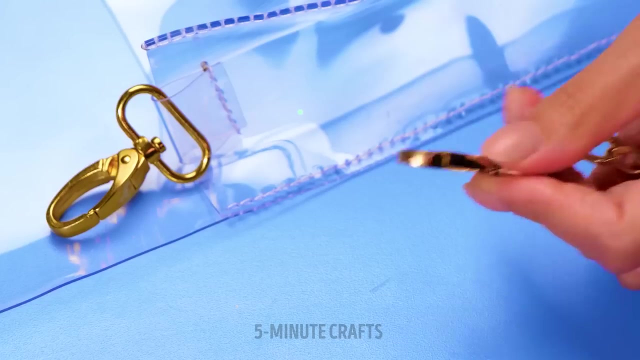 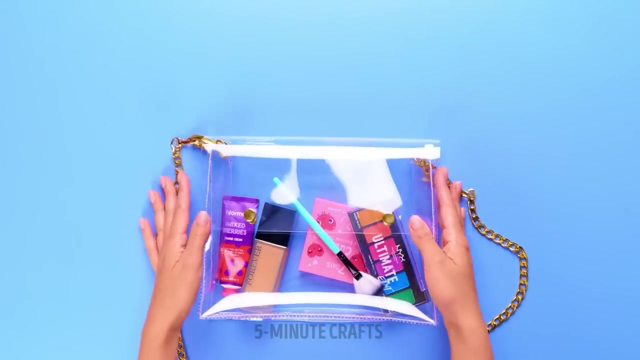 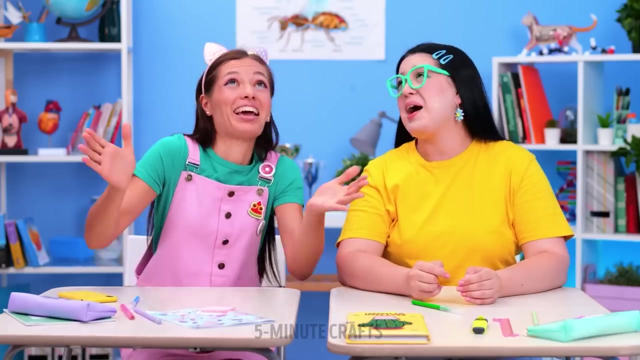 I'ma try to help you, let it go. You got, you got. you got something on your mind. I'ma try to help you. let it go. I'ma try to help you. let it go. Try to help you, let it go. I'ma try to help you. let it go. 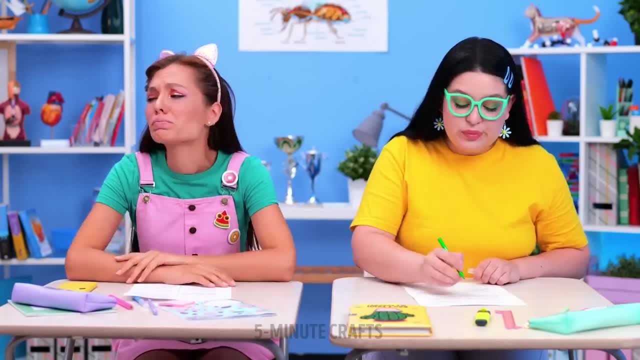 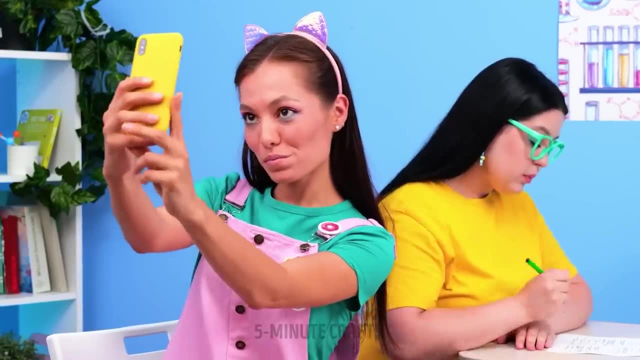 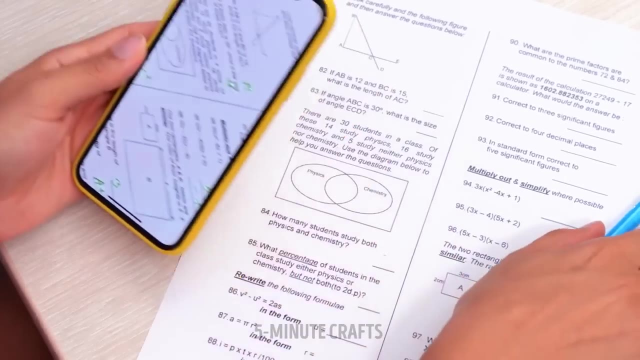 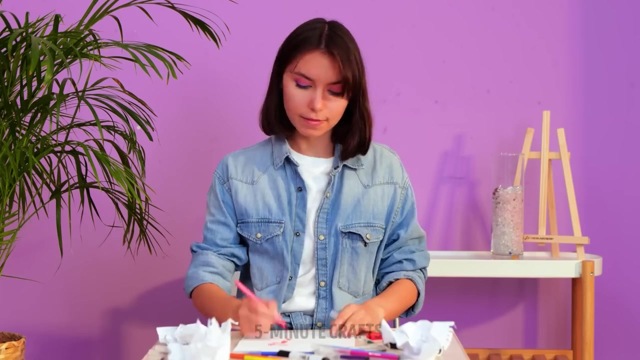 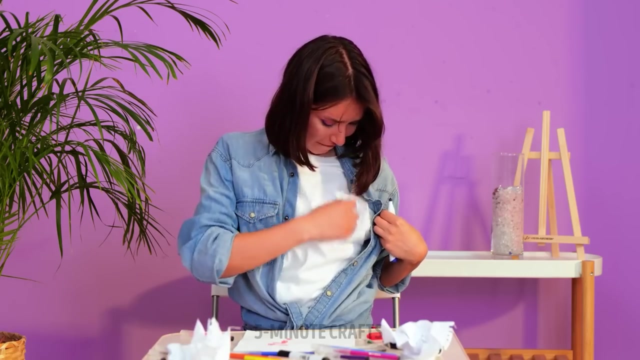 Try to help you. let it go. You know it's way too late. regretting our mistakes- See, that's so head over heels crazy. Need to apologize. we went too far this time. Come a little closer. there's something I have to say: I love you and I hate you, and I hope you feel the same. 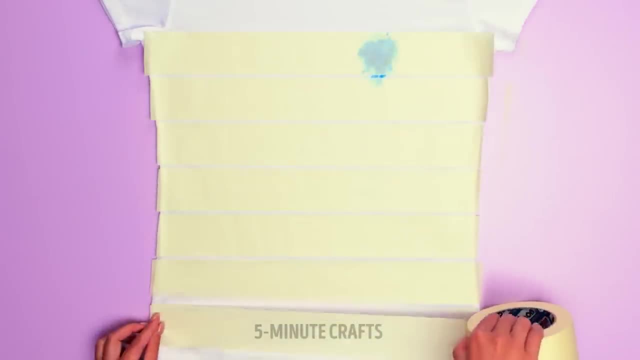 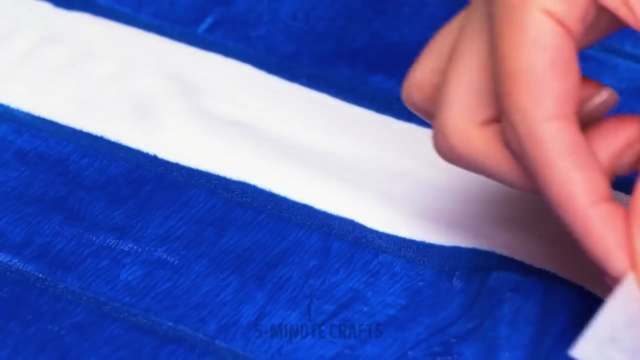 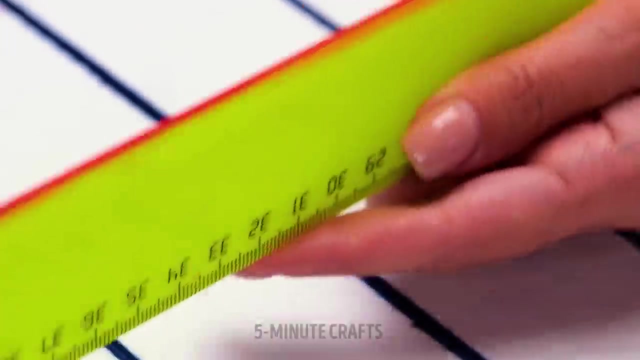 Come a little closer, baby. please don't walk away. I love you and I- yeah. You got nothing to prove, oh, baby, I know. You're done right by me, I'm done right by you. You got nothing to prove, oh baby, I know. 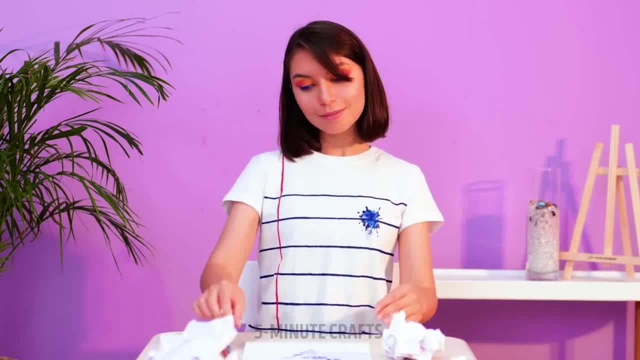 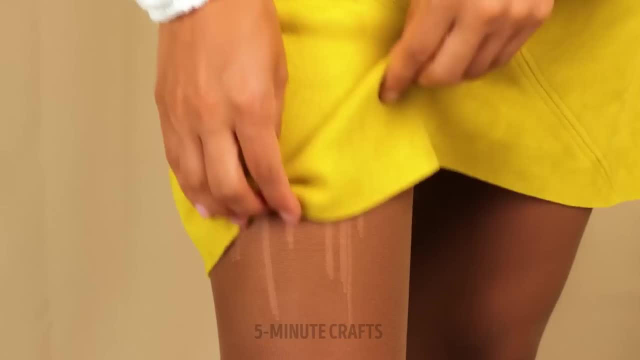 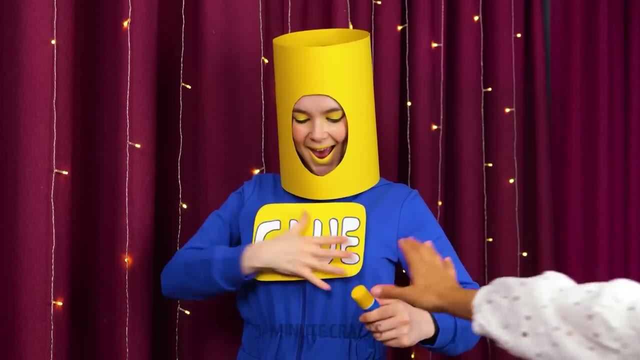 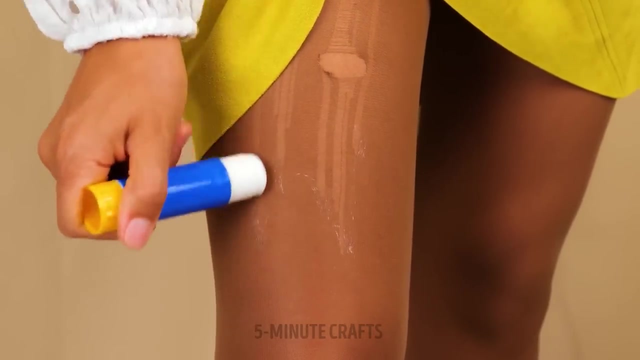 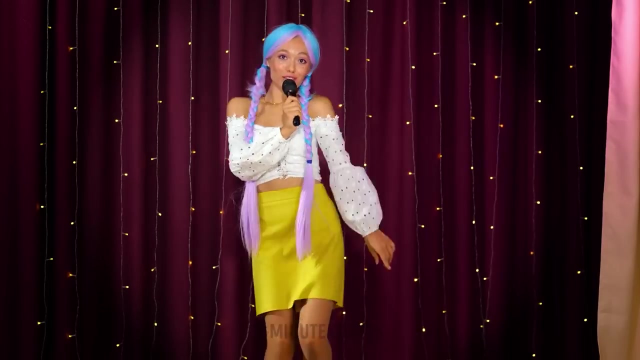 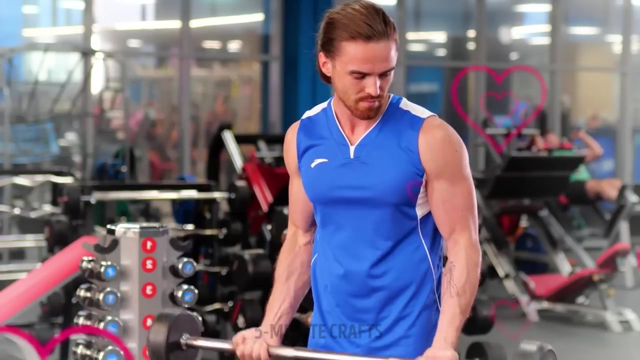 Oh, We got this. It's way too easy to say stuff I never do. You know, it's not how I feel, baby. So can we love each other. So can we love each other. Let this slide. can't stop to see you cry. Come a little closer. there's something I have to say. 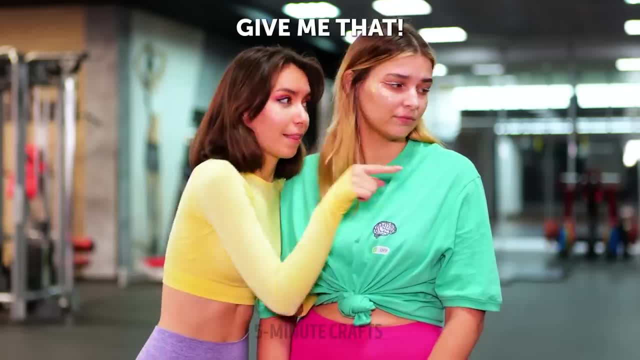 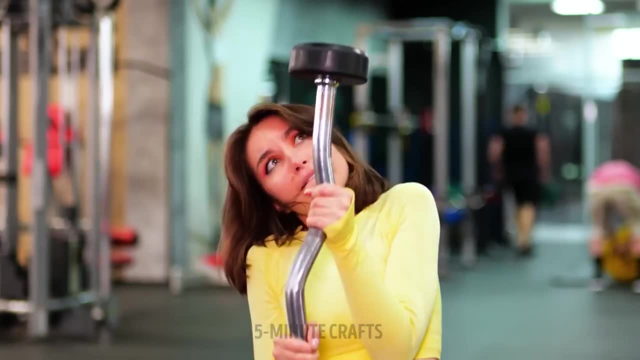 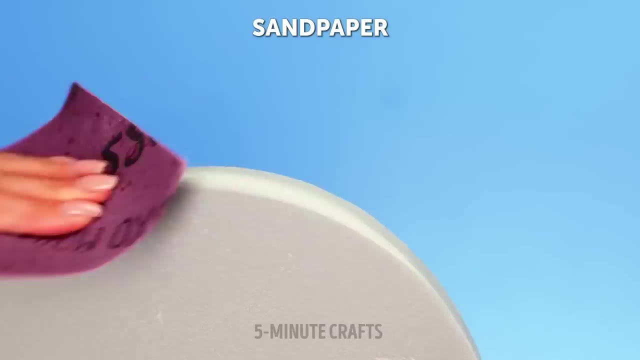 I love you and I hate you, and I hope you feel the same. Come a little closer, baby. please don't walk away. I love you and I- yeah, You got nothing to prove. oh, baby, I know You're done right by me, I'm done right by you. 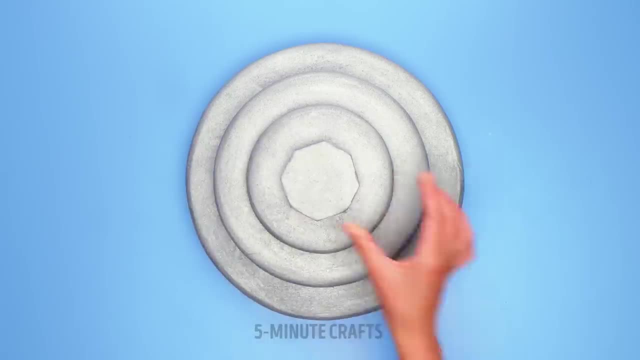 You got nothing to prove. oh baby, I know You're done right by me, I'm done right by you. You got nothing to prove, oh baby, I know You got nothing to prove. oh baby, I know You got nothing to prove. oh baby, I know. 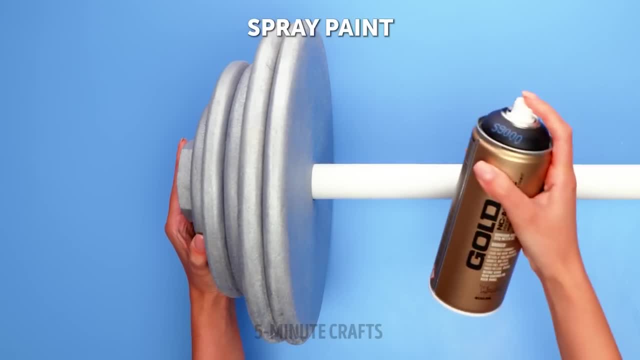 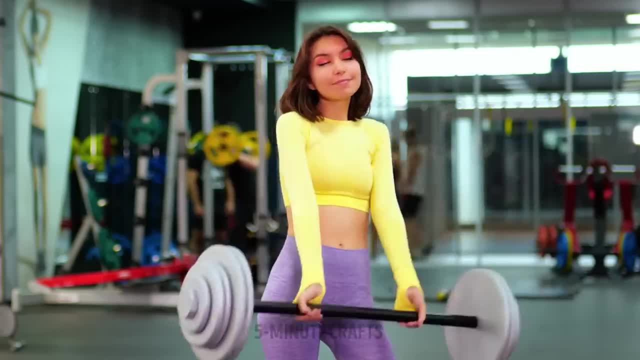 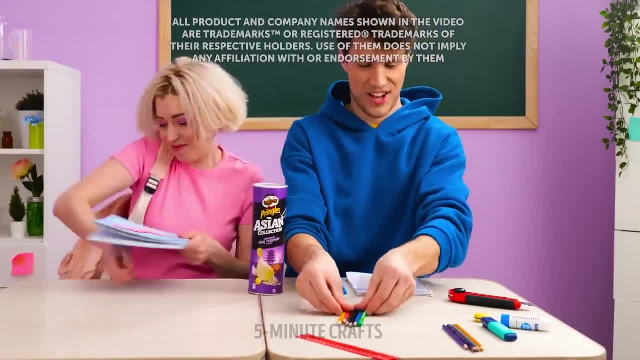 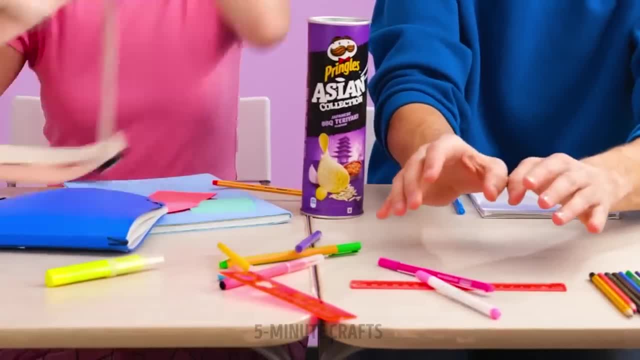 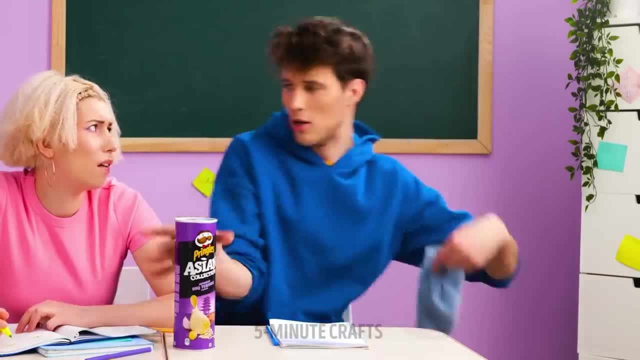 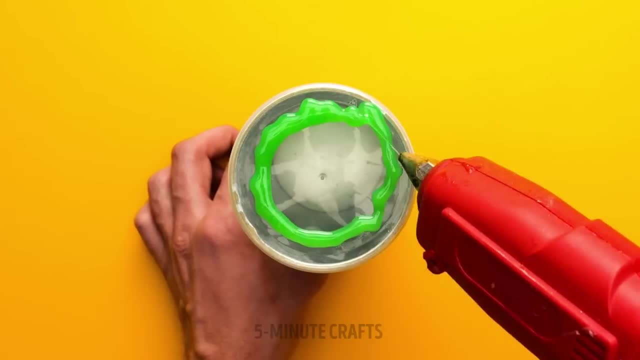 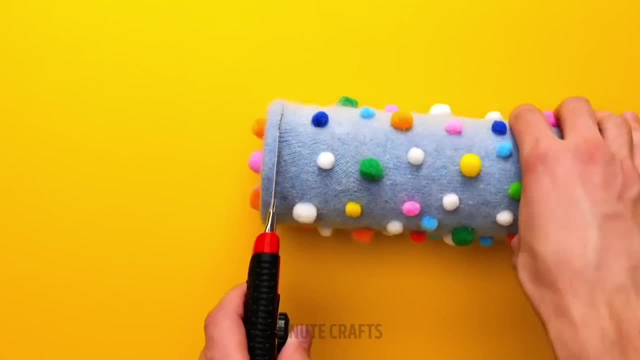 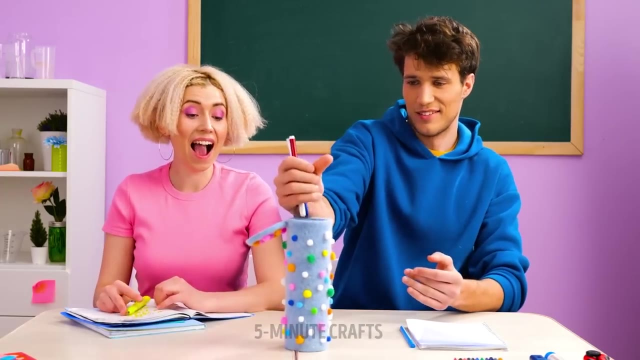 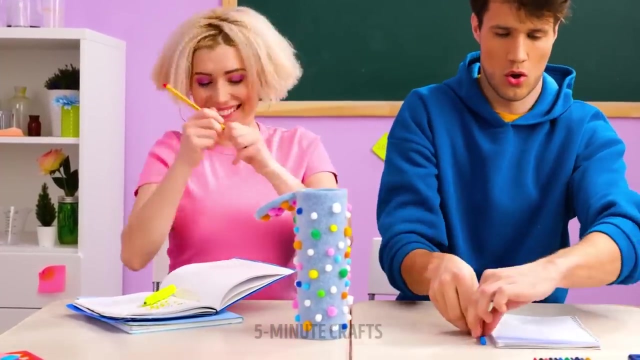 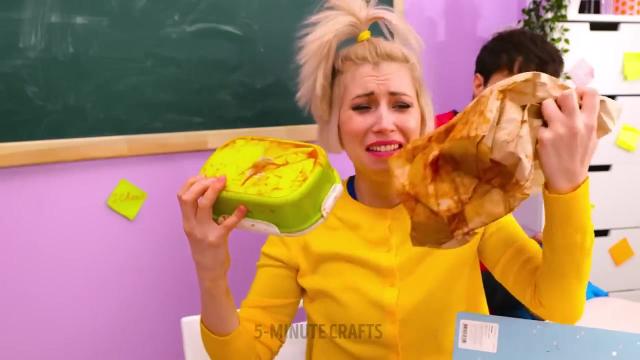 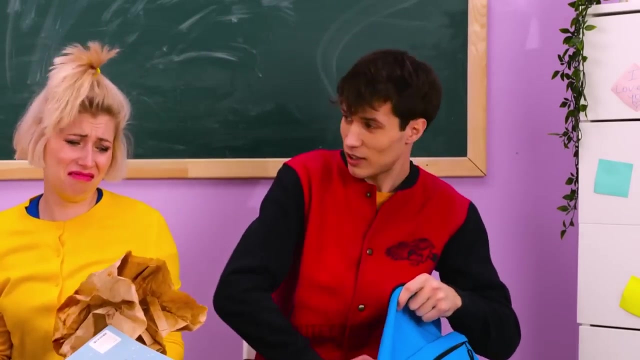 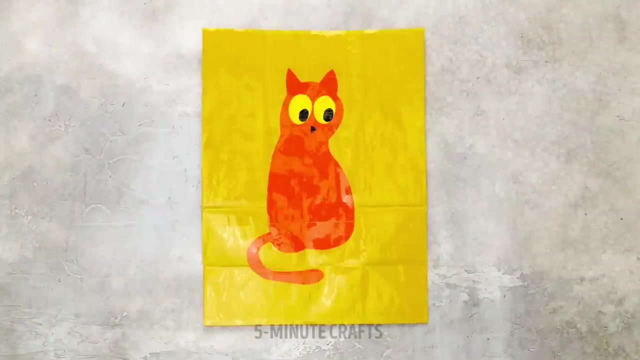 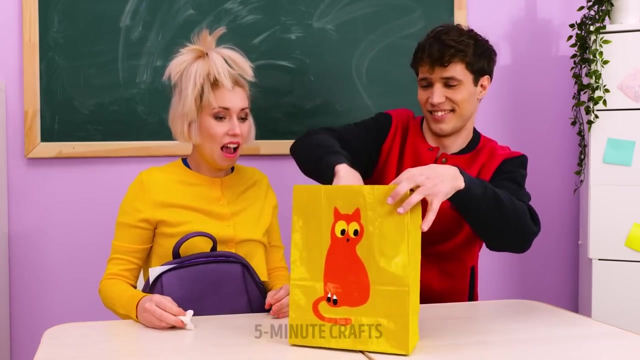 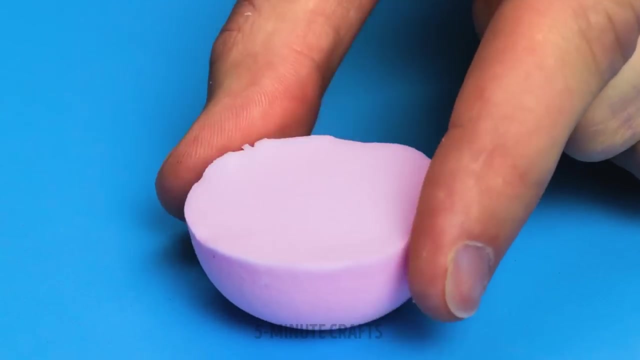 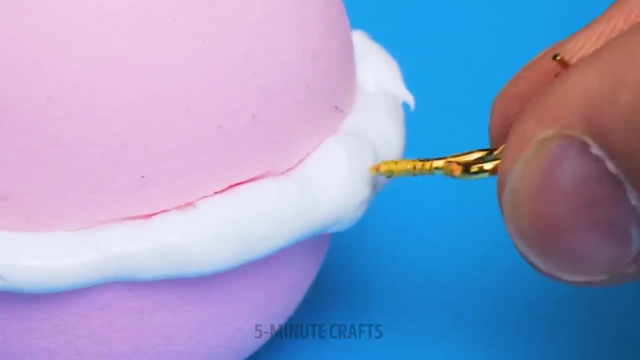 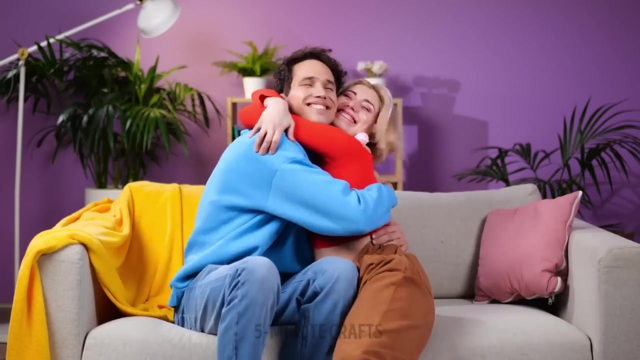 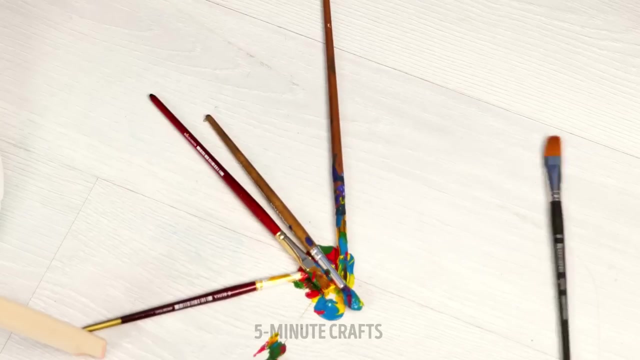 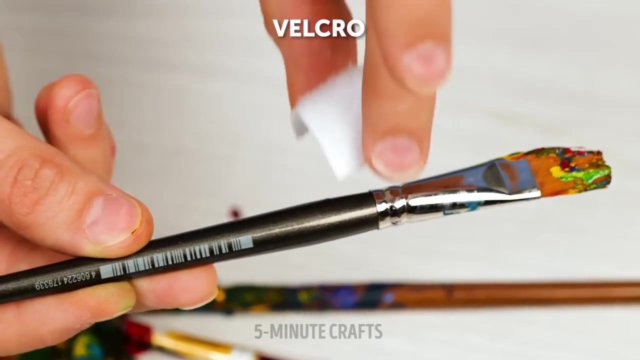